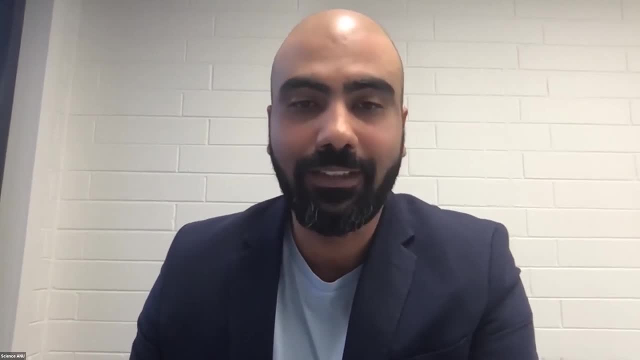 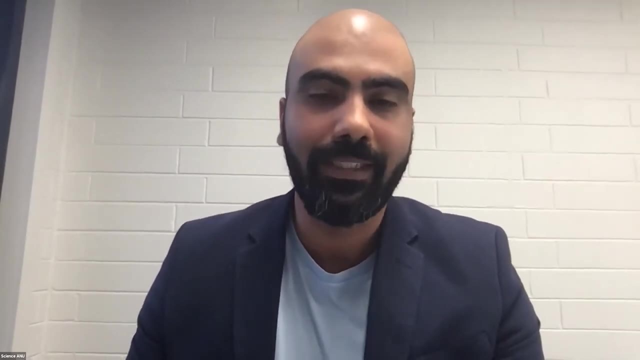 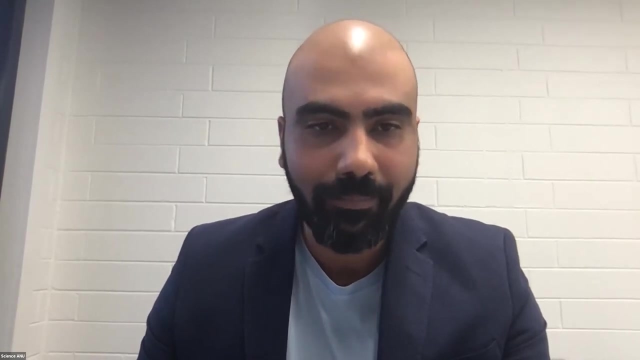 and his research interests centre on physical processes governing the ocean and climate. He's also a chief investigator of the Australian Research Council's Centre of Excellence for Climate Extremes, where he leads development of tools to understand the climate system at progressively finer scales. Andy has made many unique contributions towards our understanding. 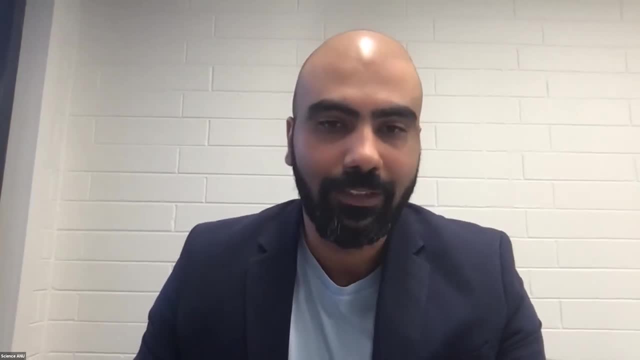 of the Southern Ocean and is the recipient of multiple prestigious awards, some of which include the Frederick White Prize from the Australian Academy of Science, the Nicholas P Fofanoff Award from the American Academy of Science. Andy is an executive director and research assistant for the Australian Institute of 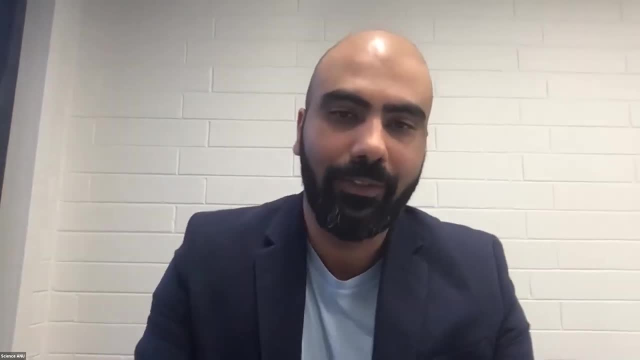 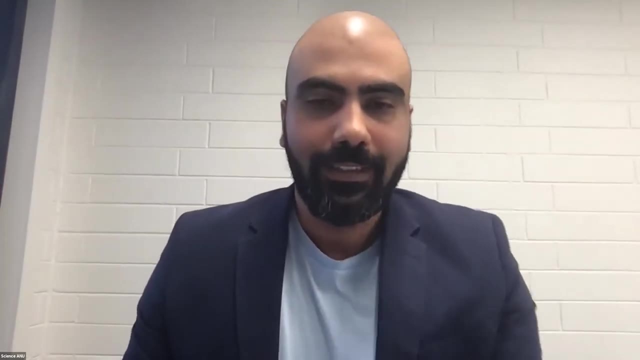 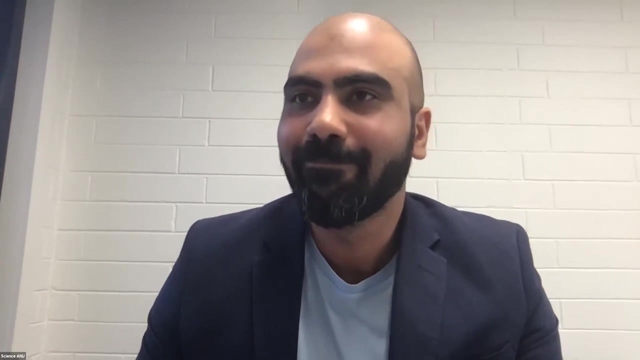 and meteorological society and the priestly medals from the australian meteorological and oceanographic society. so, without further ado, i'll now hand over to professor andy hogg to tell us more about modeling the global ocean circulation. over to you, andy, okay. thank you, jay. 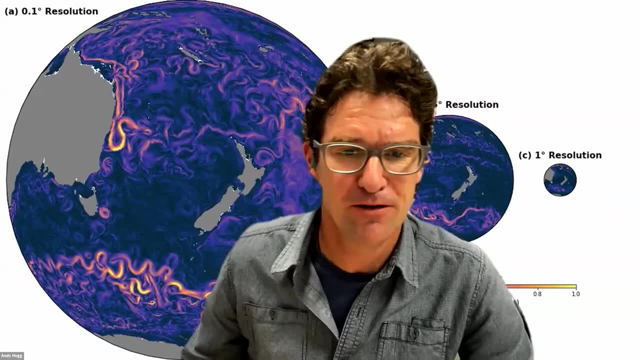 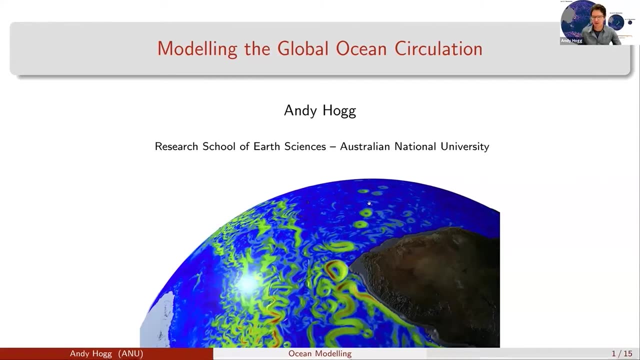 and thank you everyone for attending online. uh, i'm just going to start up my screen here and confirm with jay that. uh, well, i'll ask jay to tell me if there's a problem. hopefully, you can see the images on the screen there. so i'm going to talk. it's all good. okay, thank you, uh, today i'm 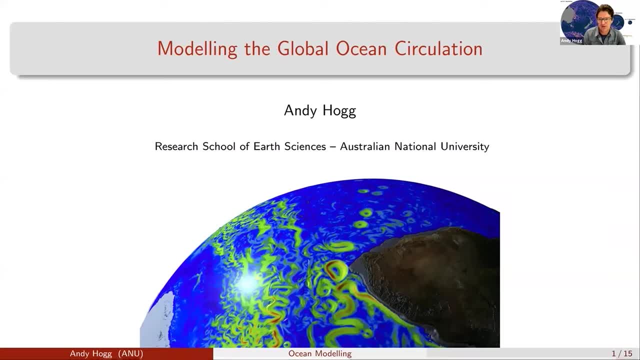 going to talk about the techniques we use to model the global ocean circulation, and i know there's going to be a range of backgrounds here. some of you are probably physicists or mathematicians, some of you might be earth scientists. what i'm going to, what i'd really like to do, is explain. 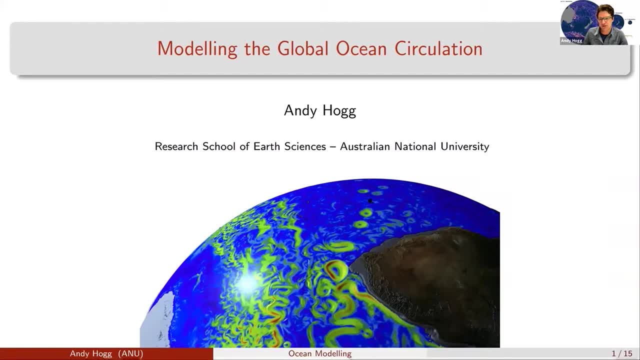 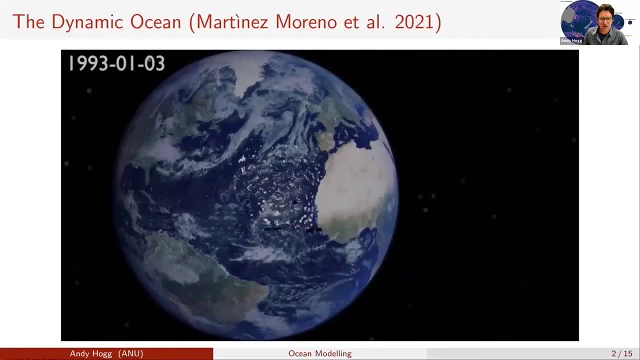 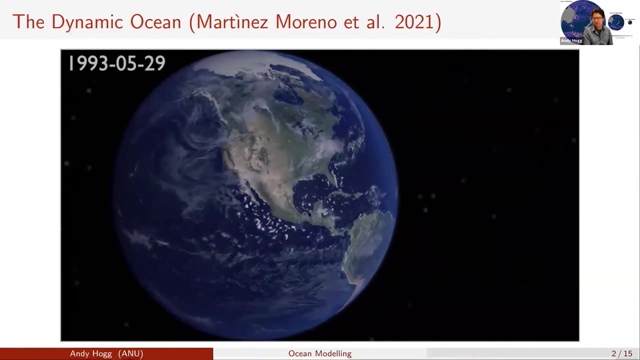 why and how we want to model the ocean circulation, some of the tools we use to do it and some of the applications of these models. so, to start with, i'm i'm going to tell you a little bit about the ocean, and this is a video one of my students made recently when he submitted a paper, and everything you're seeing. 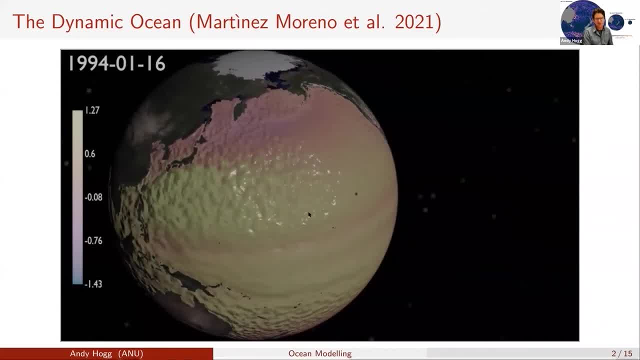 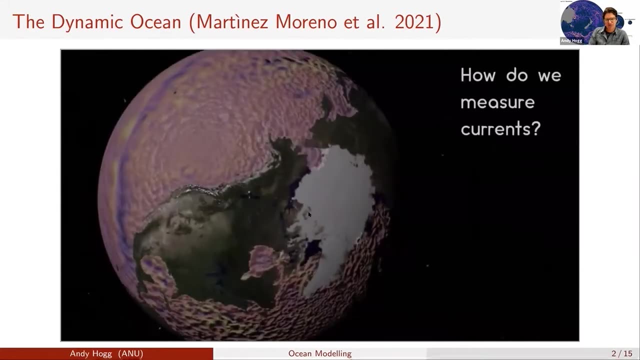 here. uh, well, actually those little satellites buzzing over there animated, but all the colors that you're seeing on the surface of the ocean, that's actually an exaggeration of the surface height of the ocean as recorded by satellites. so these, uh, satellite images give us really detailed. 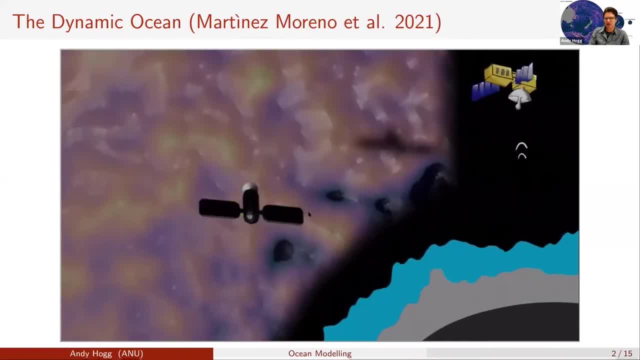 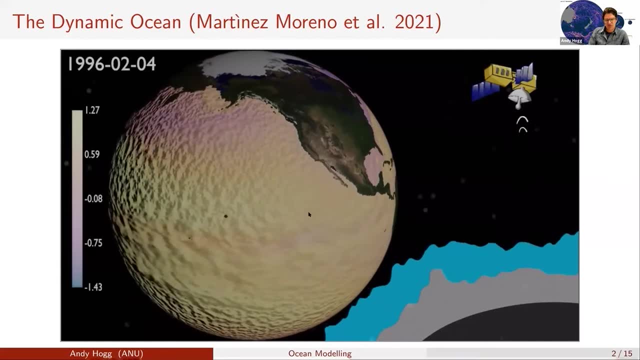 look at what the the sea surface height is doing, and this little graphic here is just to explain how these altimeters measure the height of the ocean. when you look at these sorts of images, you see that the ocean is actually a very dynamic thing. there's lots and lots of uh circulation features. 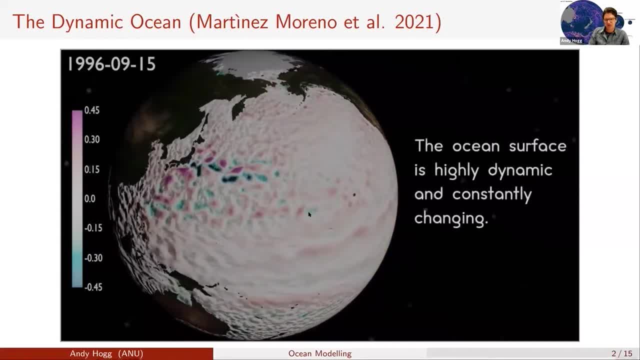 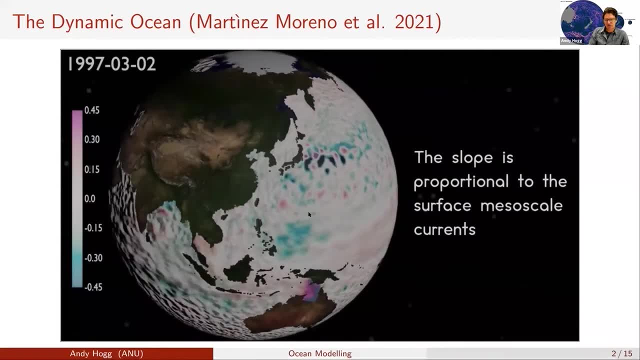 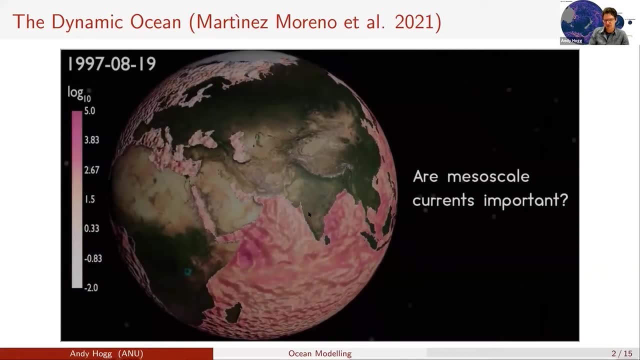 that are going on at small scales. some parts of the ocean are highly energetic. uh, some of them are not particularly energetic. you can see that, uh, it looks very different when you get close to the equator, and all these things are explainable in terms of uh, in terms of the uh, the fundamental. 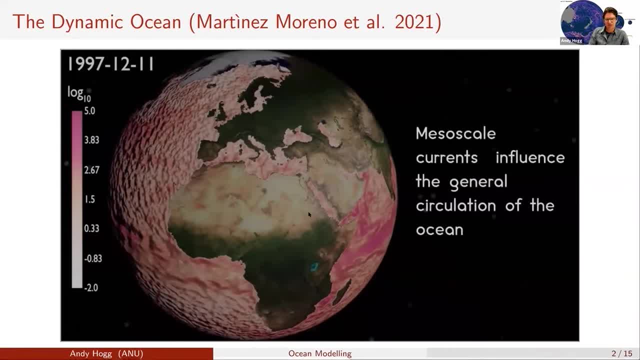 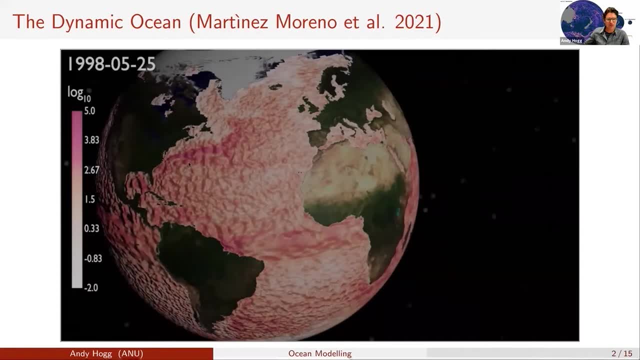 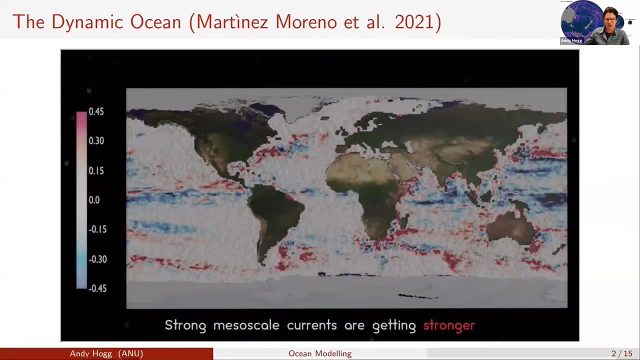 physics of how fluid mechanics on the ocean circulation works. so, uh, just to pick out a few of the key features here you can see things. hopefully you can see my mouse. here you can see things like the gulf stream coming up the west coast of the eastern coast of the us and the egalis current. that you can see. 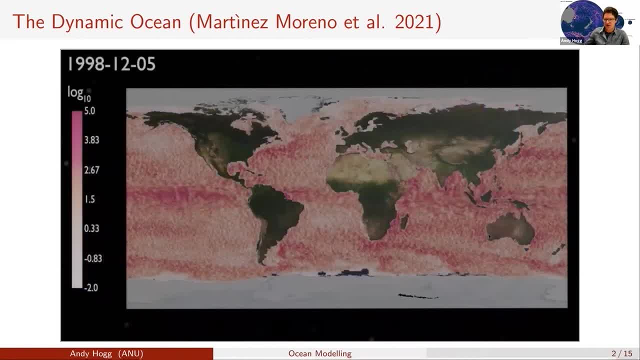 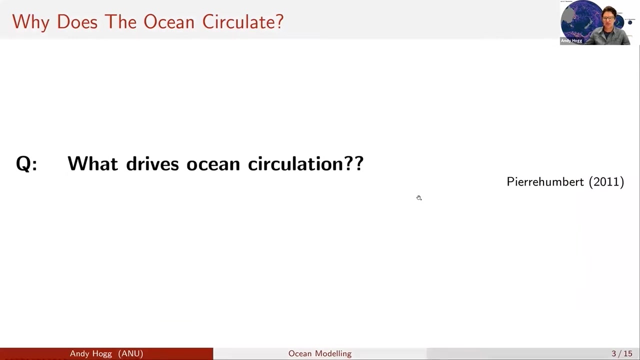 off the tip of south africa here and you can also see at the equator a few features propagating westward, causing lots of big eddies and things like that. so i'm going to stop this simulation here and if i can get the right uh button, that's right, and i'm going to ask you all a fundamental 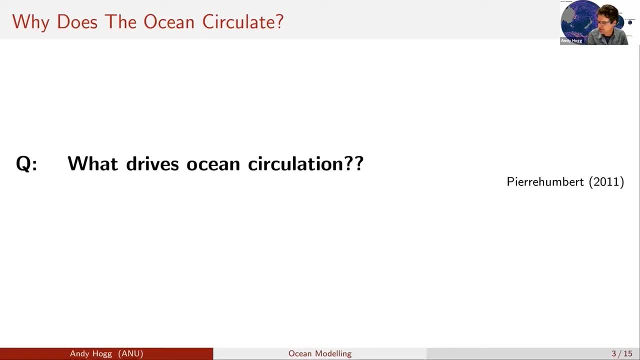 question and jay's going to actually release a poll. i understand we can see how that that works. i i would like you all to give this a little bit of thought and answer me. the question is: why does the ocean circulate? what? what is it that is driving, uh, the ocean to actually move in the first place? 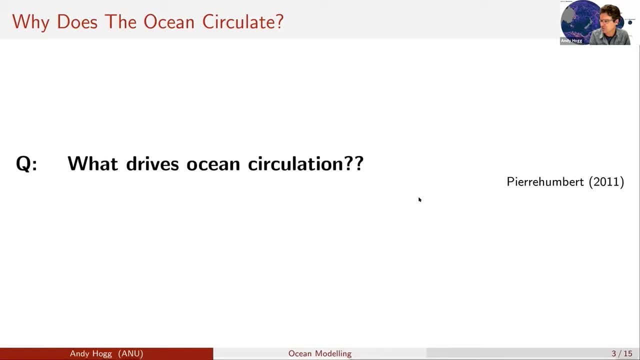 if we know what makes the ocean move, then we've got some ability to understand, uh, how things are gonna um, how things are gonna change and how we can model it. and, jay, maybe you're um compiling these uh poll answers and you're going to be able to give them to me at some stage, but um, 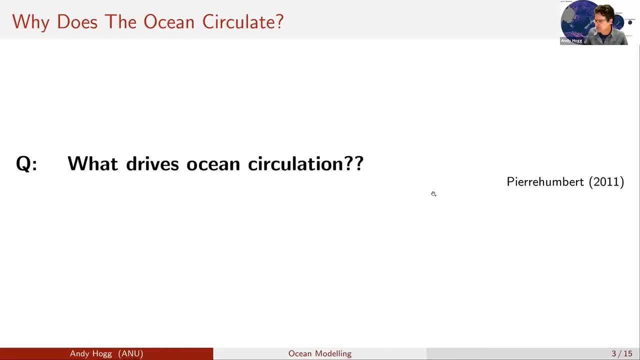 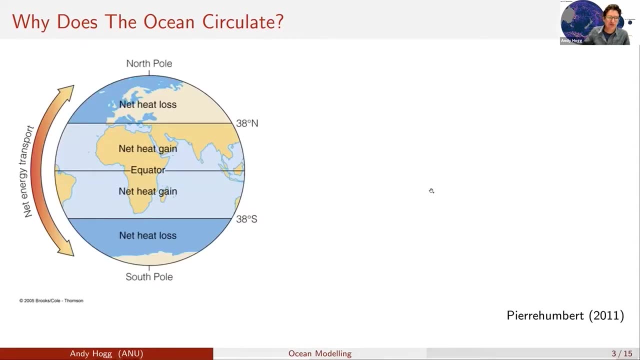 yeah, while you're answering that, i am going to just press on a little bit and we'll look at your results in a couple of slides. so, fundamentally, the reason we have a climate system at all is really because in the equatorial regions we get more sunlight than we lose in in. 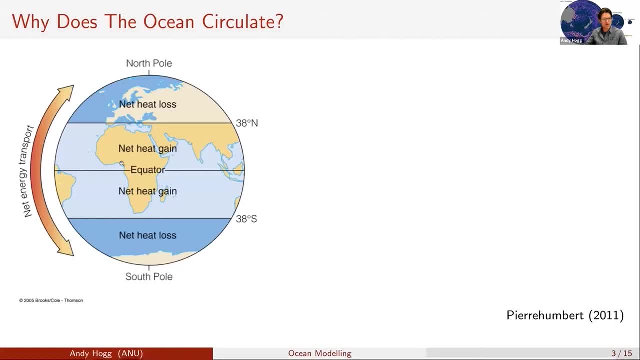 radiant energy through the top of the atmosphere. so we're always heating the equatorial regions more than we're cooling it by release of energy back to space. on the other hand, in the polar regions, uh, we're always heating, uh, the equatorial regions more than we're cooling it by release of energy back to space. on the other hand, in the polar regions. 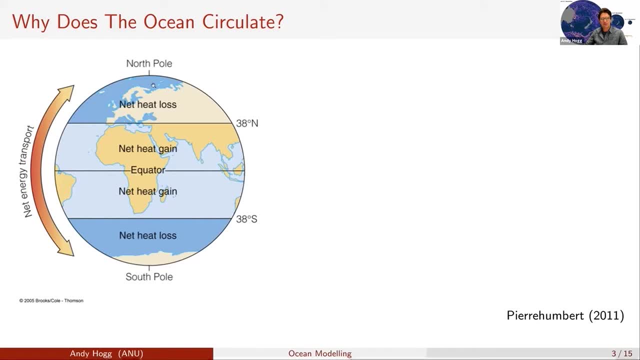 uh, we're actually cooling to space more than we're receiving from sunlight, and this is going on all the time. of course, these lines uh oscillate a little around a little bit as we go between uh seasons, um, but in general, north of about 38 north we we've got a net heat. 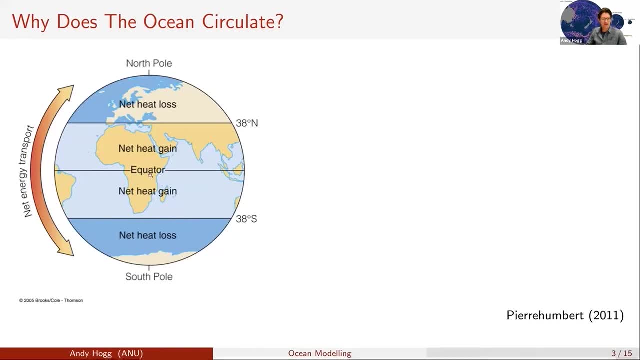 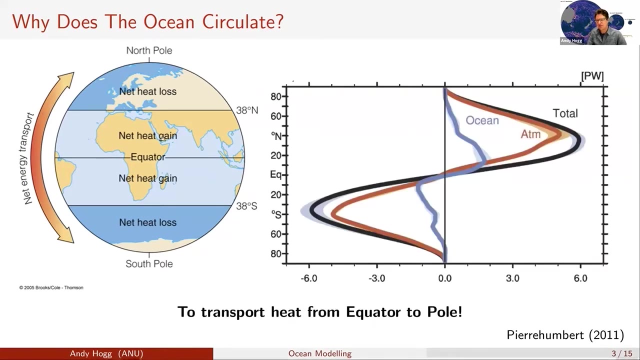 loss and in this equatorial region we have a net heat gain and what that means is really to conserve heat, then we must have some sort of system of transporting heat from the equatorial regions to the poles. this is what we call the polewood heat transport and this graph on the 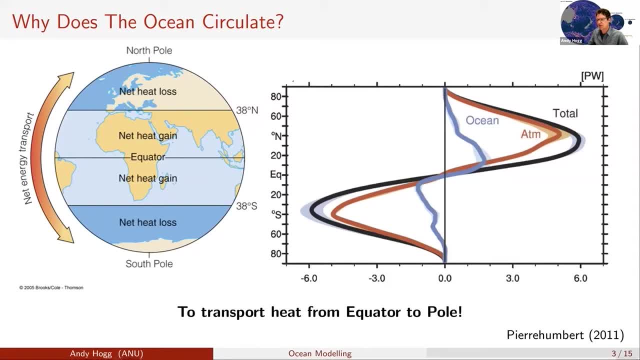 right is showing an estimate of the polewood heat transport that occurs and the estimate is from this black line here, and that estimate can be broken up into the atmospheric component, which is what you're seeing in the red here, and the ocean component, which is what you're seeing in the blue. 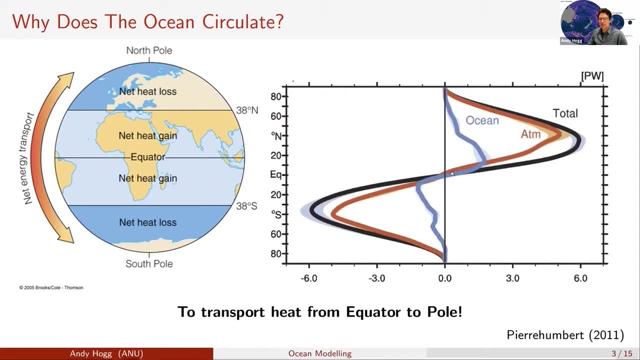 so what this is saying is: when, uh, heat transport is possible, it's pushing heat in a northward direction, and when heat transport is negative, it's pushing heat in a southward direction. and you can see that right at the equator we're just about at zero. so this is very much the ocean, and 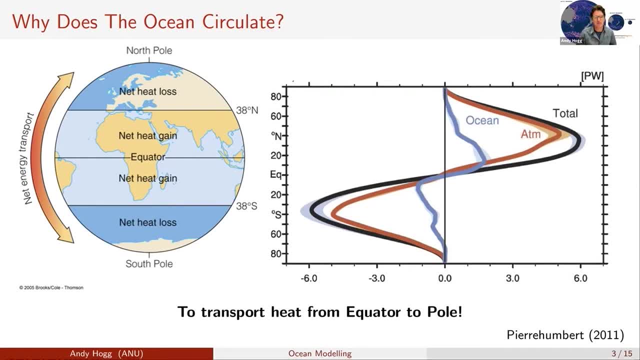 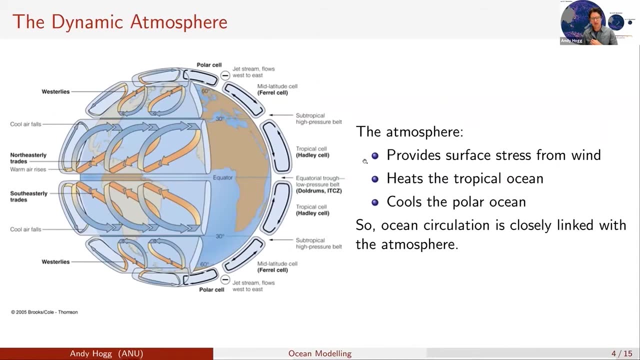 atmosphere system working to do its best to to shift heat from equator to pole. if it wasn't for that, we wouldn't have a climate system. how does that apply to the ocean? well, it implies it applies to the ocean because we've got a very dynamic atmosphere, and so the atmosphere does a few things. firstly, it the 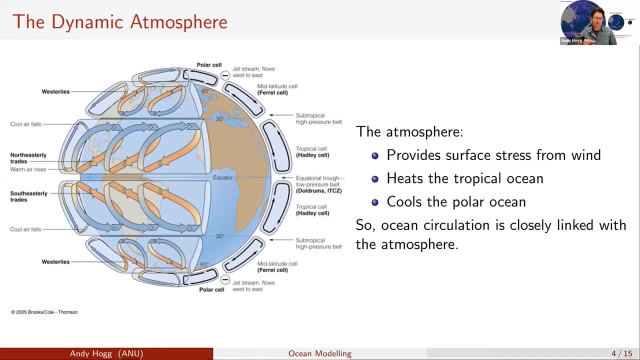 atmosphere has wind stresses which push on the surface surface of the ocean and move around the surface ocean waters, and the second thing it does is the atmosphere heats and cools, helps to heat and cool. the provide the boundary conditions that heat and cool the tropical and polar ocean. 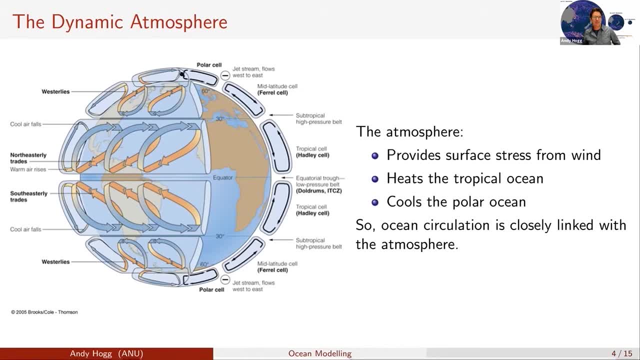 respectively. so at the tropics the ocean is heating and at the poles the ocean is cooling, and that is, of course, linked to the to the heat transport as well. so if, if Jay maybe has the answer to our poll, because I don't think I can see it, do you able to? okay, so the question was a little bit of a trick. 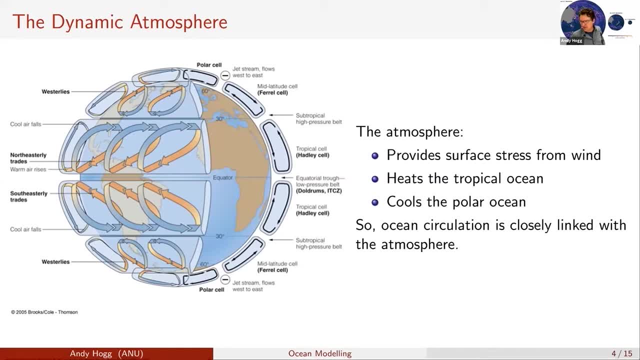 question, because the right answer is actually all of the above. certainly ice formation and melting actually does drive a flow in the ocean. certainly the winds push the ocean around, but fundamentally the temperature difference between equator and poles also also helped to drive circulation. so in the net 70% of you, I think, picked, although these percentages don't quite. 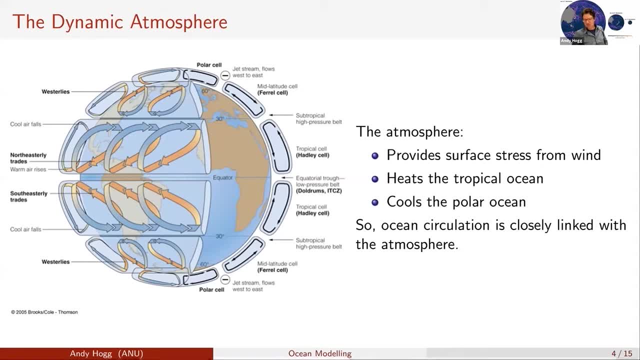 add up to me, Jay, but that's okay. the majority of you picked the right answer and hopefully you all thought about the answer for just a moment before you, before you gave your answer. I think some could pick more than one. that's why we add up to. 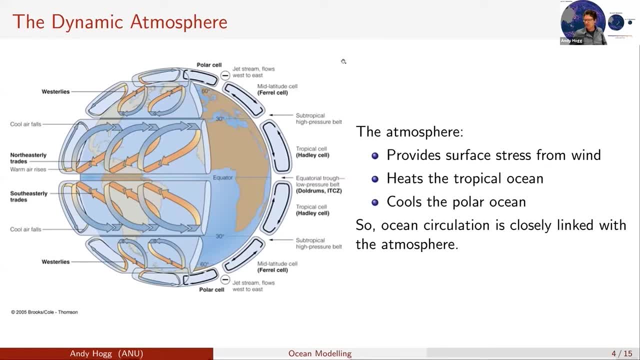 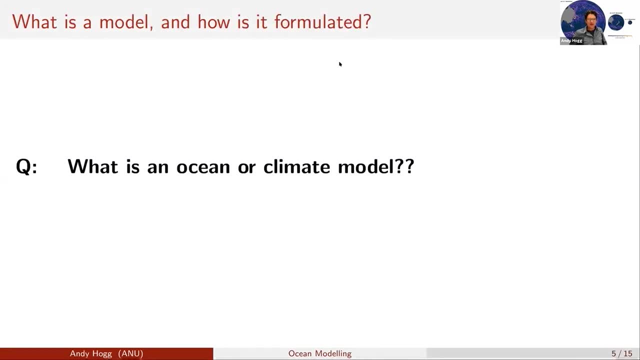 more than 100%. okay, in fact, maybe, maybe you gave one answer and then you reconsidered and gave a second, which is just fine, okay, so we've talked about the fundamentals of what drives our climate system. so the next question poll question Jay has for you, and then I'll let you go on to the next question. 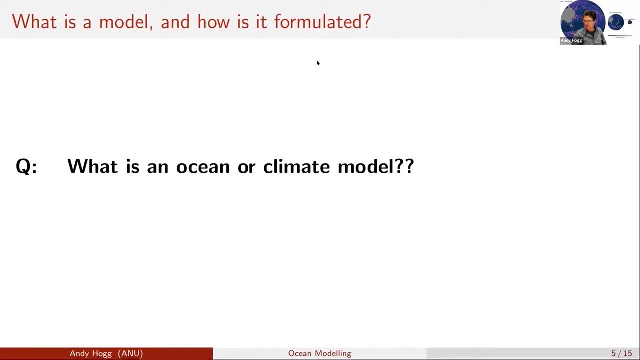 though, Jay, I will answer it. and you uh said it's the same question, so we'll get started. uh, okay, thank you, okay, so, um, so, I'm going to send it back to you. and again, this isn't I'm not out to trick you here- what, what I really want to do. 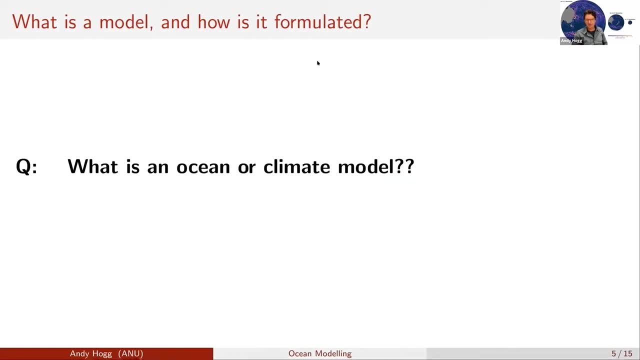 is is to ask you: what is a model? and I'm not going to leave this one open for very long so, and and I guess I'd make the point, some of you, you may be familiar things like that. so, of course, a model, the word model can mean different things to different 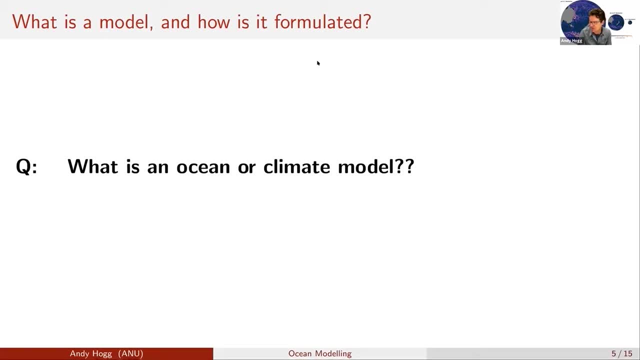 fields, but I'm interested to see what you all think. what of an ocean model? so hopefully you've all got some sort of response in- and Jay can maybe show me the answers to this one already- and there's a lot of support for empirical fits to observations and projection of trends. 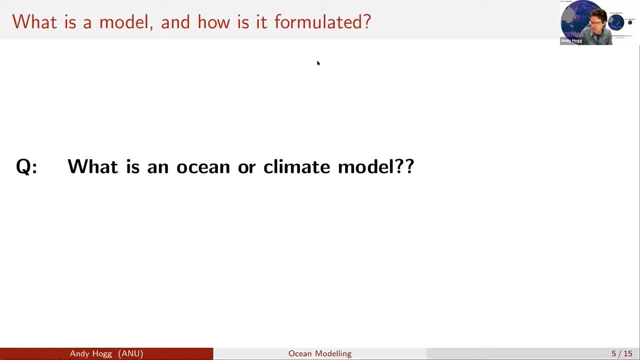 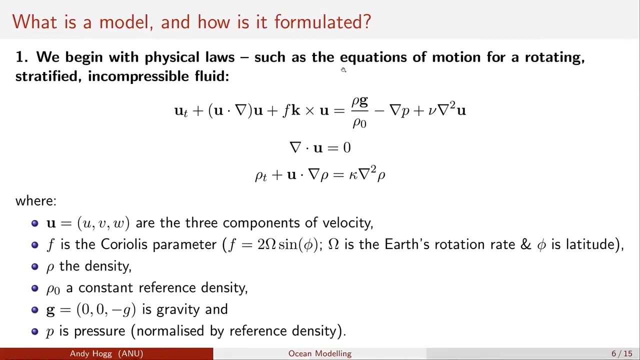 there's a little bit of support for small but exact copy, and there's also a little bit of support for a set of partial differential equations that are solved computationally. so the winner is actually that a model, you is a set of equations that we use to integrate forward, and so this differs from other fields. 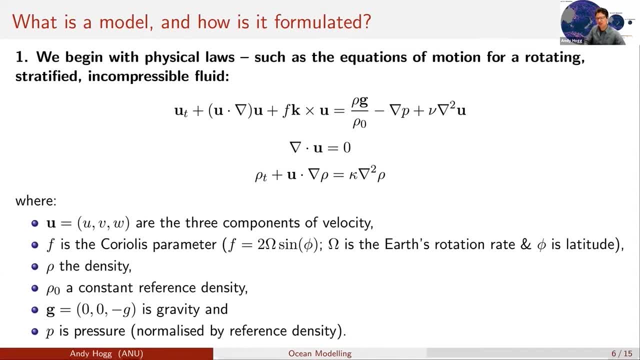 it differs from example, from economics and economic modeling, because in economic modeling you never have a set of physical laws that you can fall back on. what we have for an ocean model is a set of physical laws that we know. if we could actually solve the set of equations that I'm 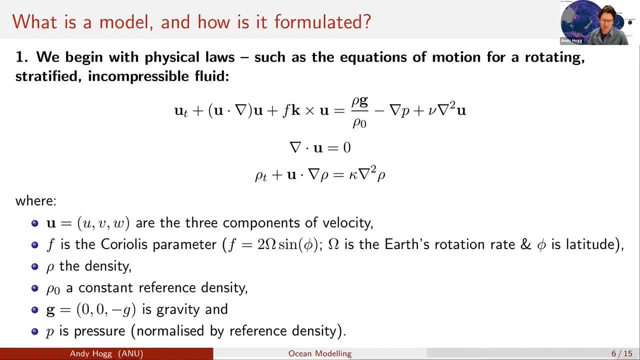 writing on the board in front of you. here we could actually model a set of equations that we could actually solve. the set of equations that I'm writing on the board, basically all the sets of equations- are just like a set of zooms: 일�ham, but not Cerda. 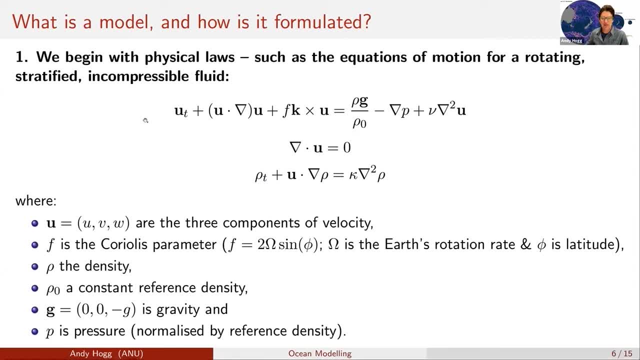 掩 � PuntaCty so these are all things that you can replicate in order to isolate them as you go through the the whole earth system almost exactly so for those of you who are not mathematicians don't be scared by this set of equations I don't expect you to assimilate everything that's on here but I do just want to explain just quickly how the how these equations are related to physical laws that you might understand. so this top equation here- well, actually this top equation here is a vector equation. so, yeah, it develops and we use vector equations more often than most others would like to do. it sausages into the scheme here, rather than policies or some rules. 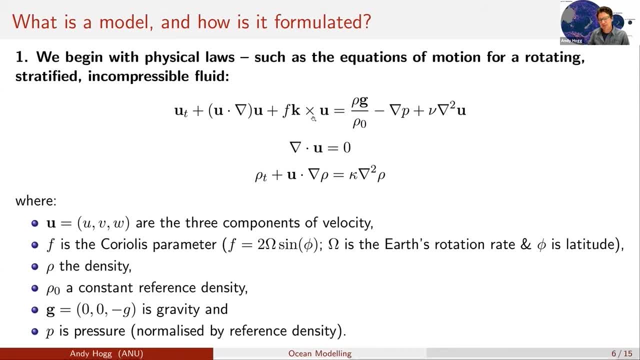 run them more quickly. if you don't find them, we'll talk about them during the training in this post and finish wouldn't think of them from the traditional platform or even further on. so I think sometimes teachers would probably try this top equation. here is a vector equation, so it's actually three equations and those of you. 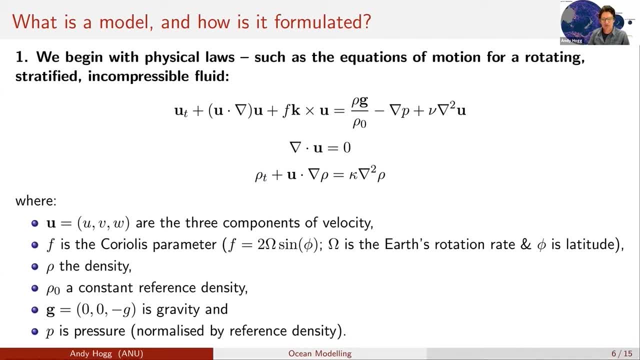 who are doing engineering or heat transfer may recognize this as the navier-stokes equation, and this equation is basically a force balance equation. it tells us how fast the momentum of a fluid will change, and there's a few things coming into play here. there's a term at the end. 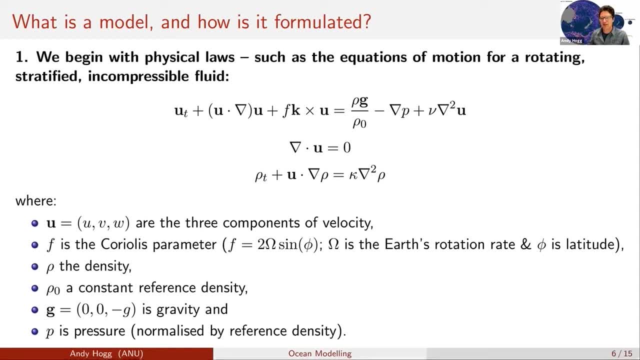 here, which is a viscosity which damps away- uh, things that are happening. there's a pressure gradient term here, which helps to drive a flow. uh, there's a gravitational term, because it turns out the, uh, the gravitational forces are important to the, to the ocean. uh, there's a coriolis term. 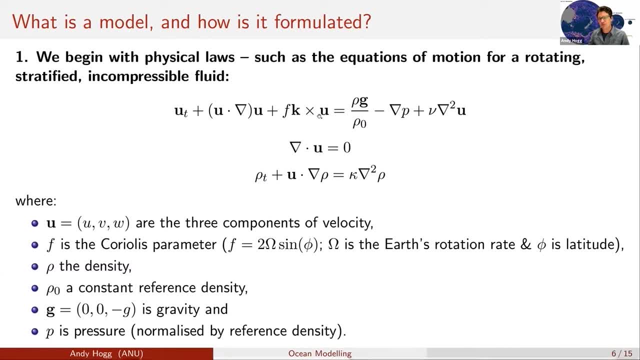 that you can see here. this is the effect of the rotating earth and it's why flows look different at the equator than they do at the poles. and we've got an advection term here. uh, this is the tricky term. this is the term that means that we actually find it very difficult to 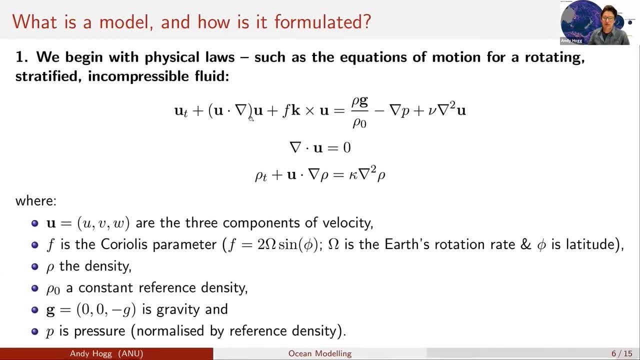 solve this: a set of equations for, for a global flow- and this is the term that's really responsible for all those small scale features that you were, you were seeing in that initial animation that i showed. this is a really difficult equation to solve numerically, um, so i'll. 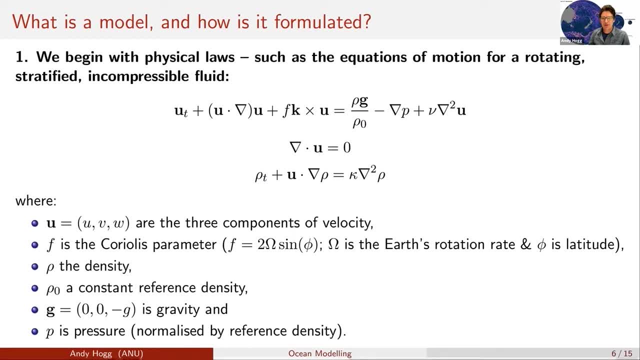 speak a little bit about how we do that in a moment. but, um, but rest assured, if we could solve this, we would have almost the perfect model for the ocean circulation. there's a couple of other things that are important. this is essentially an equation, which is, if you like, the conservation of 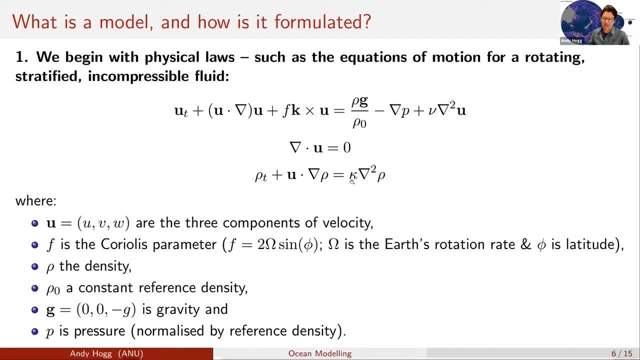 mass for an incompressible fluid and this is an equation for the conservation of density, quite often in the ocean. i would break that in up into the conservation of salinity and temperature. now, if you don't like looking equation at equations, that's okay, because i'm not going to show you any. 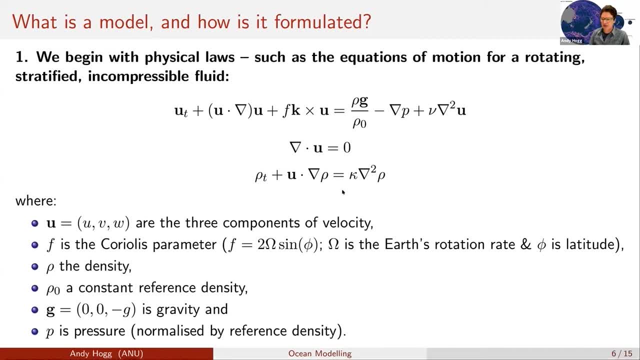 of these equations. most of the rest, i'm going to show you techniques about how we solve for these equations and and what we do, what we do with them. once we can solve for these equations, so let's move on to think about how we can solve these. so, as i said, this is a set of 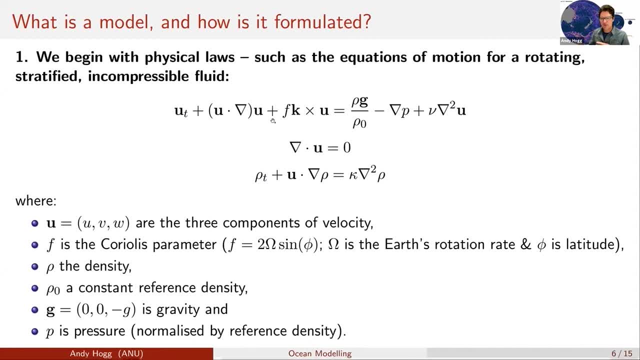 partial differential equations. that means this: these equations are full of derivatives. for example, this triangle: here is the gradient. this is the gradient of pressure in three dimensions: dpdx and dpdy. so to solve this, what we actually do is we break the earth up into a bunch of little. 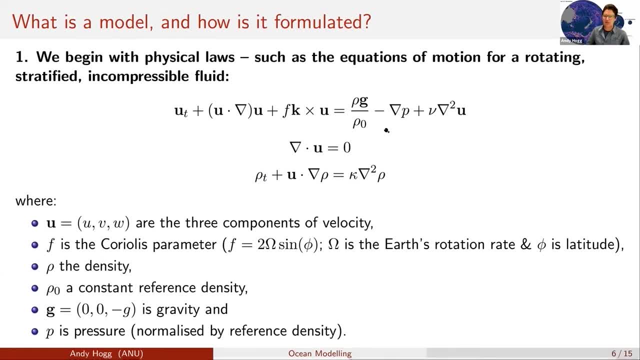 cubes, uh, and these, these little cubes allow us to approximate all of these derivatives. we can take the difference between the pressure at one cube and the next, and that will give us this pressure gradient that you're seeing here. so we take the earth, we divide it up into a set of cubes. 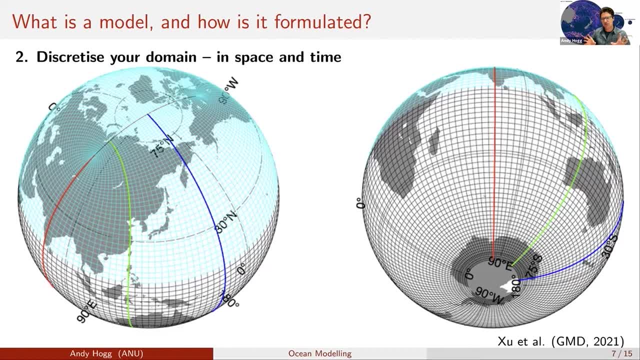 and we divide it up into x and y or latitude and longitude grid, like this, if you like. we'll also divide it up into a series of layers or vertical levels, and when we do that, we're in a position that we might be able to begin to discretize these equations. 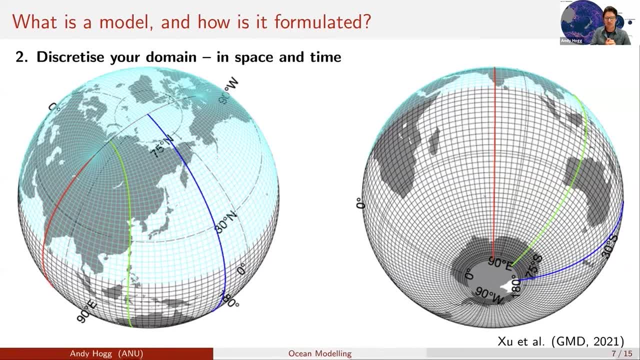 compute little gradients at each location. once we discretize these equations in space as well as time, actually, what we will actually do is that we can then feed it to a computer and this computer will be able to compute these things for us. so this discretization that you're seeing here, it's not a trivial thing and in fact what you're looking at here is a is. 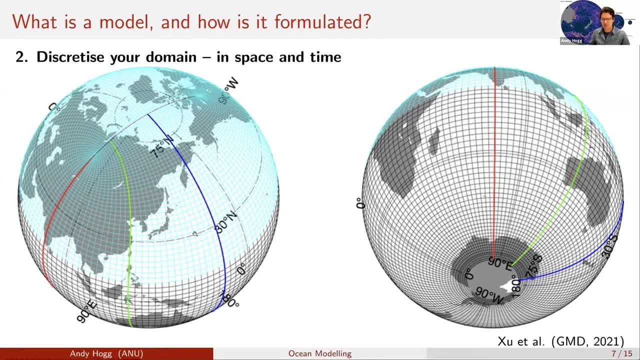 a grid that's about one degree by one degree. that's. that's quite a coarse grid, if you can see the, the model of the globe that's sitting in the image right behind me. that's a that's a 0.1 degree grid of a model that i'm running here at the moment. 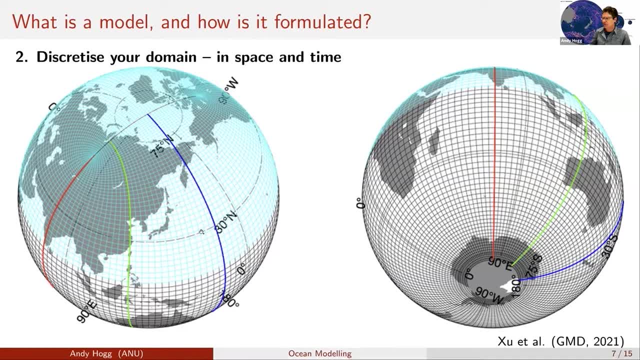 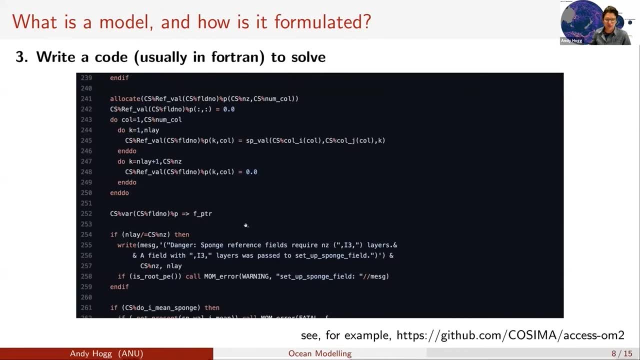 i'll speak a little bit more about that. once you get up to these really high resolution models, you you need a big computer. well, first you need a code and then you need a big computer. so a lot of the time we're using languages like fortran or python that we'll use to model the flow. 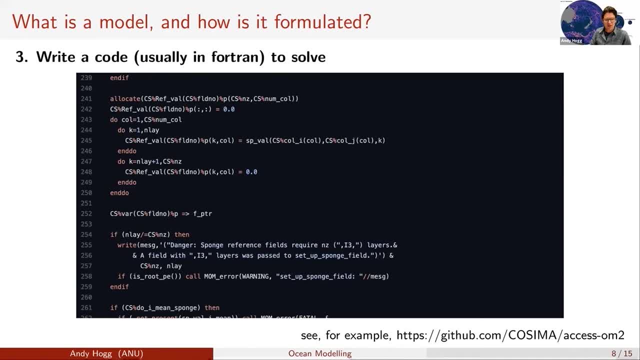 in the ocean. i just, i don't expect you to understand what this particular little tiny bit of code does, but in a, in an ocean model, we have hundreds and hundreds and hundreds of thousands of lines of this type of code, and all this code would be to solve those equations once we've discretized them. 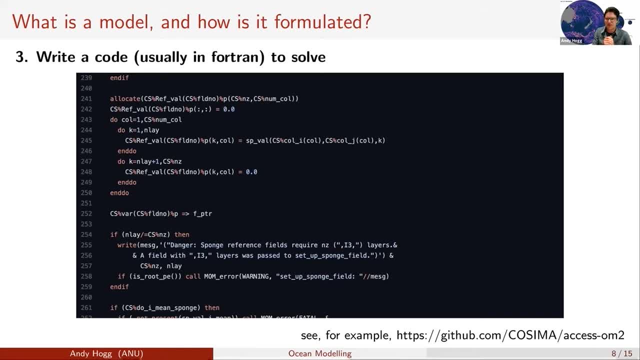 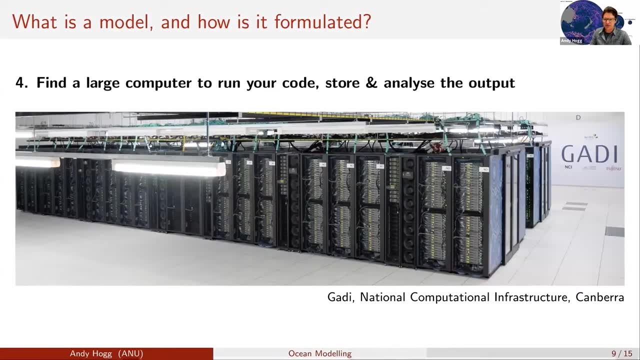 onto a regular grid which allows us to to solve for those equations, and the final thing we need is a really big computer. so here's a big computer at the national computational infrastructure, and the national computational infrastructure sits here at anu, in fact, if i hear out my window. 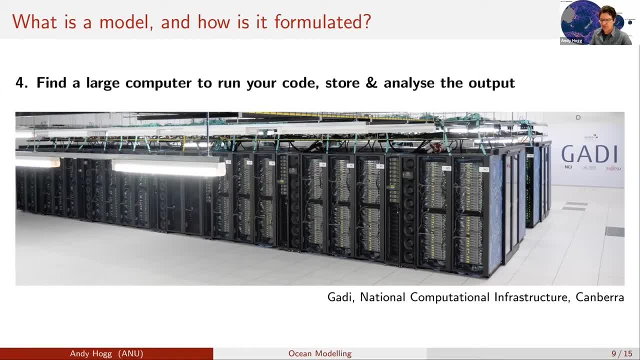 i can actually see the steam coming off the cooling towers that uh sit at the nci. this is their machine, guardi, there's uh hundreds of thousands of cores in this machine, uh, and, and this is the machine where we're running um all these calculations, and so an ocean model is really. 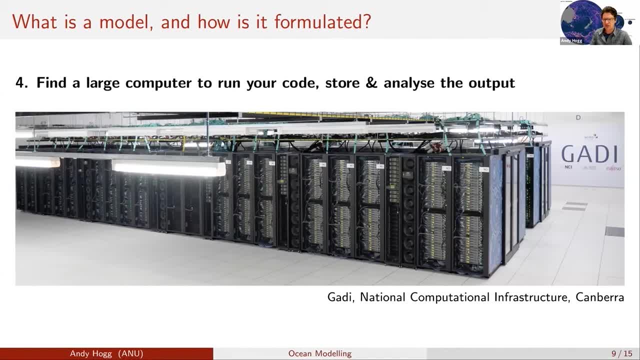 you know it's a set of equations. that set of equations is is uh choppy up into little bits so that we can estimate uh derivatives. those derivatives are coded up into a fortran code or some other coding language, compiled and put on a computer like this, and then 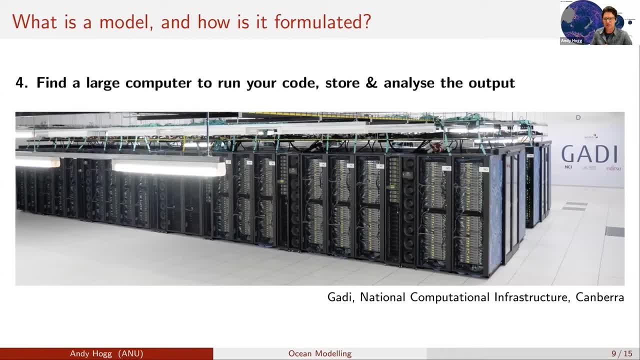 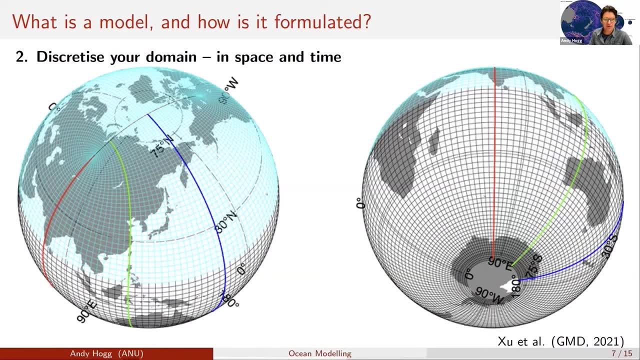 and then the output comes out and we see how things go. so just a just a point i want to make before i go any further. i'm going to jump back to this slide here, where i'm talking about the discretization, and here there's- we've always got a trade-off. 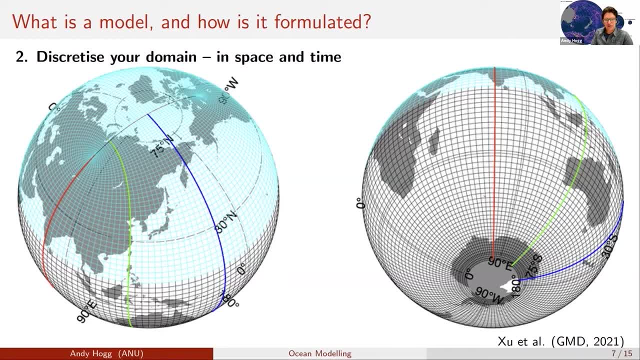 so in in this particular grid it's about one degree by one degree and that means we have around about 360 by 180 points in the horizontal, plus maybe 50 layers in the vertical, and we want to integrate that whole system forward in time for 10 years, 100 years, whatever we like. 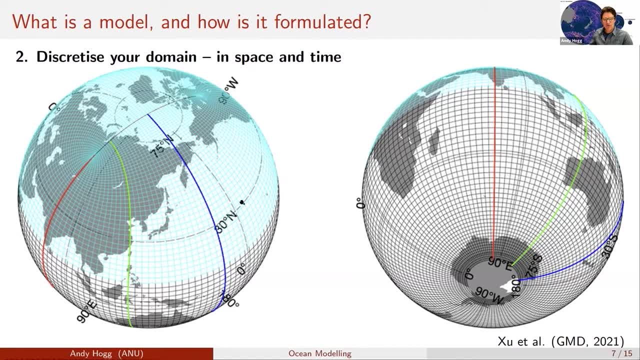 so, um, every time we compute something on one of these grids, we have to ask the computer to compute. so obviously, if we have less grids then we have to make, you know, less computations. and so if we space all these grids out, then we have to make less computations and actually our model runs. 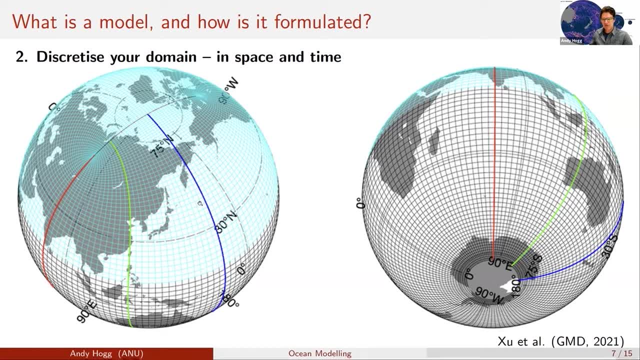 much faster. but if we space these grids out, then we can't resolve all the processes that are going on. and so if we want to resolve all the processes that are going on, we need a really fine grid, and in fact, the processes in the global ocean can vary between the millimeter scales of uh, of convective turbulence. 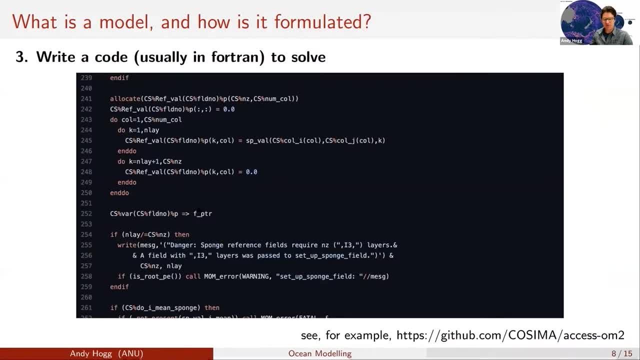 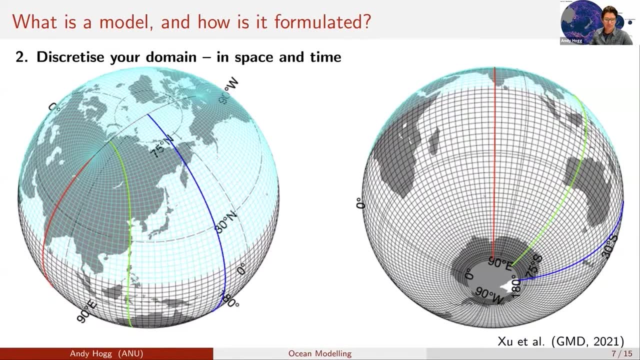 and the base, and wide hundred kilometer scales, that, excuse me that, that you're seeing, um, as we go across the, uh, the whole globe, and so, uh, what we have here is we have a compromise between the number of grid points we use and the number of grid points we can afford, so the more we can, 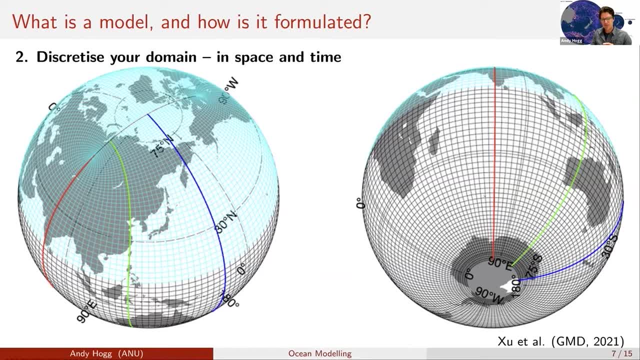 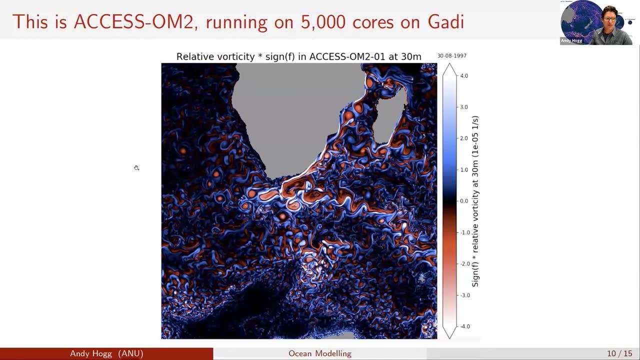 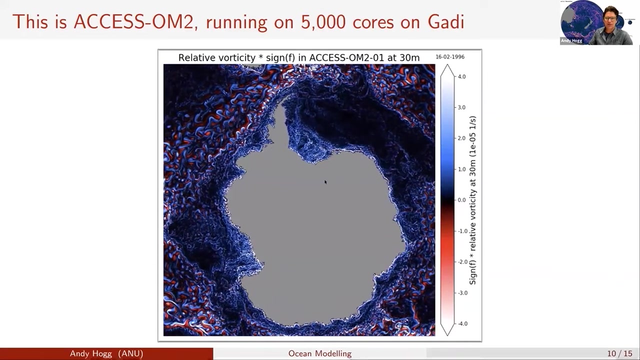 afford. the more processes we can resolve, the better will be the physics of our model, but the computational cost of that is is it can get immense. okay, so i'm going to, uh, i'm going to show you a few examples of um, of how we use ocean models, and a lot of these examples come from a. 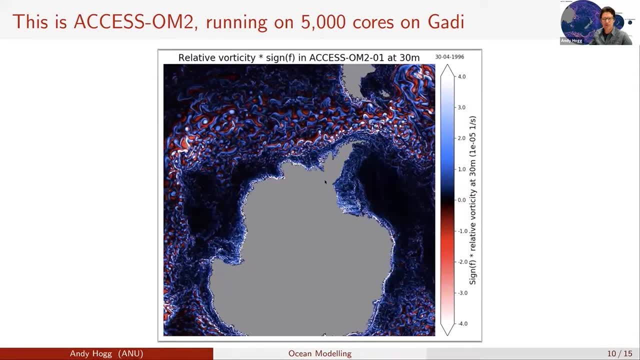 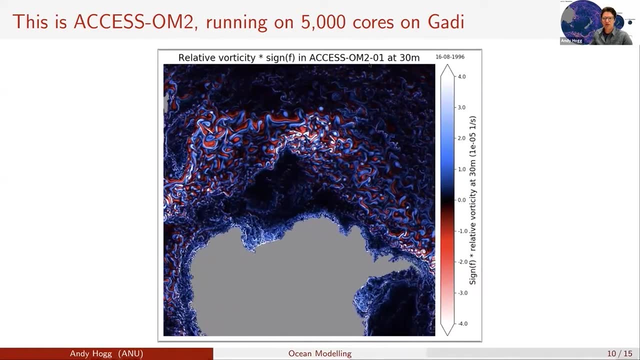 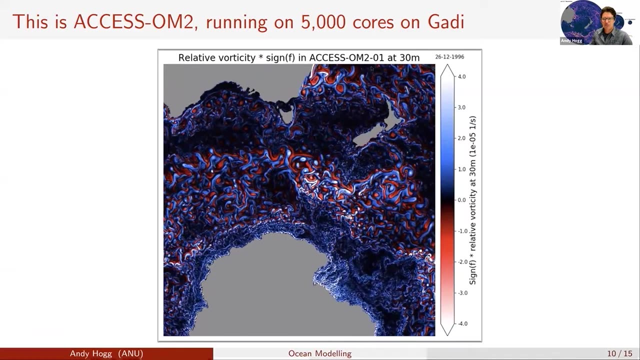 model that i helped to build here at anu. it's called access rm2. um, what i'm showing you here is the 10th degree uh climate model. this is a little animation. i hope it doesn't make you too dizzy. it's a little choppy on my machine. it's probably a bit choppy on yours as well. 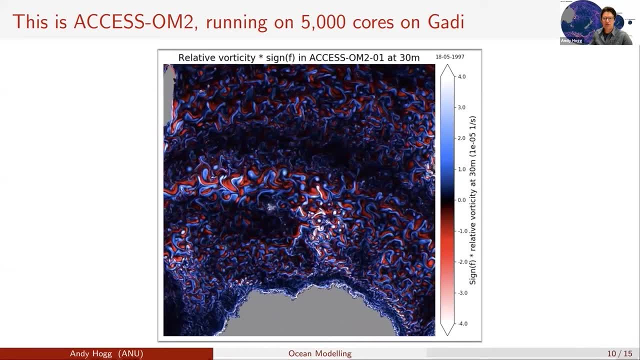 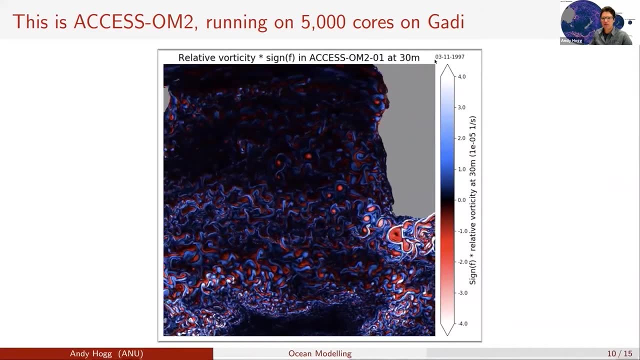 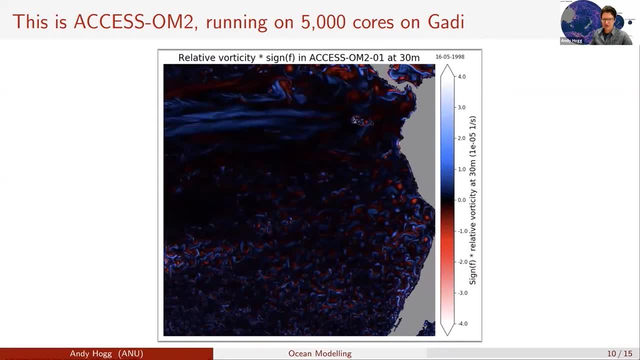 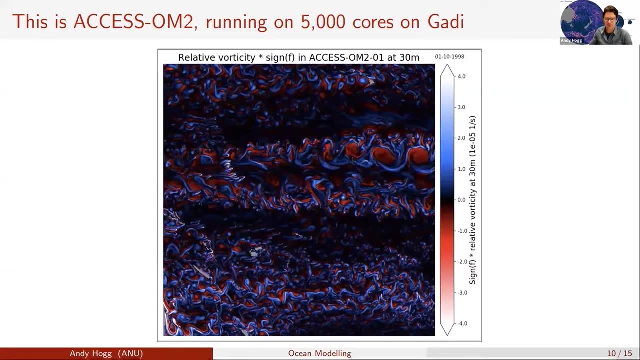 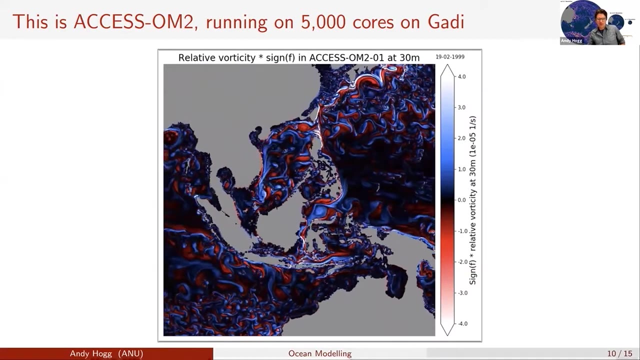 line moving ahead and the point is that these, uh, this relative vorticity is a good tracer to really understand the dynamics of of what's going on. so you can see, in the tropical pacific we get all these large-scale eddies as we go past the top of australia, through the indonesian archipelago. 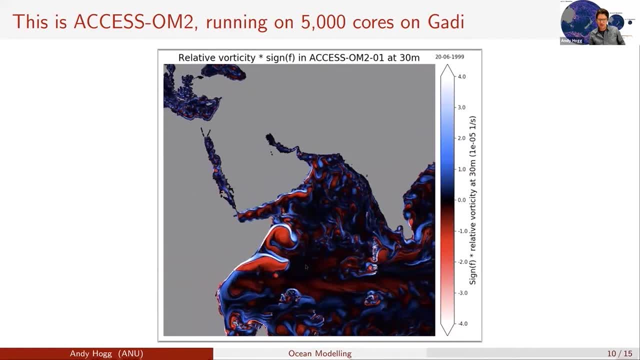 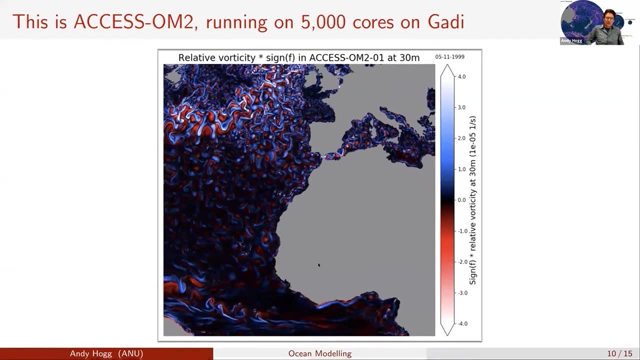 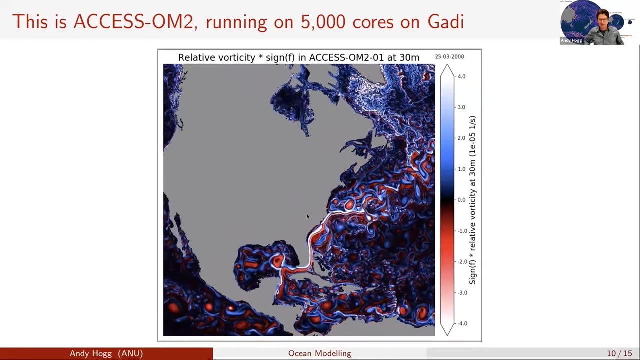 we see lots of boundary current interactions. we see this comb-like effects and eddies that are happening in the arabian sea, and so you can see the this uh simulation is picking out a lot of the dynamic features. this is the gulf stream ripping up the coast of america. in a moment we're going to see, hopefully, the curashio which is on the other. 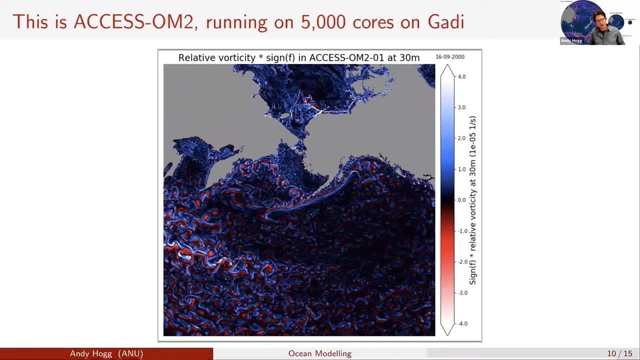 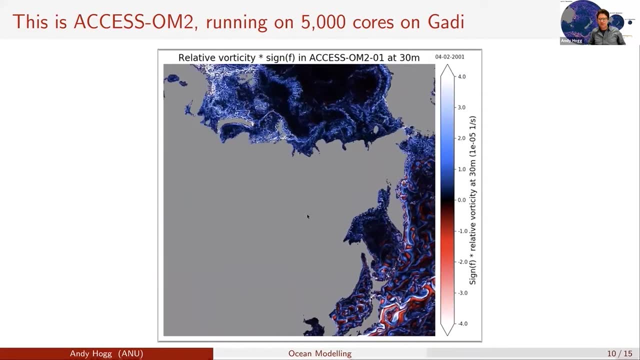 side of the pacific, or maybe we'll drift too far north before we see it. no, here's the curashio, off the current, off the coast of japan, and to get a simulation like this, what i need to do is i need to um is i need to run the model for. 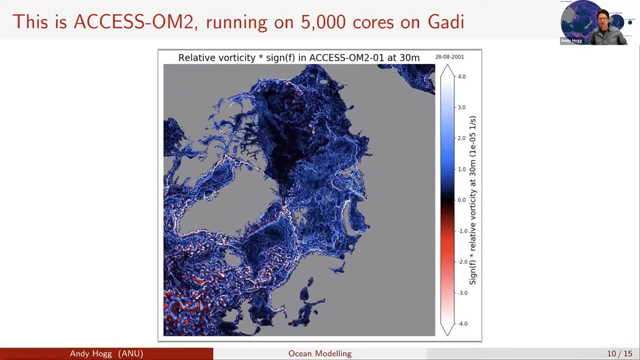 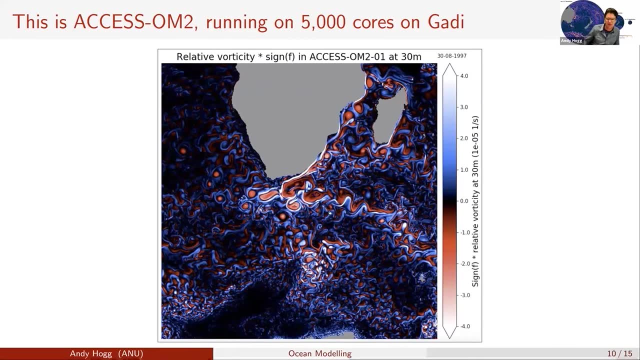 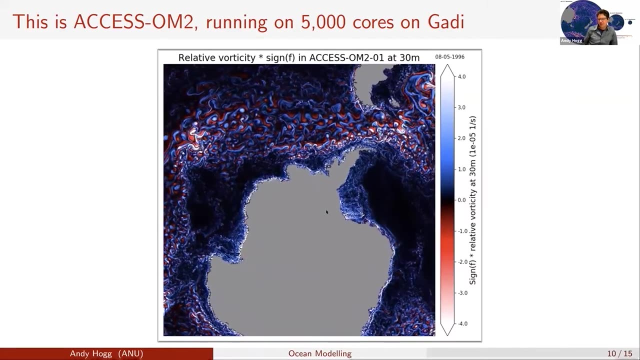 uh, on something like 5 000 cores on our computer here. actually the model scales to something like 20 000 cores, but i can't get that through the cube because we don't have a, we don't have enough computer time. um and um. roughly speaking, i spend about 50 000 compute hours per year of simulation. 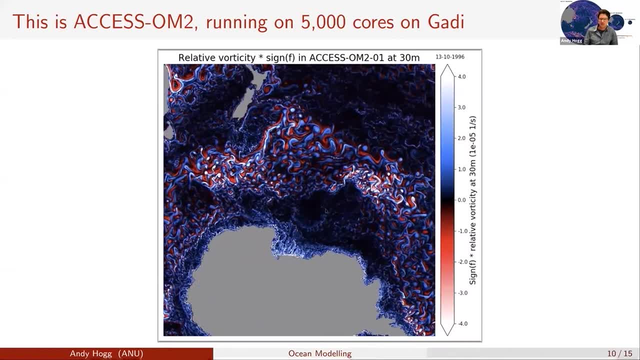 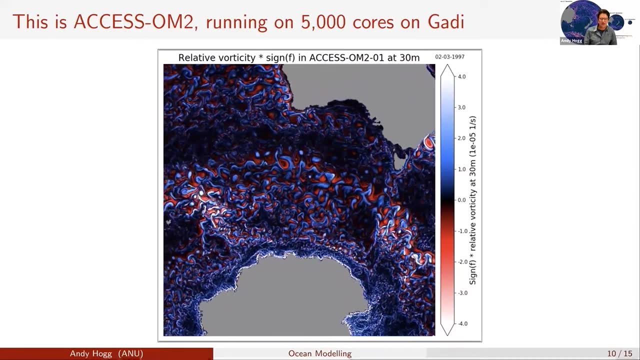 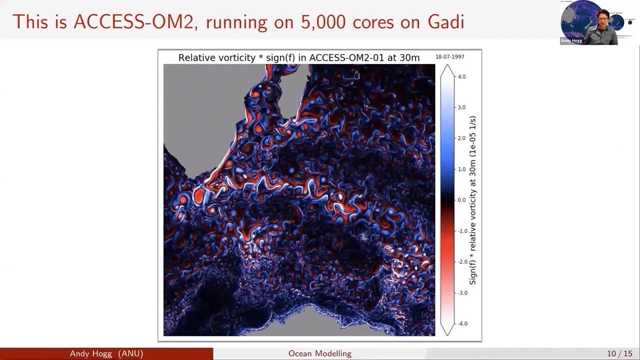 often. i want to run this model for 10 years, 100 years. our longest run has gone for 300 years, and so um and uh and so on. so so this is the access im2 model and i'm going to show you a few of the 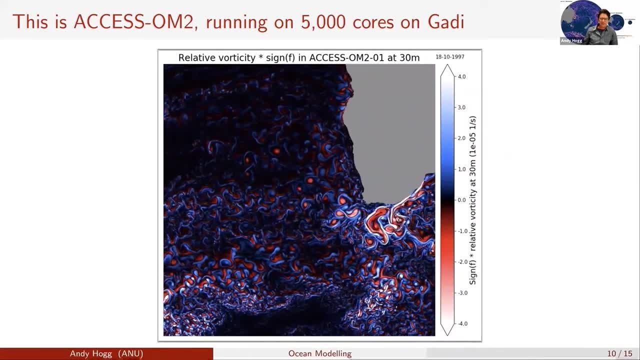 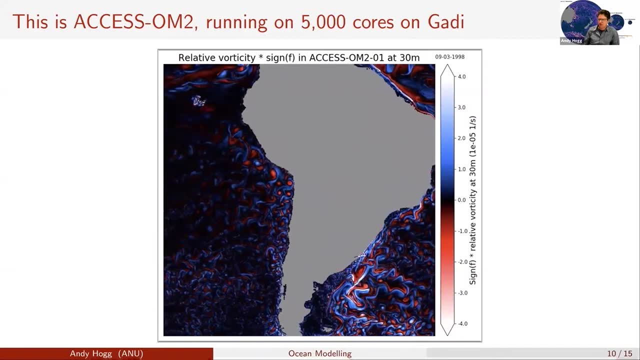 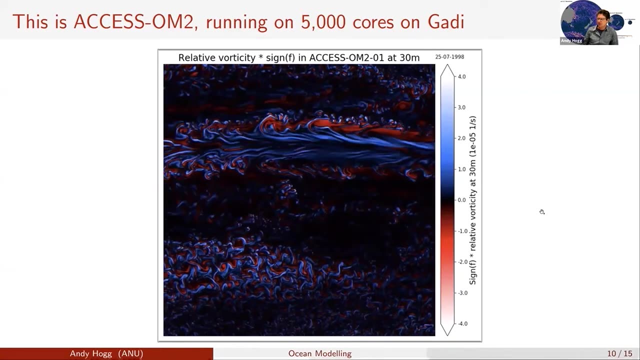 types of research questions. we can answer with that. as i'm going through these, i i just want to encourage you. if you have a question, you can ask the question on the q a, um. i'm going to, um. i'm going to get to those questions, most likely at the end. 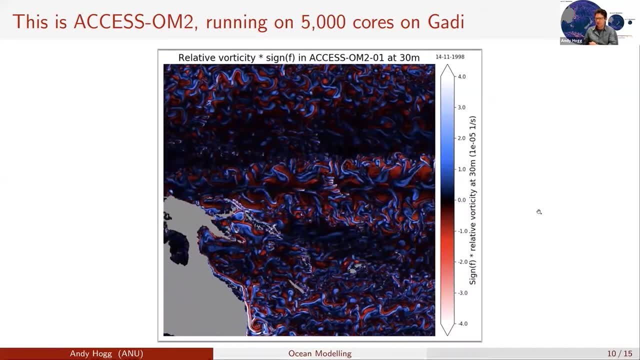 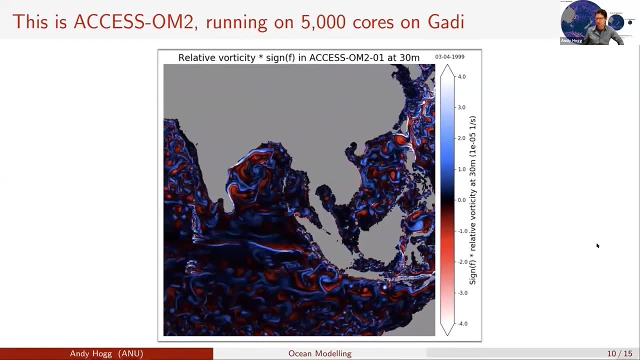 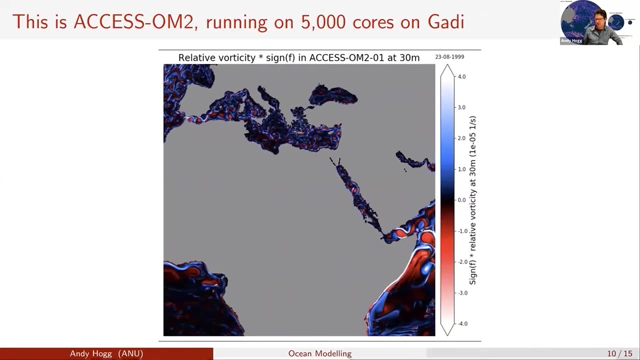 of the presentation: um and i'll. i probably won't interrupt my talk, um and but i'll, um, i'll. in fact, i can see that there's a question here which i actually want to answer right now, which which may help some of you, so i'll do that now, and that is. someone asked why we use relative. 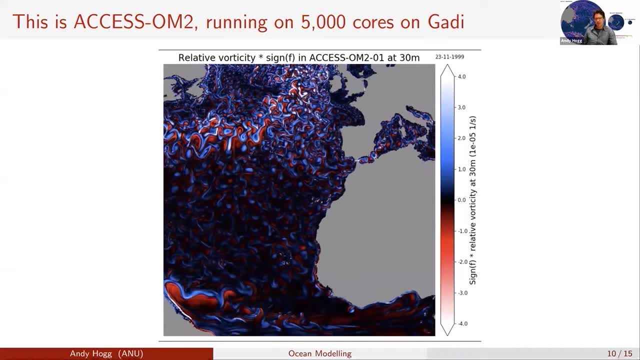 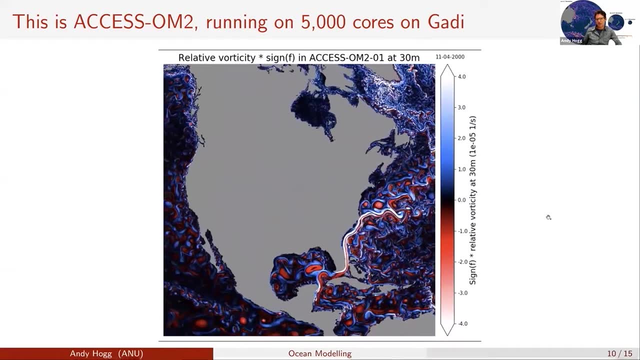 vorticity instead of relative velocity. what is its significance? and the vorticity is? you know, it's actually derived from the velocity itself. the reason i'd like to show vorticity sometimes is because it really brings out these eddying structures, so you can see these circular eddying. 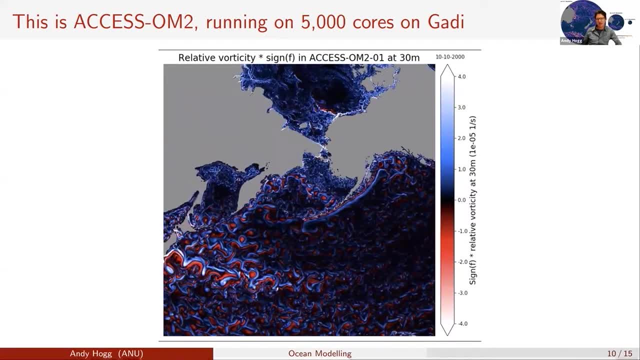 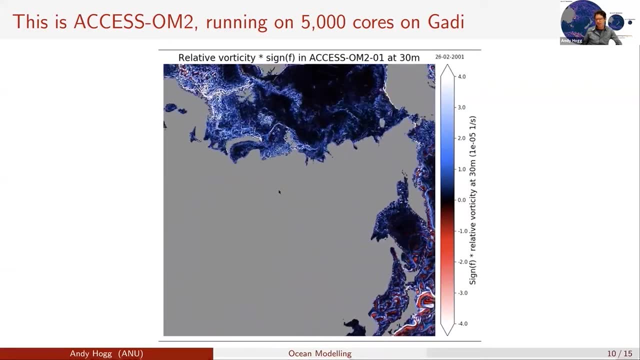 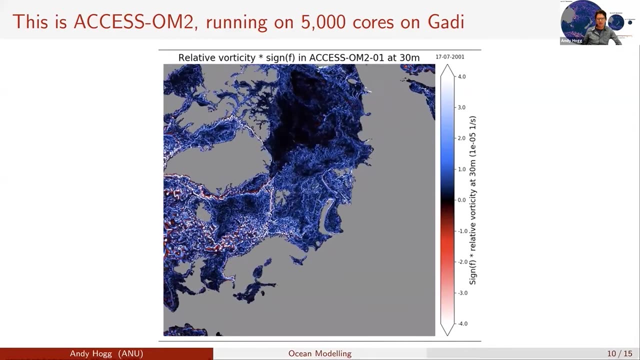 structures, and that's just brought out a little bit more in the relative vorticity. you can also see them in velocity. so this is really- i would call this simulation- eye candy. this is just something that i want to um, that i want to show, um, uh, just just to show what these patterns look. 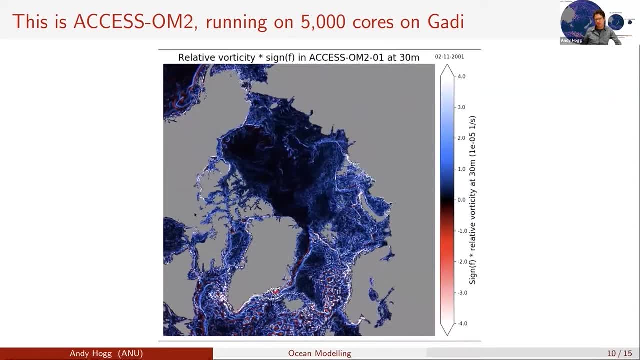 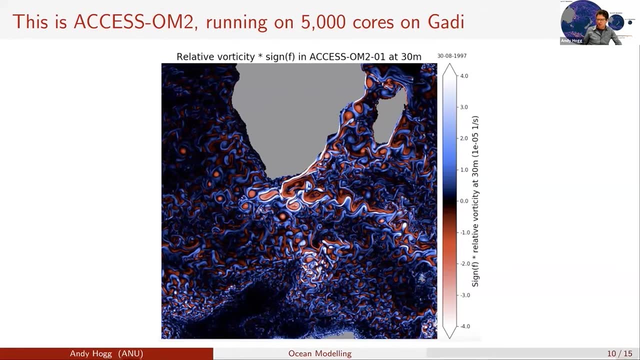 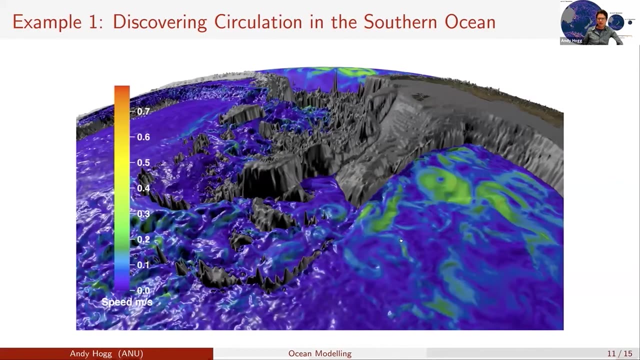 like in the ocean, um, and really, and just to emphasize just how dynamic uh the, the, the ocean is. so, um, i'll come to some of the other questions, uh, later, but first i want to elaborate a little bit on some of our, um, some of the bigger projects we're doing here at anu. um, and this might 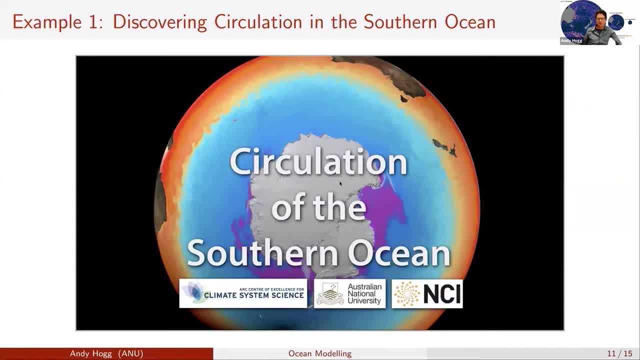 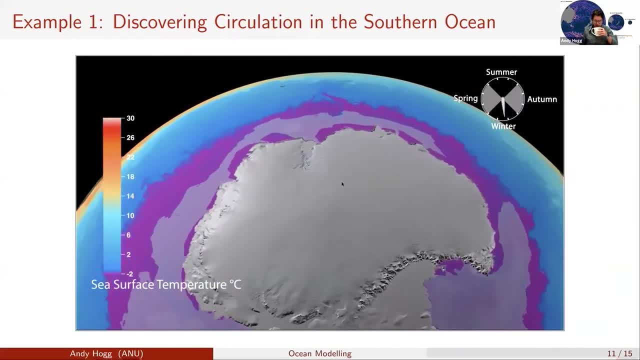 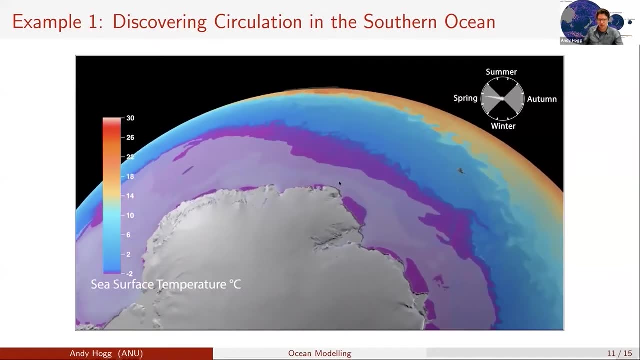 help to answer some of your questions that i can see coming through, so i'm going to show you now an animation of from this model that's going to focus on the southern ocean, and the southern ocean is a is a big uh topic of research for our group, and one of the reasons is 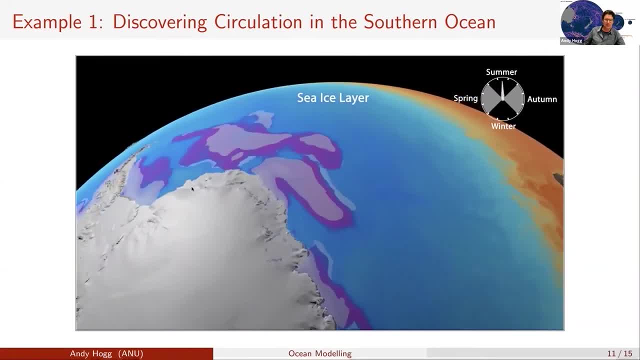 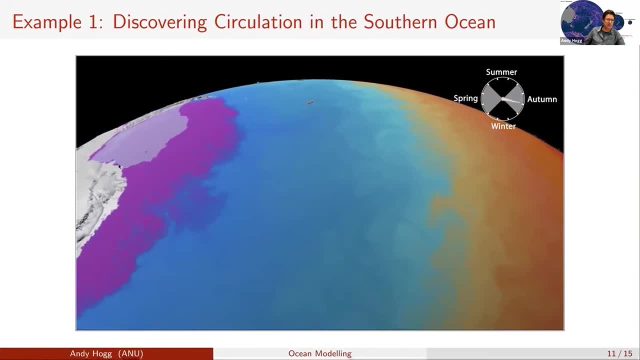 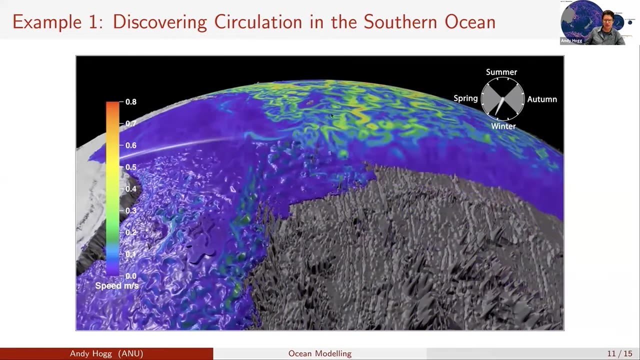 because we're very interested in what's going on close to antarctica, where you can see sea, ice forming and the ocean sitting upright against the uh, the continent here, where there's ice shelves that are beginning to rapidly melt and this is actually showing the the velocity at the surface. 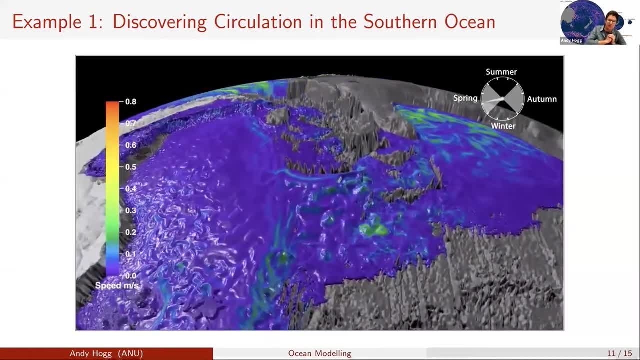 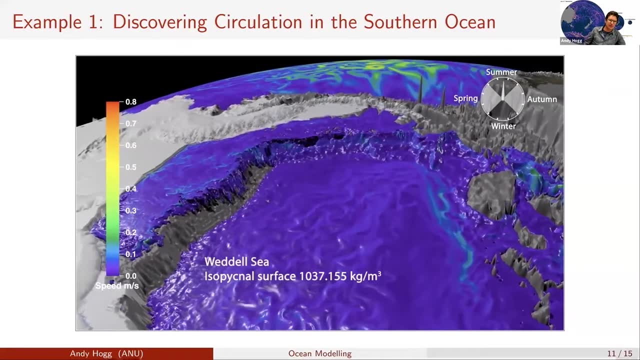 here. but what i actually want to do with this simulation is to peel back what's going on at the surface and look at what's going on at the surface and what's going on at the surface and on at the bottom of the ocean. so what you can see here is that we're taking a, what i call an. 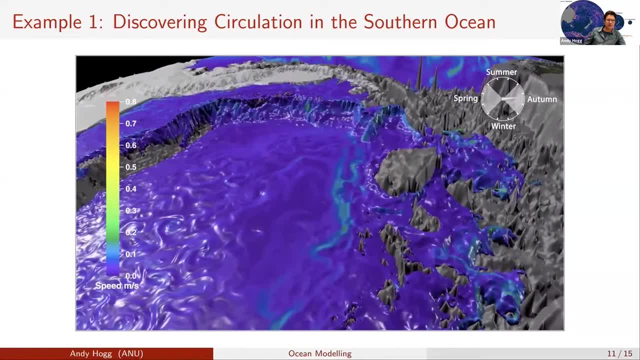 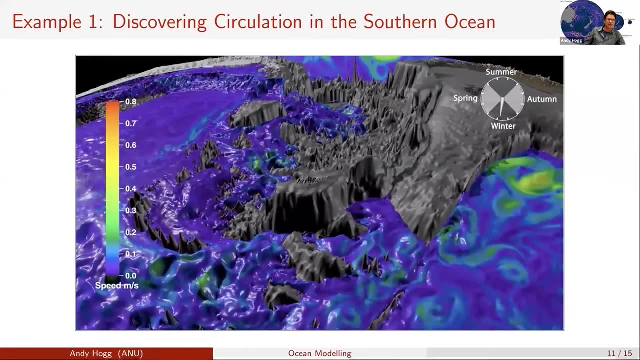 isopic layer. this is a layer of constant density and i'm looking at velocity or speed on this, on this surface, and you can see that there's really dense water up on the shelf here, the the antarctic continental shelf, really close to the continent, and that water cascades off the 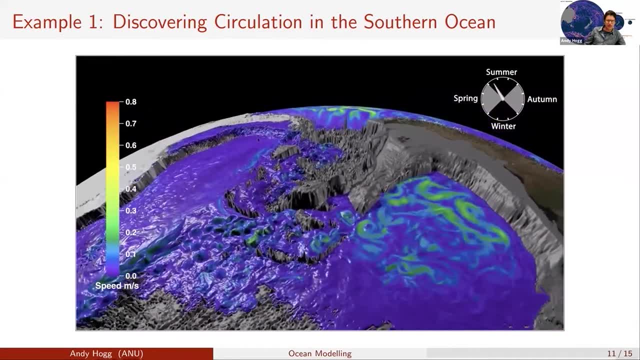 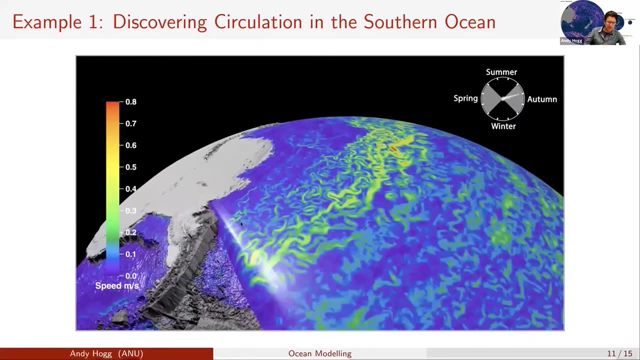 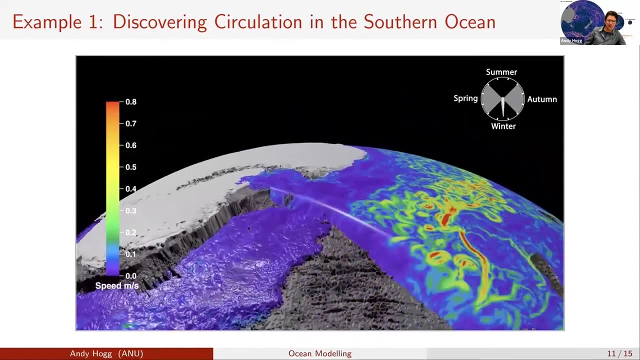 shelf, a bit like a massive underwater waterfall, and then fills up the basin at the bottom of the ocean and that dense water just sort of sits there as we peel back and look around at the ross sea. i'm going to look at another surface here. this is another part of antarctica again. 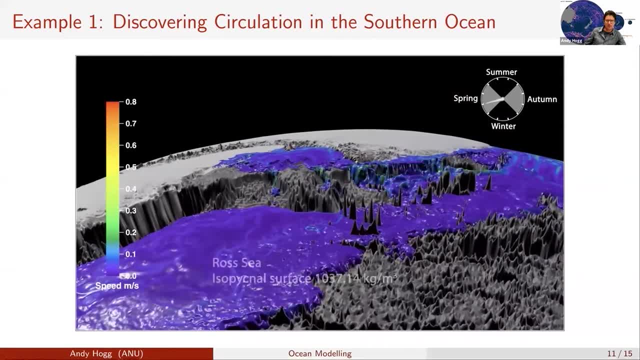 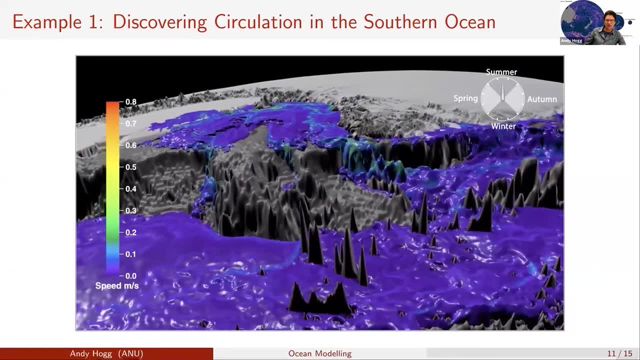 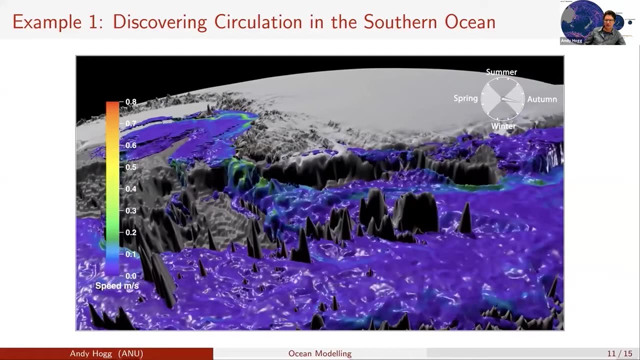 this part of antarctica is also associated with really cold, dense water forming up on the shelf here and you can see these waterfalls flowing off the, these dense waterfalls flowing down, getting down to what i call the abyssal ocean and then flowing around and and. 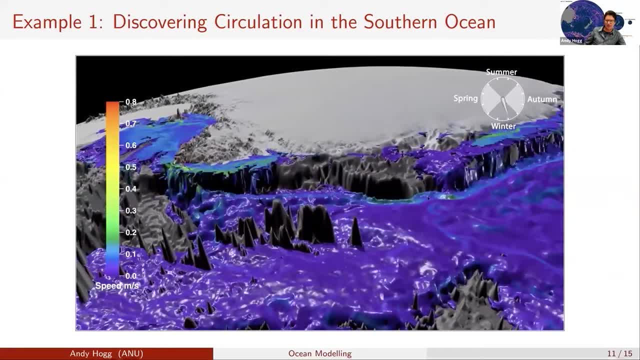 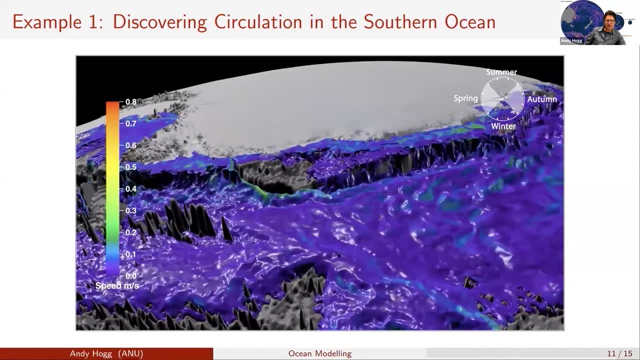 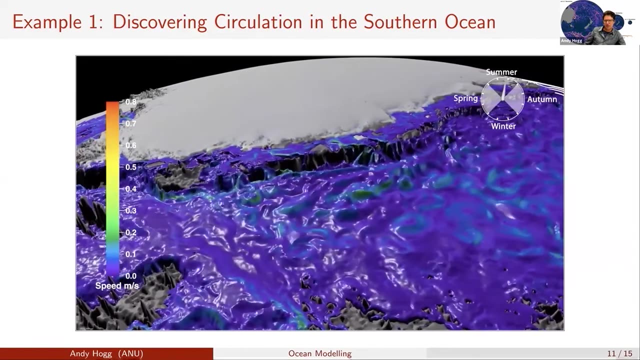 doing a lot of, a lot of dynamic interaction with the topography and the symmetry in those lower regions. so this is a process that we call a process that calls causes the formation of abyssal water. it's a type of water that we oceanographers refer to. 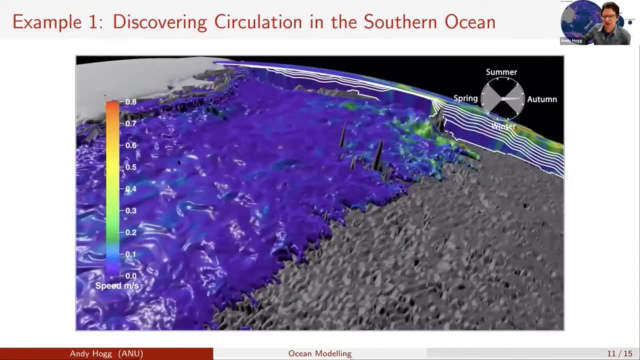 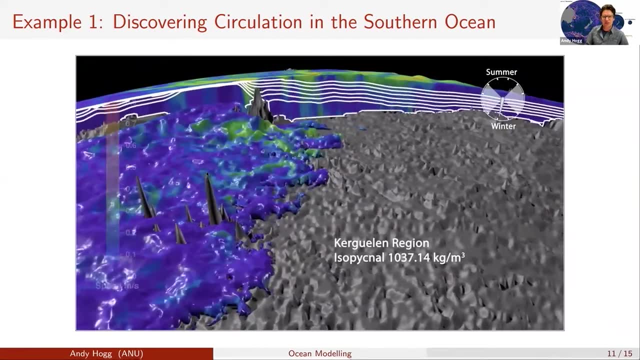 as antarctic bottom water. and the antarctic bottom water kind of fills up the very bottom of the ocean and so the bottom water is basically the the bottom of the ocean and sits there for a very long time. in parts of the Pacific Ocean water can can be at. 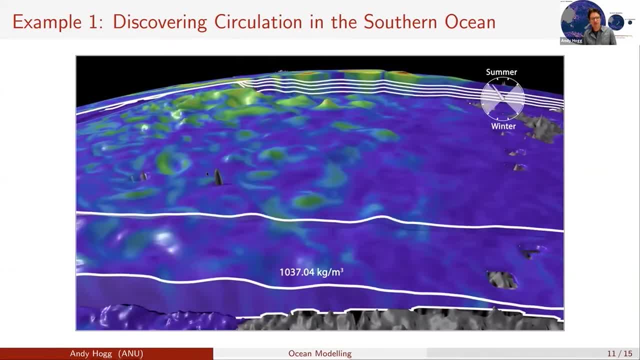 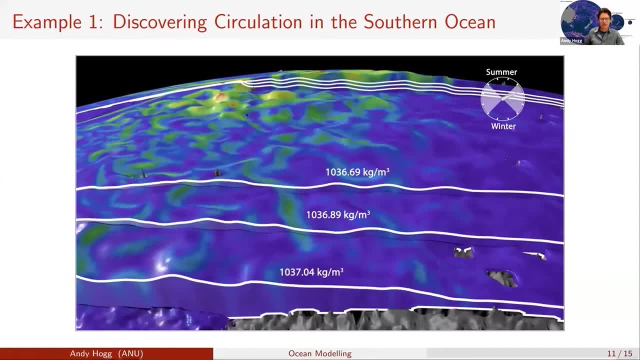 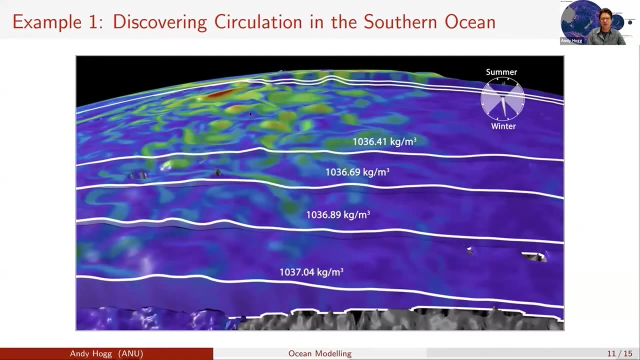 the abyssal part of the ocean for thousands of years before it gets back up to the surface. and when we look at this is this is now looking at more in the middle of the Southern Ocean and it's showing how much, how dynamic, the intermediate depth field is, with all these little features that we call ocean. 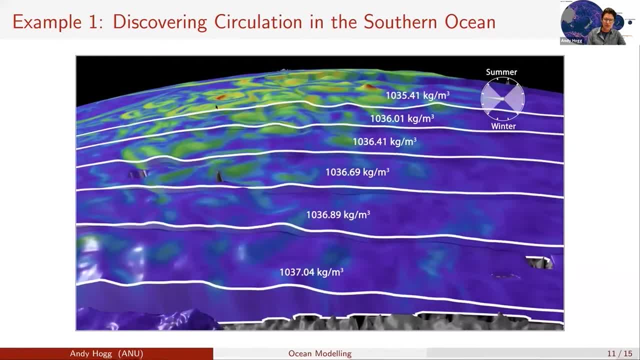 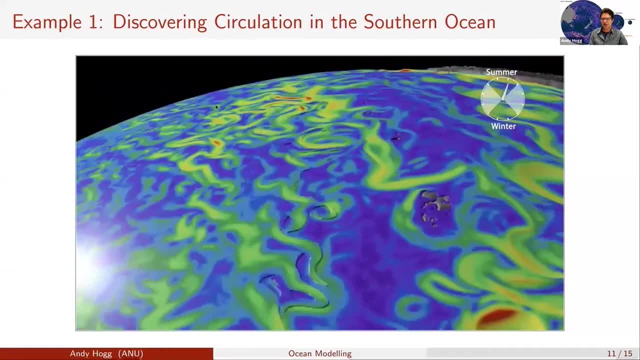 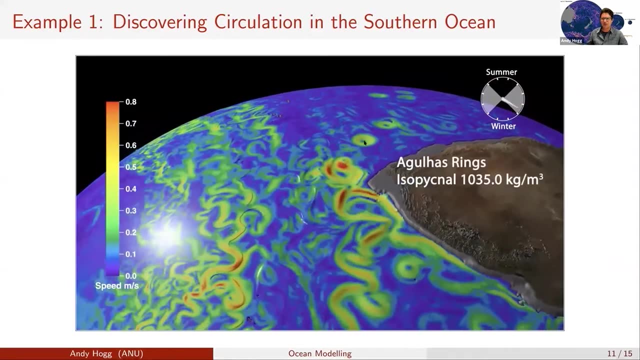 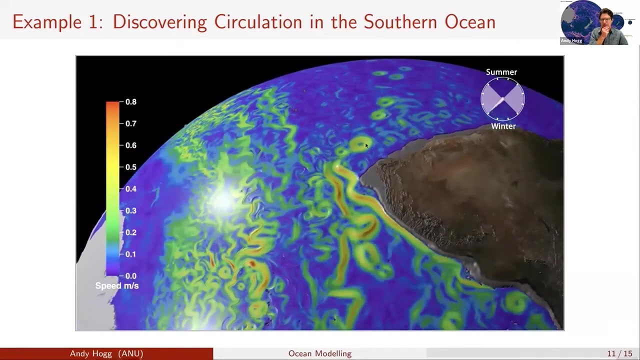 eddies that are always moving around, and so the the ambition of this, of this animation, is just to give you an idea of what the just how dynamic these features are, particularly these eddies that you can see off the coast of Africa here, but also to give you a feel for how close to Antarctica this bottom water can be. 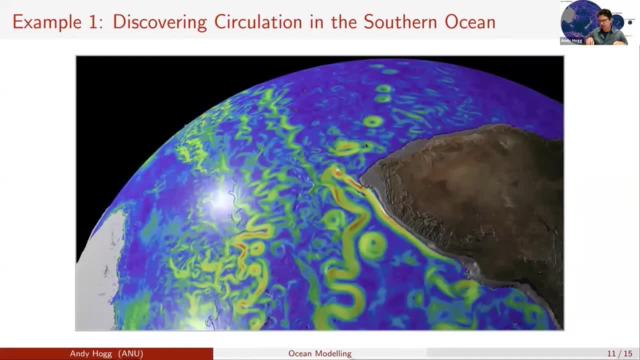 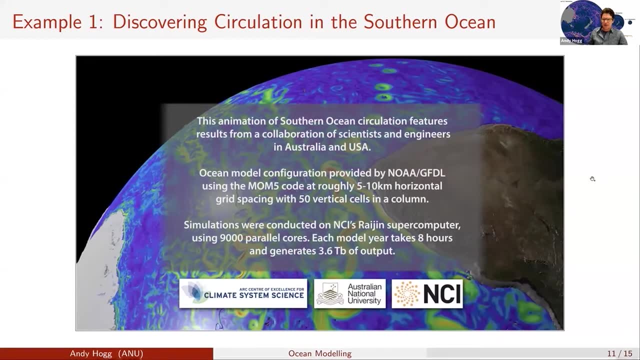 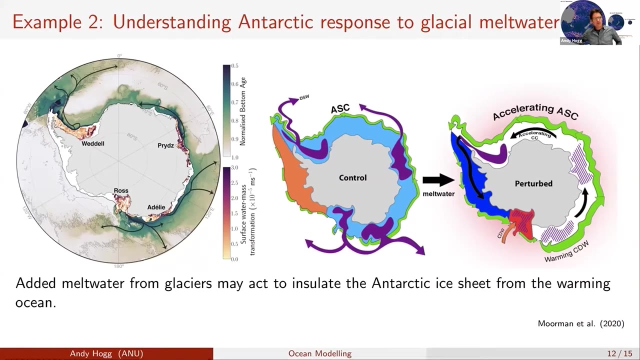 formed. this bottom water is really dense and cold, and it sinks right to the bottom and stays there for a very long time. okay, so I'm going to jump forward to to understanding one of the projects that that is key to our work here, and that is to use this model to understand. 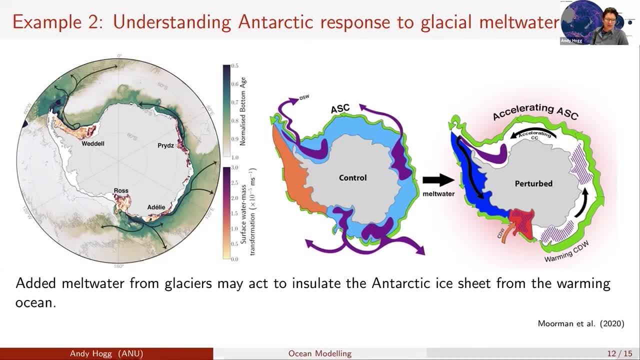 how things may change in the future. so many of you may have heard that the ice shelves around Antarctica- that's fringing around Antarctica here- that the ice shelves are causing a lot of melt water and this melt water puts fresh, really low salinity water into the surface regions of of the coastal. 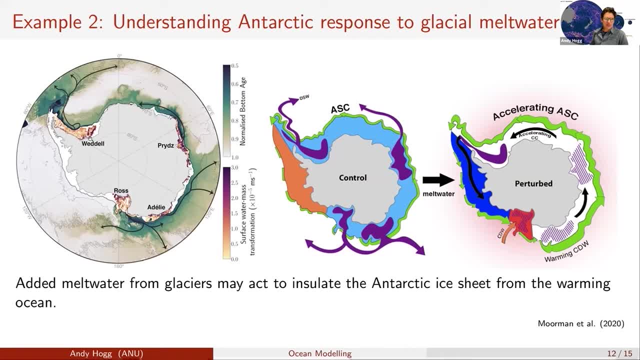 Antarctic Ocean and this coastal Antarctic Ocean water is really important because, as as you just saw in the in the recent movie I showed, this coastal Antarctic region forms really dense water which follows these pathways down into the, into the abyssal ocean, and it's really important that the ice shelves. 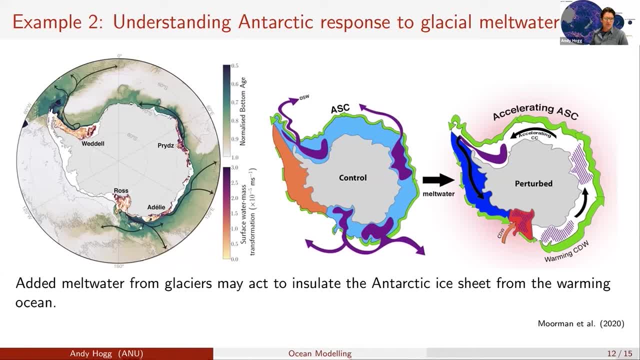 that the ice shelves are causing a lot of melt water and this melt water puts extremely highius bubbles in these 설명 audio. and one of the things we want to know is: well, if melting of antarctic oceans is of Antarctica ice shelves is going to continue, how is that going to affect the 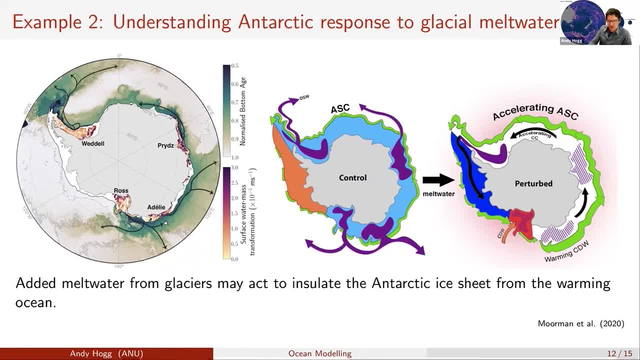 bottom of the ocean. give me, when I turn my lights on, how's that gonna affect the bottom of the ocean? and so one of our students a couple of years ago worked on this question and what she did is she took this model and, instead of trying to have views of the ocean, most of the science we learned was out that. 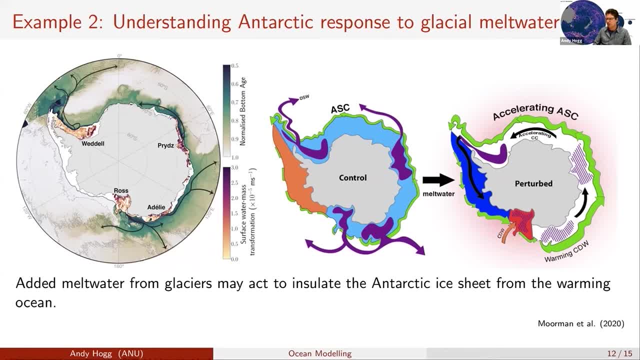 replicate reality. she used a scenario to jump forward to the year 2100 and to dump in the amount of fresh water that we expect to be melting off glaciers by 2100, and when she did this, she found that we went from a state of the oceans around Antarctica where we would put in a lot of 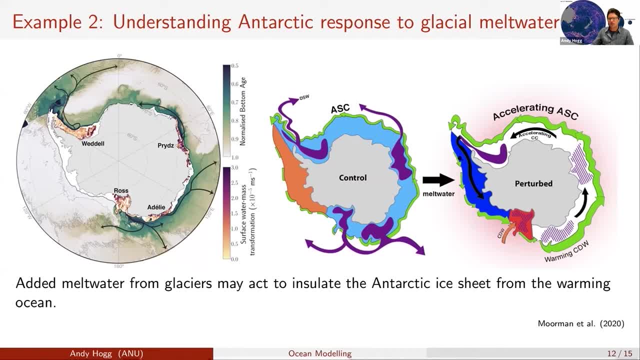 fresh water, and this fresh water would cool part of the Antarctic shelf here and it would warm other parts of the Antarctic shelf, and so different parts of the Antarctic shelf responded differently, and we can only get this signal when we, when we have a model that isn't fine enough. resolution. 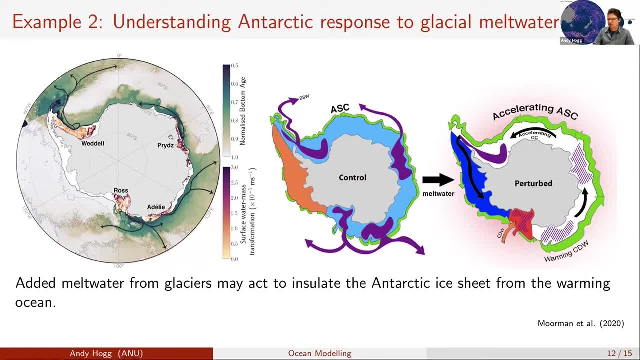 to really represent all the processes that are going on here. so the idea here is to is- and this is a little bit in reference to one of the questions which I'll come to later- is to avoid using sub grid scale models for things. it's actually, it's actually here to to simulate. 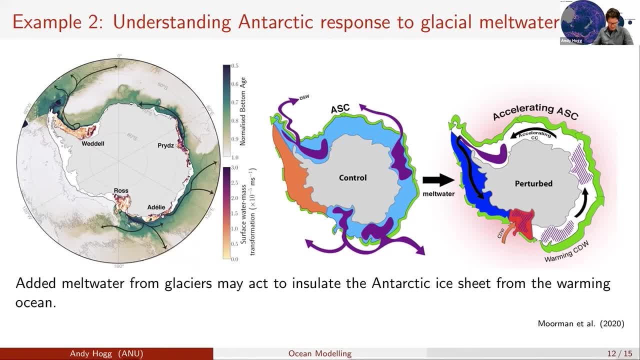 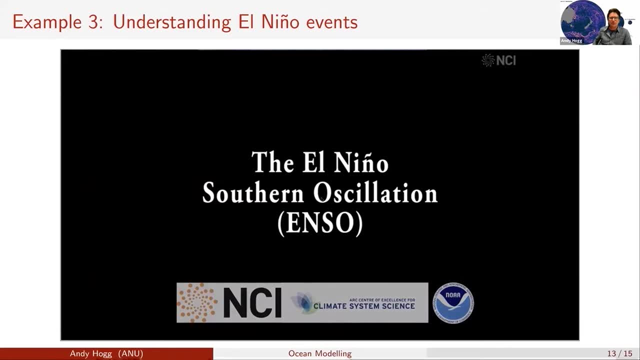 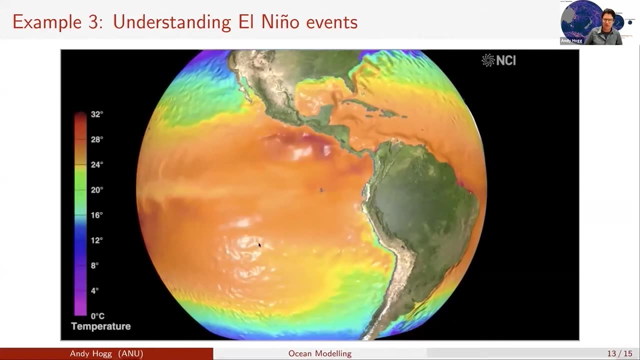 as many of the important processes that we, that we think we can. okay, I'm going to move away from the Southern Ocean for a moment and I'm going to talk about something else which which is important to the ocean, in fact to the climate, which is El Nino and, and many of you will have heard of, El. 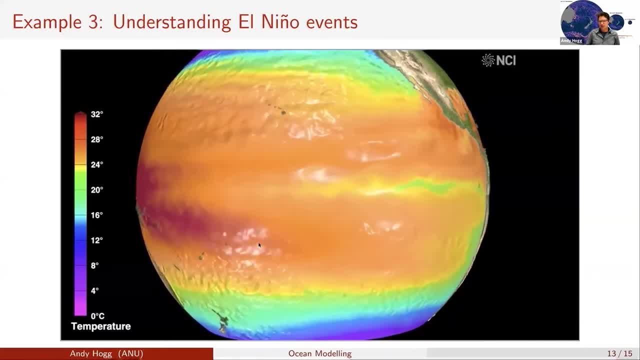 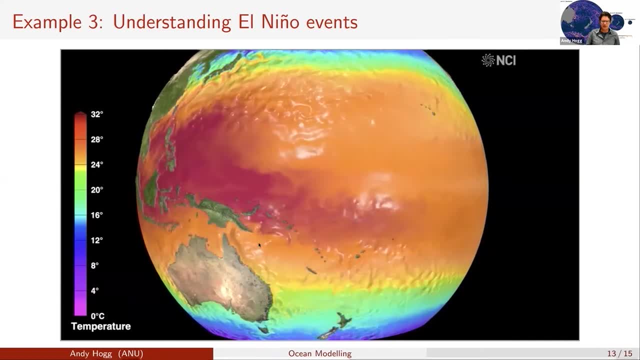 Nino, and many of you will have heard of El Nino, and many of you will have heard of El Nino and before, but you may not really understand a lot about the dynamics of what's happening with El Nino, so I just want to show you this animation, which is again something we made from our ocean model. 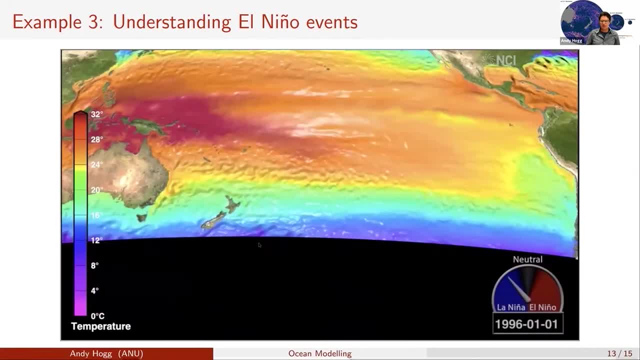 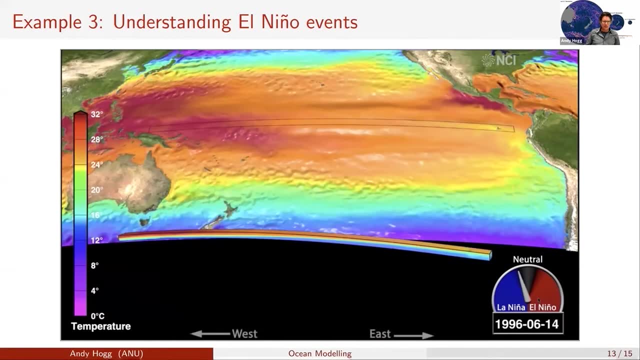 and this is simulating an El Nino event which occurred in 1997-98, and we've got a little El Nino meter down on the right here and to help show what's going on here, we're going to pull out a little bit of water from the along the equatorial Pacific and you can see that. 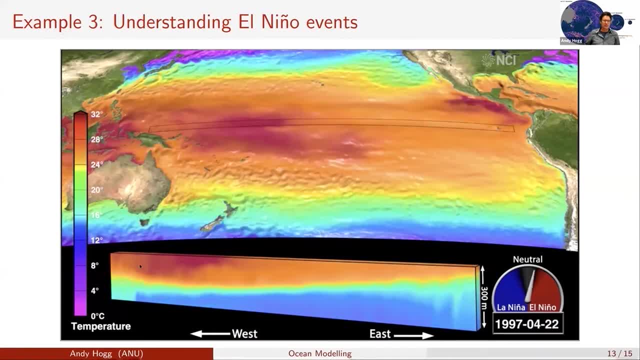 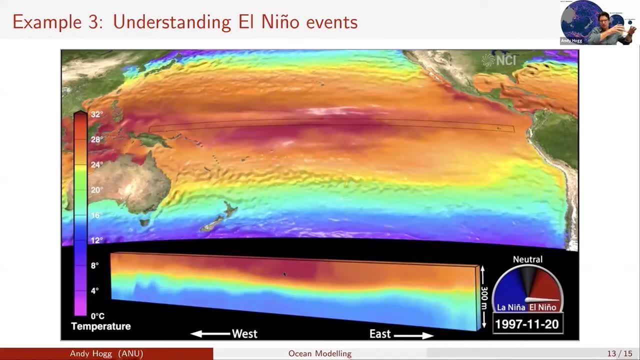 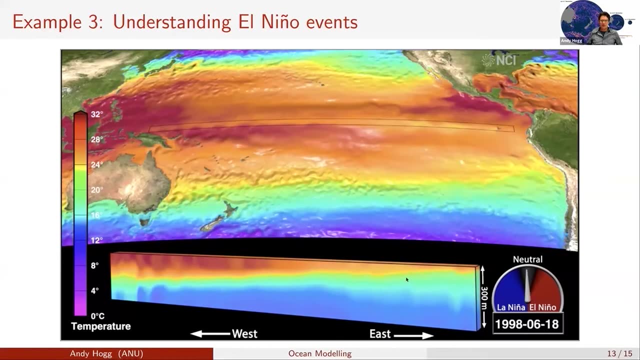 in the normal course of events, the Western Pacific is really warm and the Eastern Pacific is less warm and when we come into an El Nino, this warm water from the West Pacific floods back across the Pacific and you can see that the El Nino causes this warm water to to be in the East. 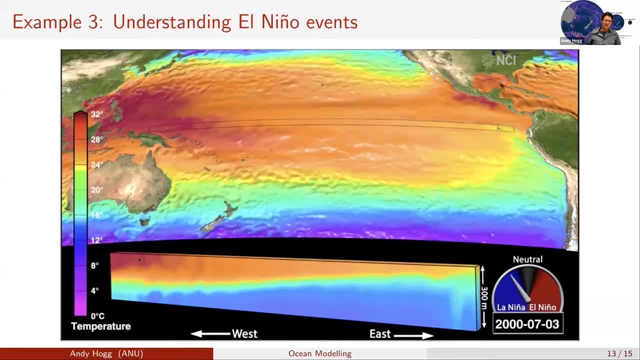 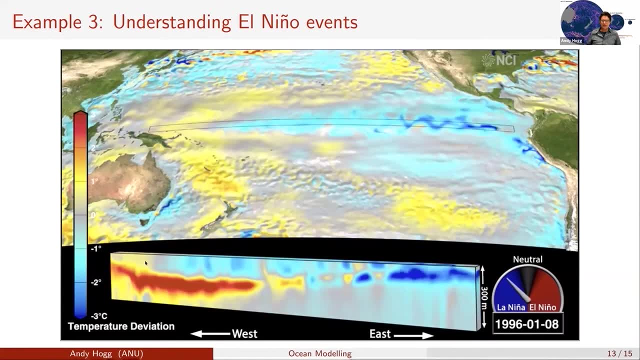 Pacific. when we come back to El Nino, the opposite happens and you can see now that the warm water is really piling up in the Western part of the ocean. you're going to see that again now, but you're going to see that again in anomaly space. so we're now looking at the temperature anomalies. 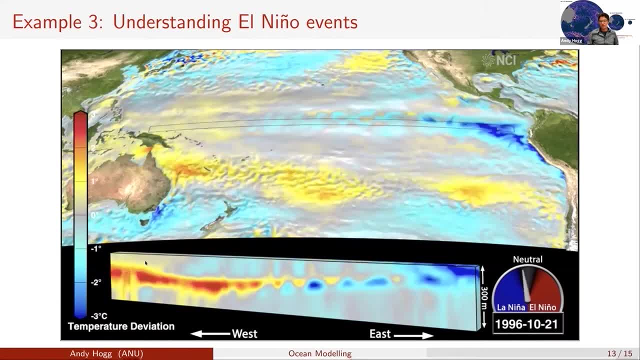 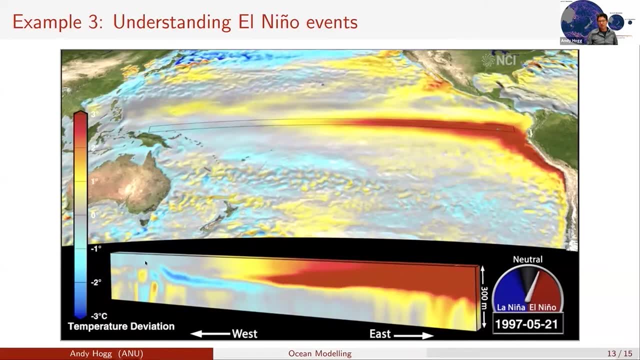 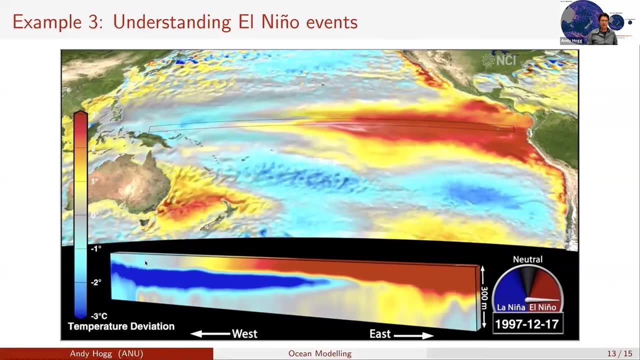 and you can see that, you will see in a moment that as we launch into 1997, when the El Nino started, all this warm water floods across to the East. this causes huge amounts of rainfall and flooding in in the Eastern Pacific. but for those of us in the Western Pacific, like Australia and Indonesia, 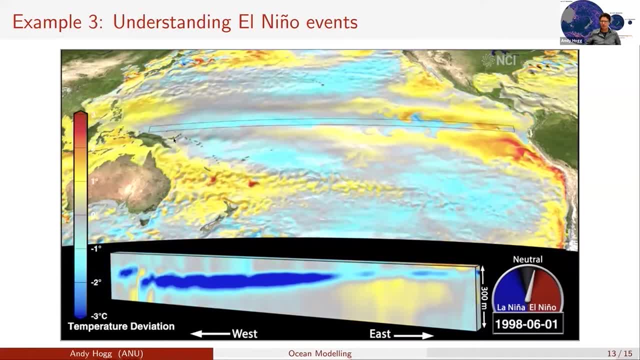 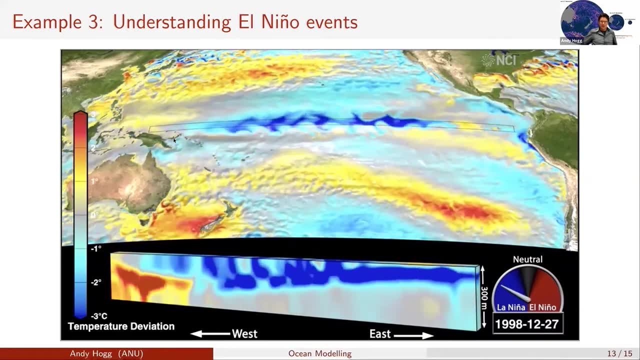 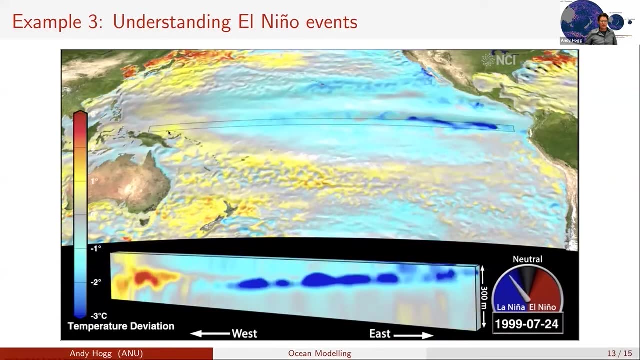 we experience dry conditions because the ocean is so cold, the tropical ocean is so cold. there's less evaporation, less moisture in the atmosphere. on the other hand, when we, when we come to La Nina conditions, this ocean returns to being in the Western Pacific, returns to being warm and we recover. 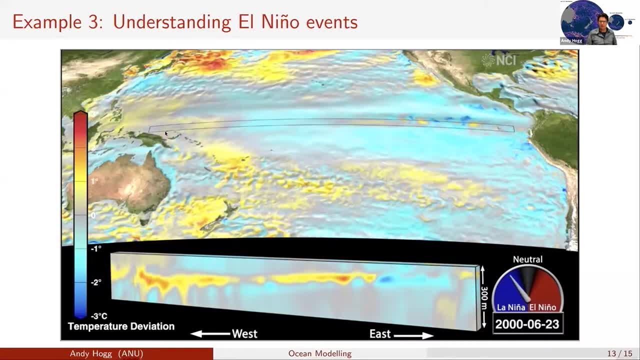 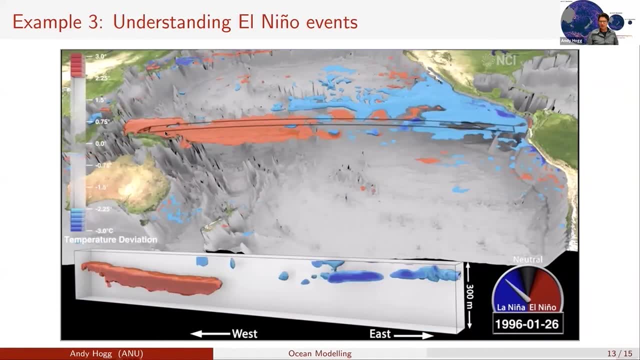 the normal climate, the normal wetter climate that we experience in the Western Pacific. so we jump jump now to a different frame, which is: this is a little bit of an attempt to show how these things are happening in three dimensions. so we're now plotting the temperature anomalies. 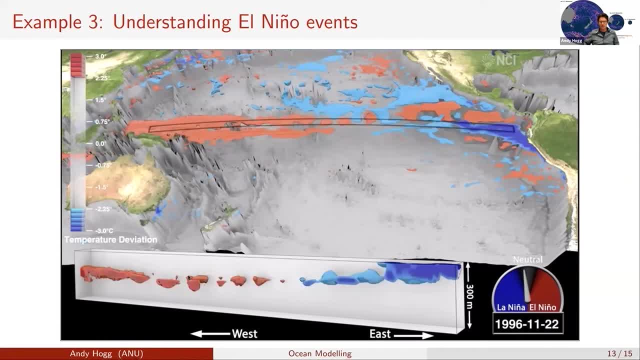 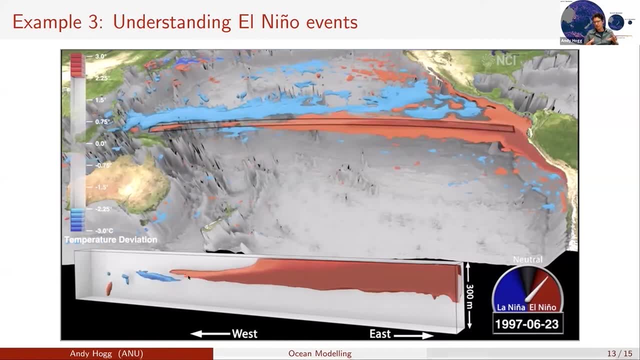 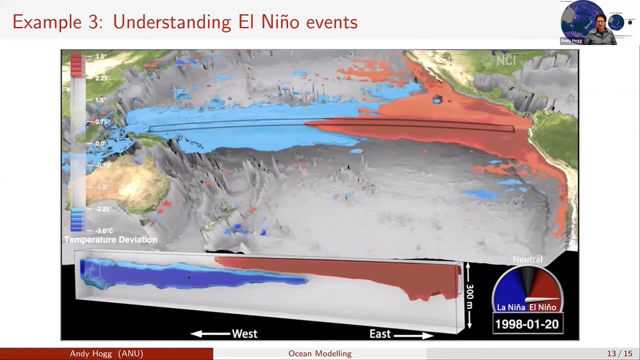 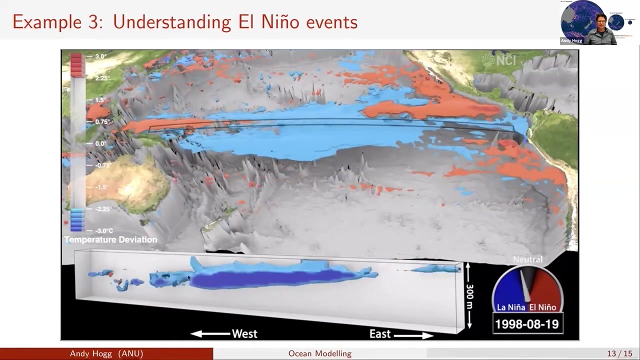 as a volume. and again we move into 1997 and you can see these warm anomalies flooding all the way across. so this is a huge amount of warm water which floods across to the Eastern Pacific and and then floods back once the El Nino ends in mid-1998 and turns back into a La Nina. so ocean models particularly higher. 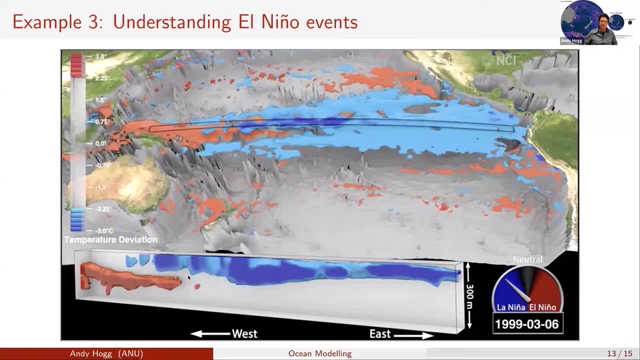 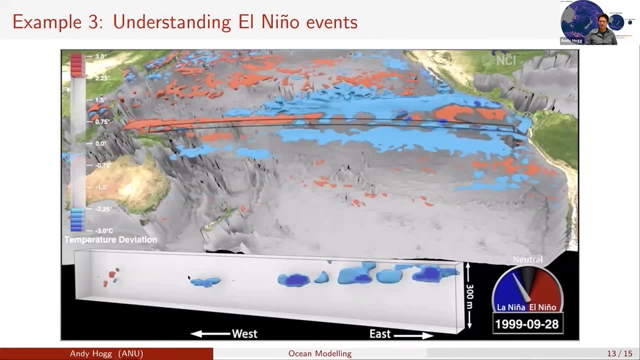 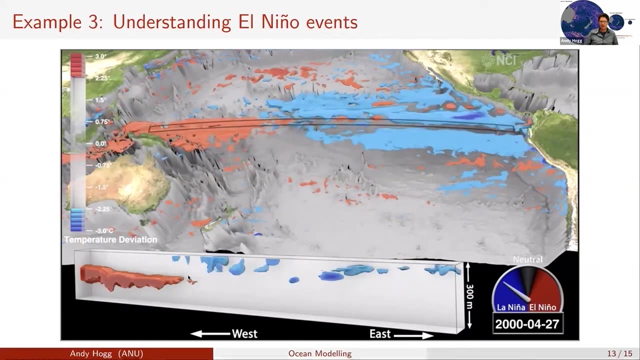 resolution. ocean models that can resolve all these processes are very useful for understanding how these events develop and for understanding the sensitivity of these events to future change, and one of the big questions that the climate centre that I'm a part of is trying to answer is you know. 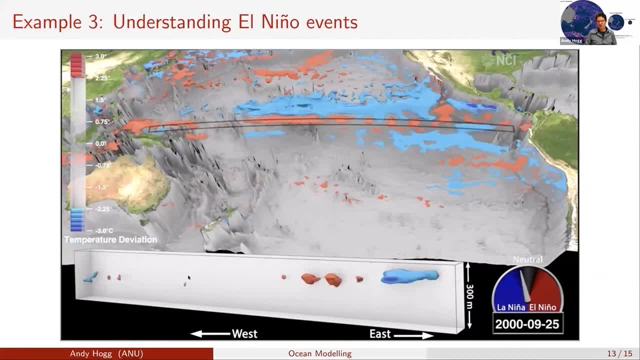 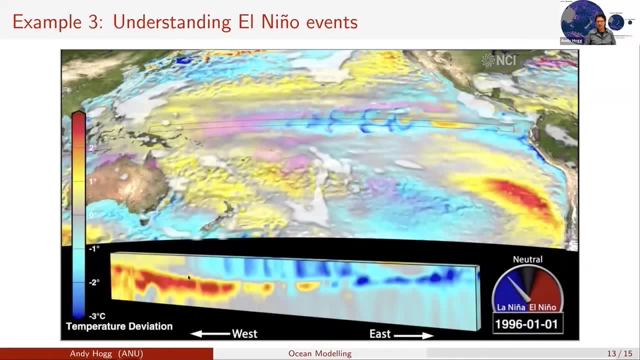 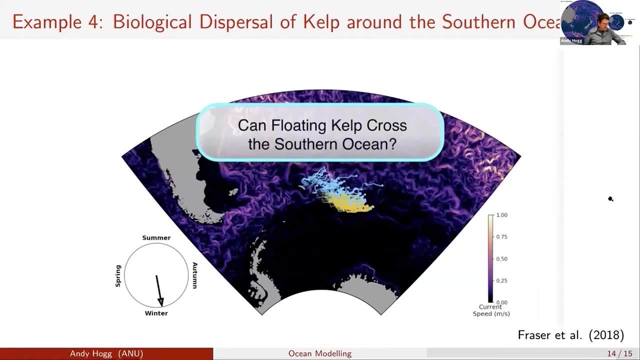 how do these El Nino events cause extreme climate conditions and how are these El Nino events going to respond to extreme climate conditions in the future? so I'm going to jump to my final example here and again, I'm going to show this example by way of an animation, and this is an animation we made when we released a paper on this topic, and 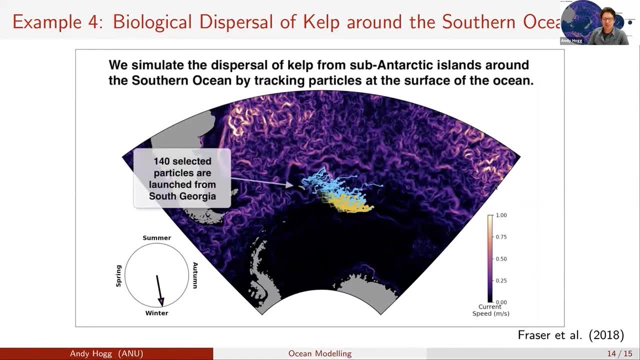 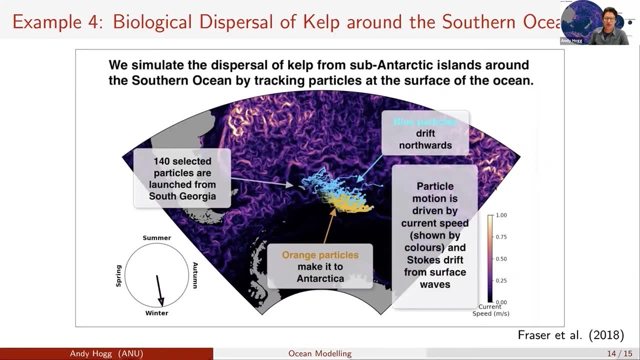 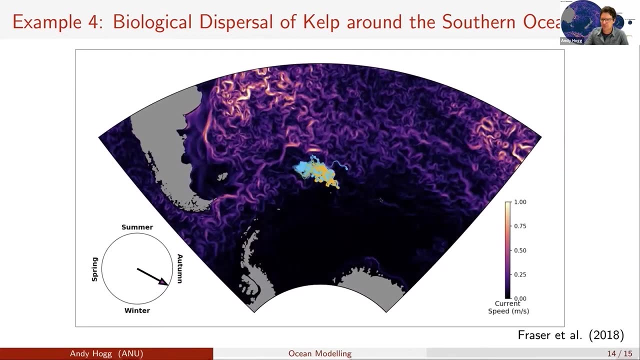 it was actually. this is actually quite an interdisciplinary project and it was motivated by a, a biologist friend of mine, who discovered- I'm just going to stop this one for a moment if I can- yes, I can. and my collaborator discovered- they discovered that on the beaches of West Antarctica. 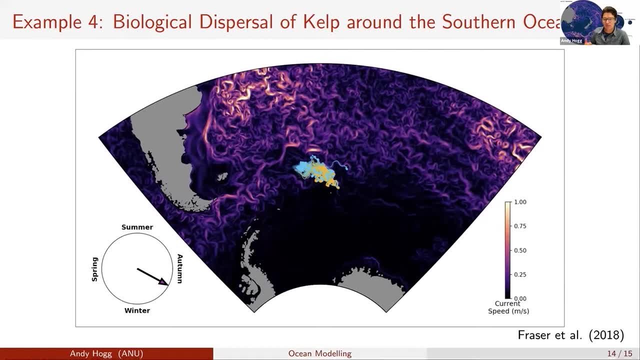 just here that, um, some kelp had been washed up on this beach, and this kelp is, um the vilia kelp, which grows on sub-antarctic islands, that only grows around islands that are around 60 degrees of latitude, and the common wisdom amongst the biologists is this kelp could not make it south of 60 degrees. 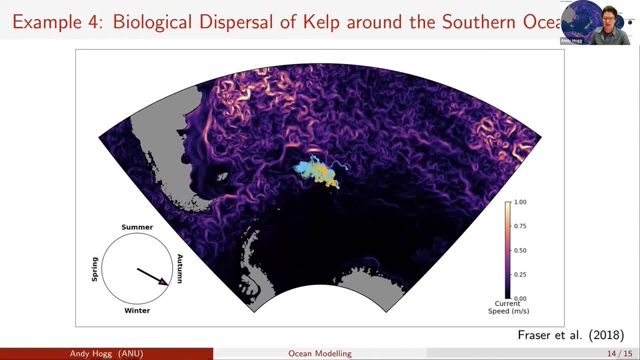 south. the physical system would stop them, and this was. this was almost folklore in the biology community. and um yet she discovered that some of this kelp had been washed up. it hadn't come by boat. it must have floated on the surface of the ocean. how could it possibly get there? and 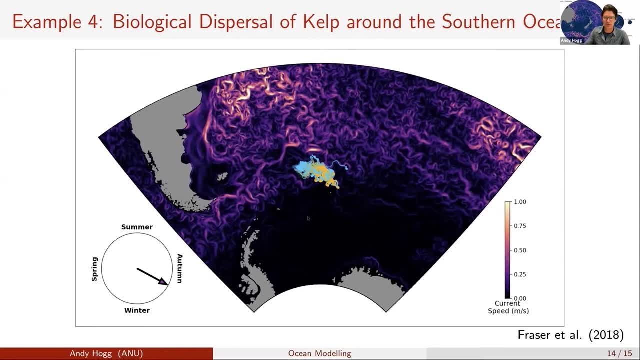 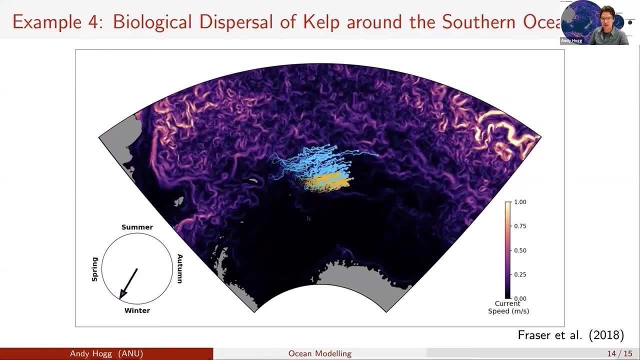 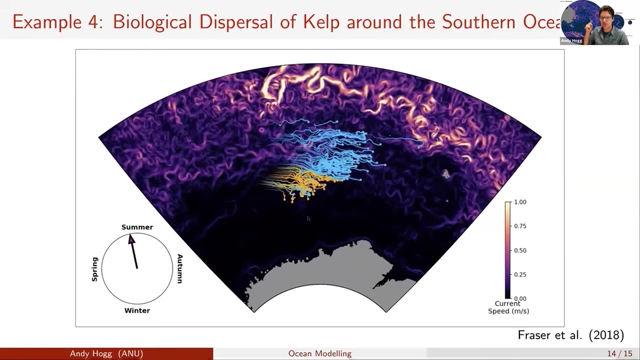 so she turned to us to to answer this question and the answer- the physical answer to this was actually, uh, that it's a combination of these small scale eddies that you can see rushing around here and the um, the poleward migration of some of these parcels during storm events. 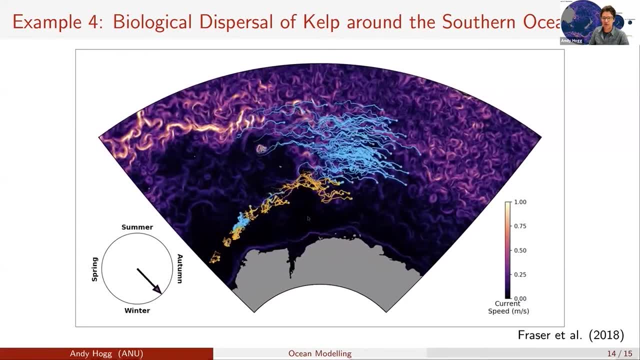 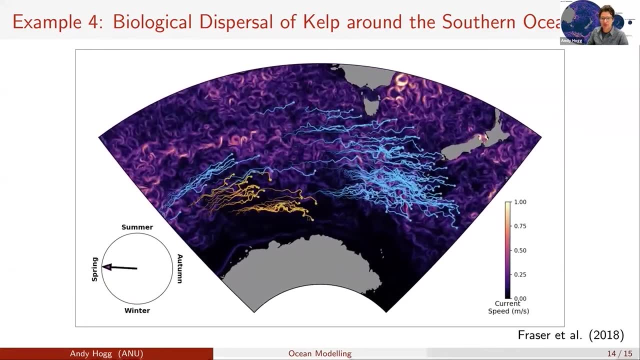 so what you're seeing here is the trajectories of a whole lot of kelp that we seeded our model with. so we put some kelp into our model and then we decided to see where they went, and the fact is, most of them follow this blue trajectory. 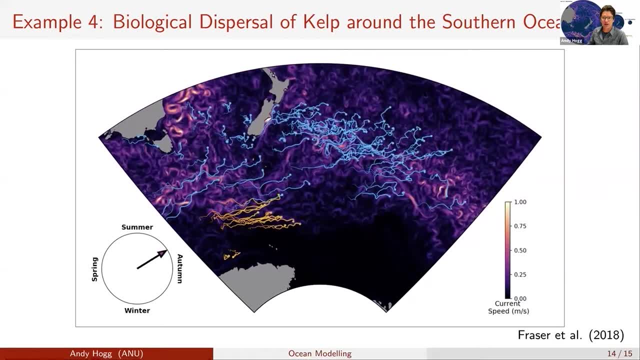 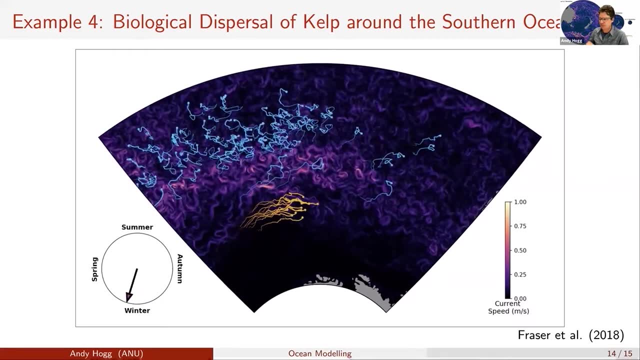 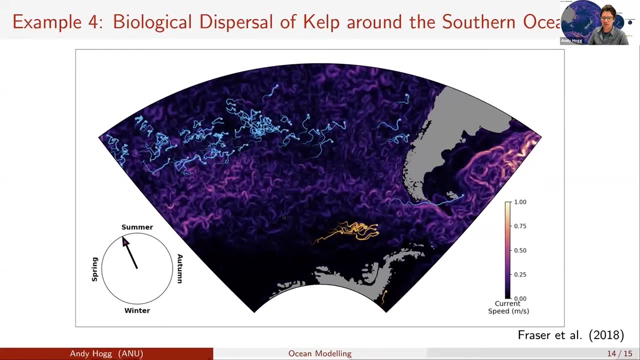 trajectory and end up going to the north and they end up in the subtropical ocean. but these little orange ones down here, they didn't go to the north, they were driven south by a storm or a particular eddy event. and this was the first time you could. you could actually show that. 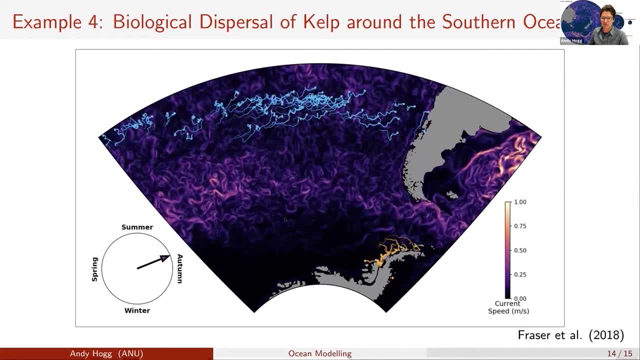 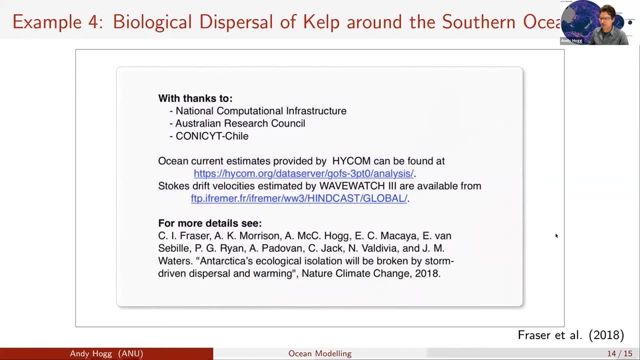 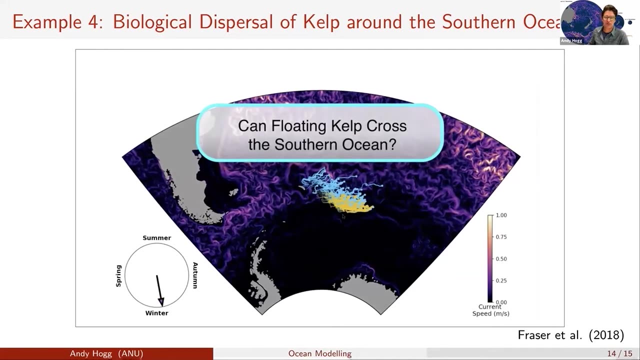 these kelp uh could actually get to the beaches on west antarctica, uh, via the pathway that we were, that we were talking about. so i'm just gonna- um, i'm just gonna play that one again, because there are a few things uh there that i that i didn't get to. so all the kelp in this particular animation. 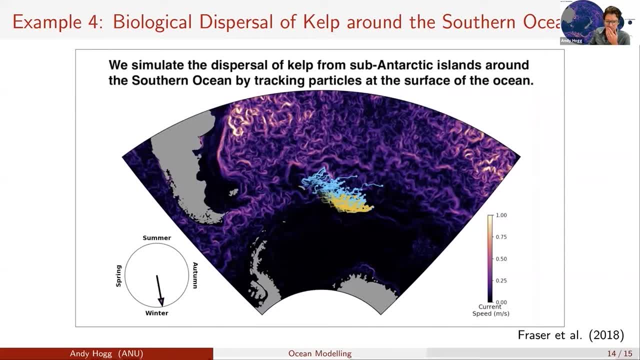 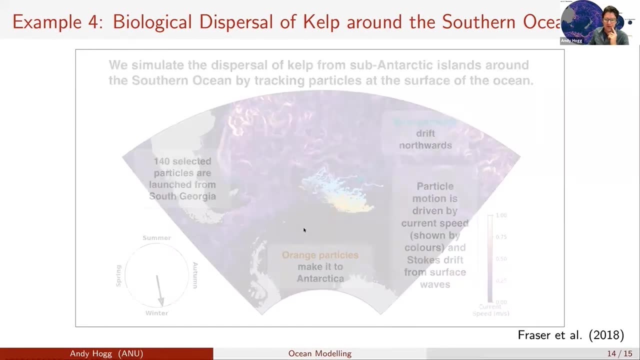 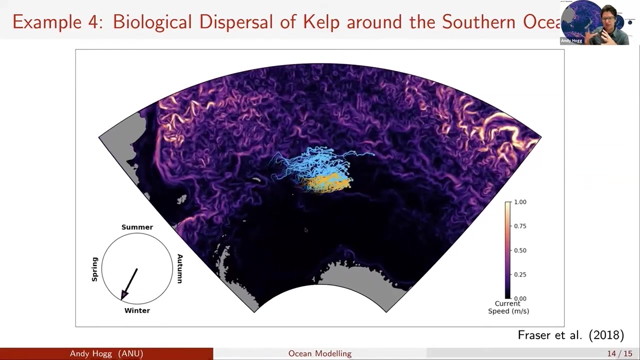 are released from south georgia, um, and you'll notice that all of these 140 selected kelps only through drake passage here. most of the rest went north and about 10 of it made it made to antarctica and uh, so what you can see is that initially these kelp all start out together and they very slowly 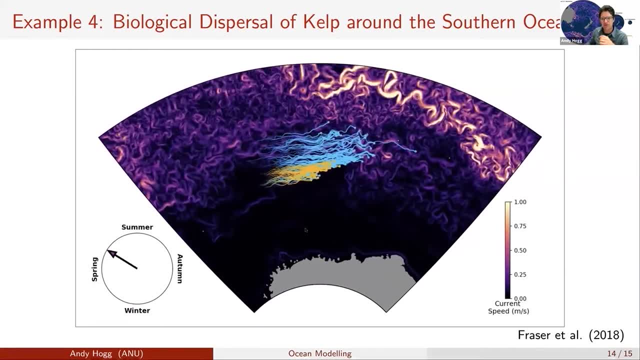 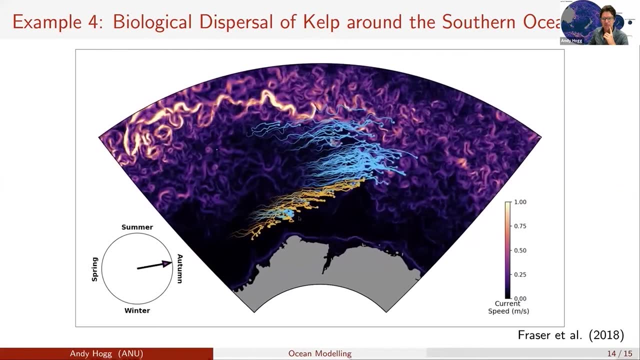 diverge. a lot of their motion is coherent, but sometimes they diverge and you can see particularly some of them just get swept up in individual currents. but this they're still blue, mixed in with orange here. some of them made the beach quite early. they got stuck in. 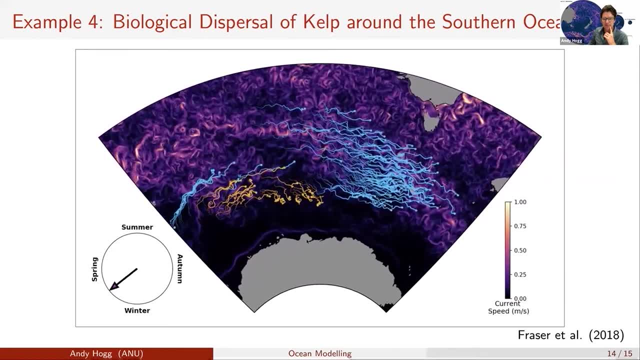 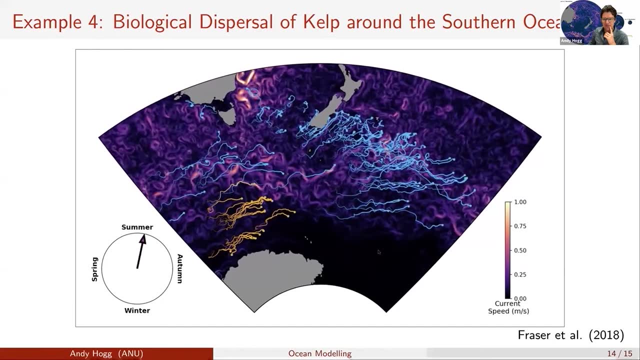 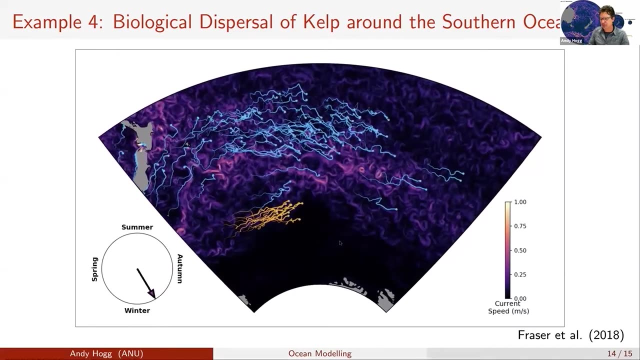 stuck in a the antarctic slope current and pulled around the other way, and some of them made it all the way around, uh, to west antarctic peninsula, so, um, so this this was a very interesting project to be involved in because it was fundamentally interdisciplinary. we we needed the high resolution modeling tools, but we also needed 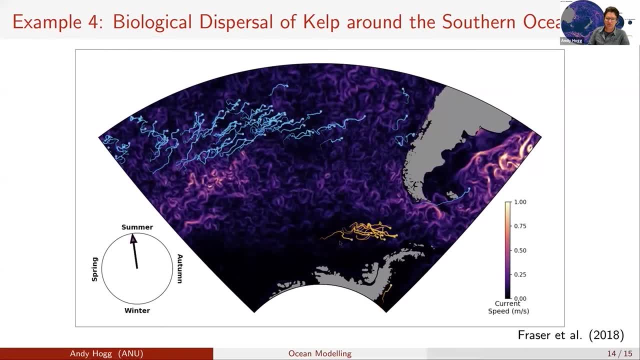 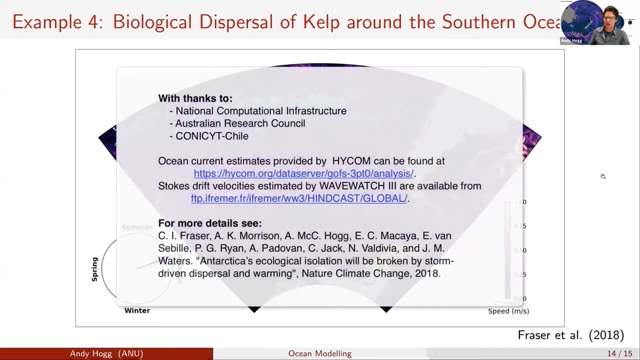 the genetic sequencing of kelp to discover where the kelp had come from. uh, and it's the sort of for this project we, we, uh, we like to get involved in. so i'm going to sum up there and that'll allow plenty of time for questions, but i just want to. 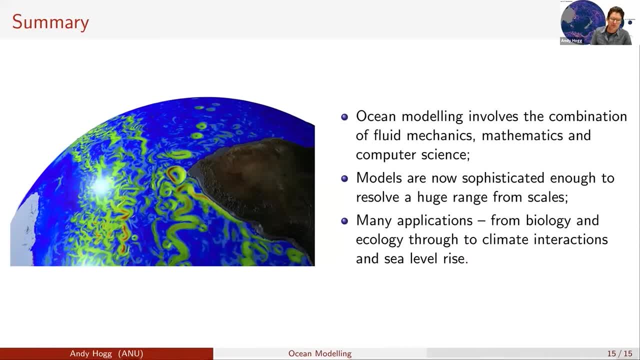 emphasize that ocean modeling is something that i i really enjoy. i i enjoy the fluid mechanics part of it. i really enjoy the maths and the computational science part of it, but i also enjoy the applications that we get out of ocean modeling, from from biology through to ecology. 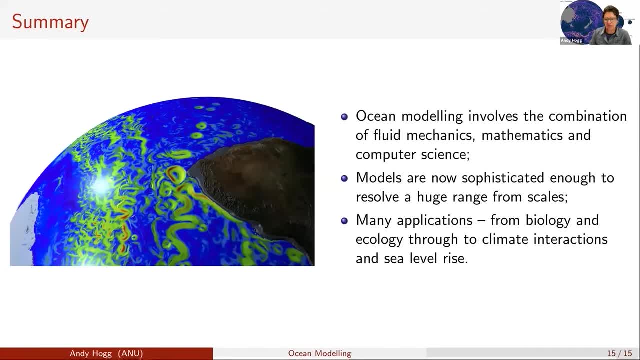 through to climate. it means that we can use fundamental physics and fundamental computer science and maths to understand problems that are really important to the real world, and that's one of the reasons why i continue to to work in this area. through my career, i've seen. i've seen models. 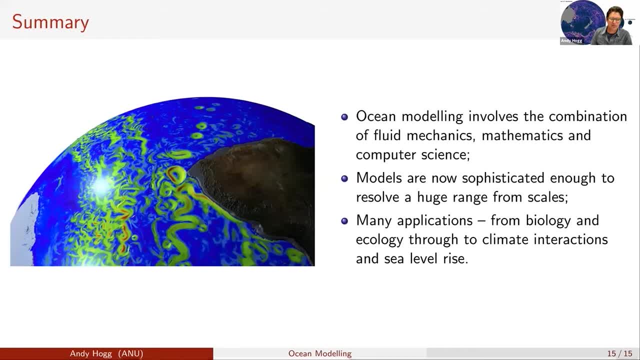 go from what i would call to be, you know, rudimentary models through to these, any resolving models that i'm showing on the left here, and when i started in this field, basically we couldn't, we couldn't simulate, uh, the ocean system at this scale with these sorts of. 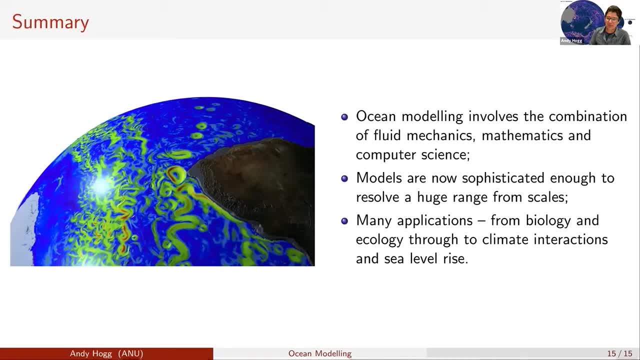 eddies. so it's been interesting to see how things develop and models are becoming more and more sophisticated and more and more able to resolve a huge range of scales, which is which i look forward to seeing how that continues to develop. so i think i'm going to stop there and i'd encourage 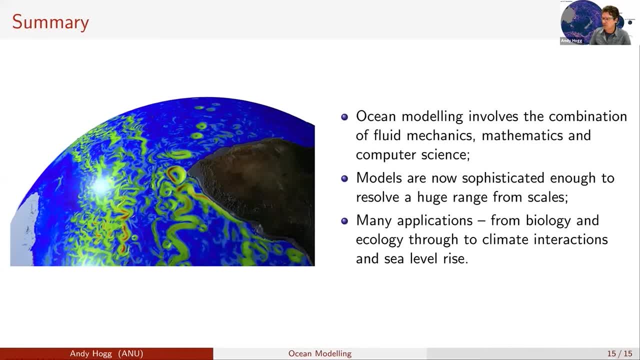 you to keep asking questions on the chat, and i'm going to get through them one by one, unless jay wants to jump in and suggest. suggest a way to proceed. please go ahead, andy. one by one is fine, okay, let's do that. so, um, i think what happens is when i click a question that i'd 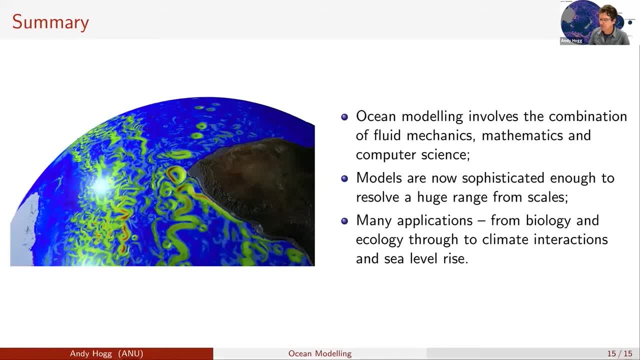 like to answer. um, the question should come up for you. is that correct, jay? people should be seeing this question here. yes, that's correct, okay. so this question is: why is the southern itcz, that is, the intertropical convergence zone, which is like the meteorological equator- why is? 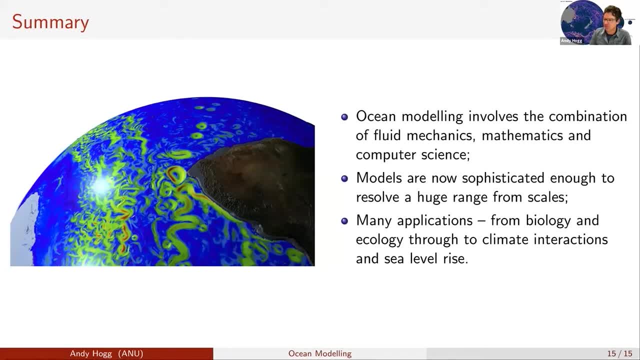 the southern weaker than the northern in terms of ocean atmosphere interaction, um and emphasizes the double. it's a tcz features, uh that occur in the pacific and atlantic, and so, in general, there's a. there's been a lot of work recently on on how, when you have one hemisphere which is warmer than 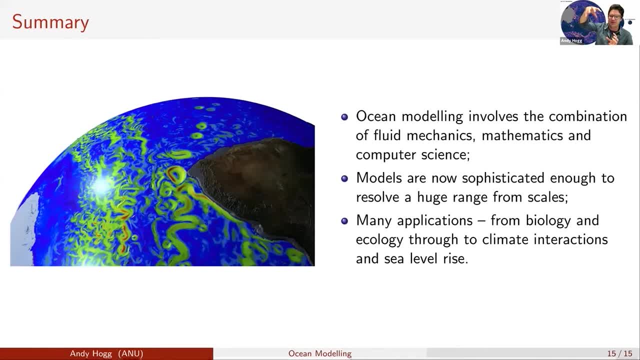 the other that can pull the itcz uh one way or the other, and so it turns out that um, the itcz which uh, um, which is roughly at the equator is, is further north at the moment than uh, than um, than it is to the south, and so that that is effectively because the northern hemisphere is warmer, and that is. 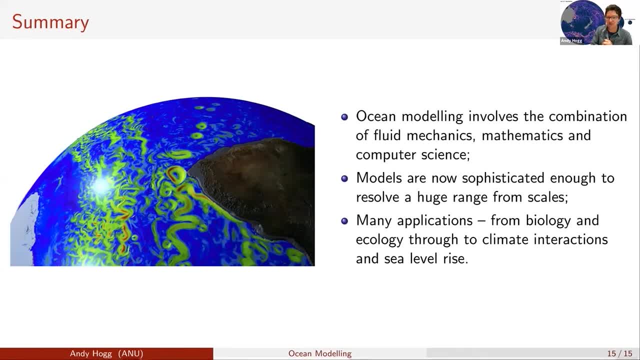 effectively because, if you like, there's more land in the northern hemisphere than there is in the eastern hemisphere and it's the northern hemisphere which, uh, helps to cool things off. um, feel free to post a follow-up if, um, if you, if you need. so i've been asked. please elaborate on. 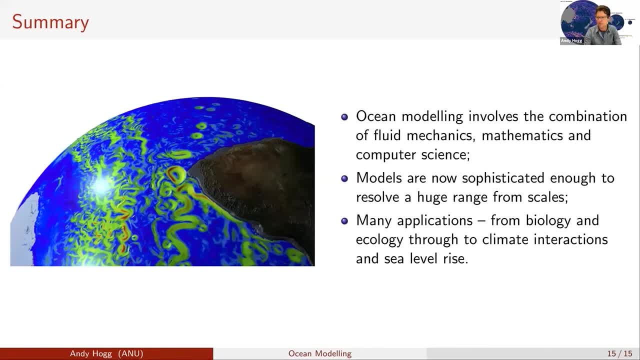 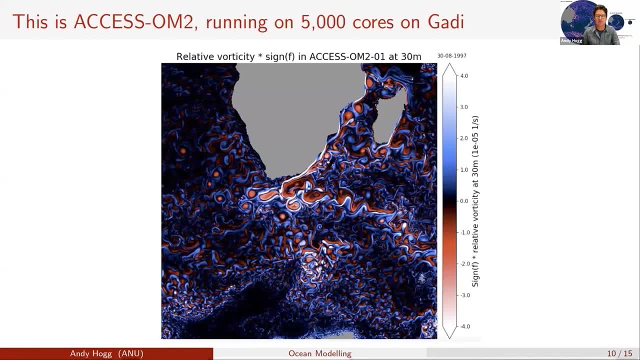 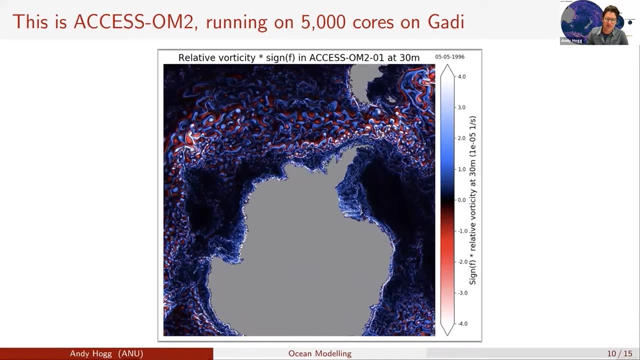 the characteristics of these patterns in the ocean, and this question came up when i was showing, um, my original- uh, potential relative vorticity movie. so, um, i'm going to go back to that and people can Wow, there is so many characteristic patterns going on here. 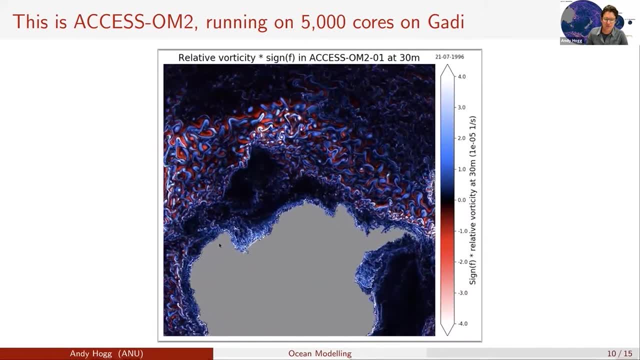 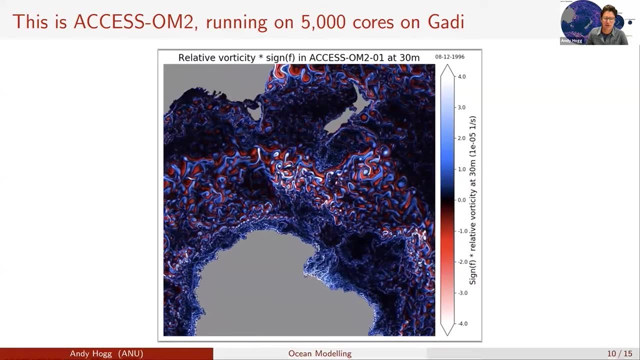 Close to Antarctica you can see really small-scale features beneath the seasonal sea ice and the formation of this Antarctic slope current which comes around here. This west-to-east current in the middle of the Southern Ocean is called the Antarctic Circumpolar Current. 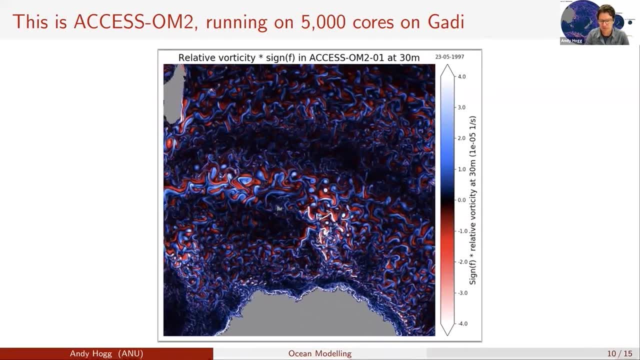 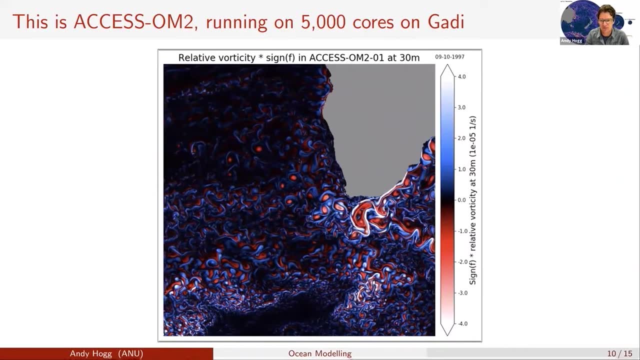 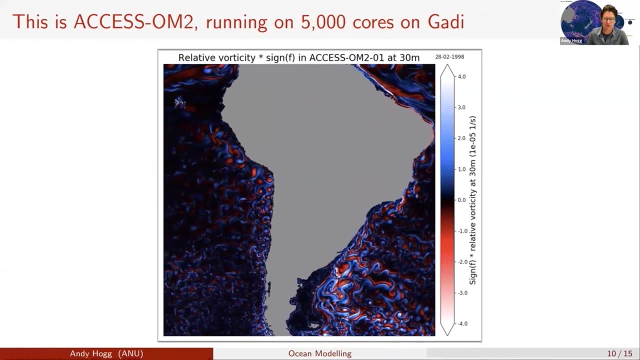 which is a sort of wind and buoyancy and topography-driven current. This is a western boundary current which is part of the subtropical gyre system in the Southern Indian Ocean and often you'll see these western boundary currents going poleward along the western boundary of an ocean basin. 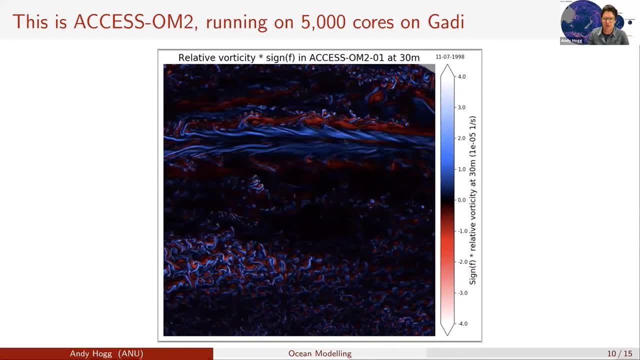 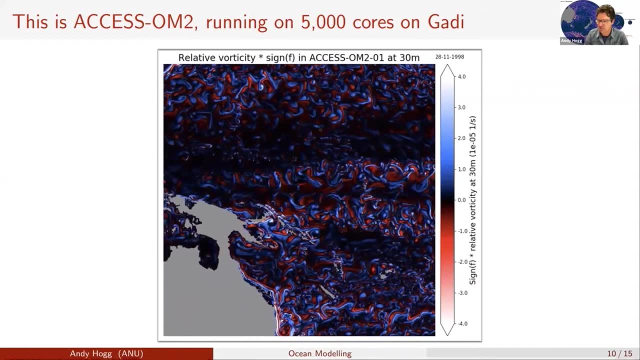 and you've got a lot of east-west currents right at the equator, causing tropical instability waves. There's just a huge number of processes going on here and I can elaborate a little bit on them, but I can't elaborate. I don't know too much. 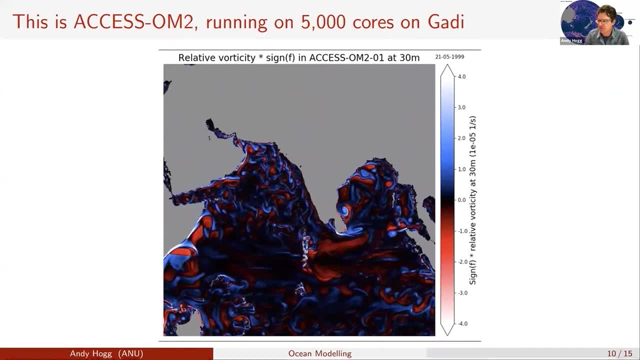 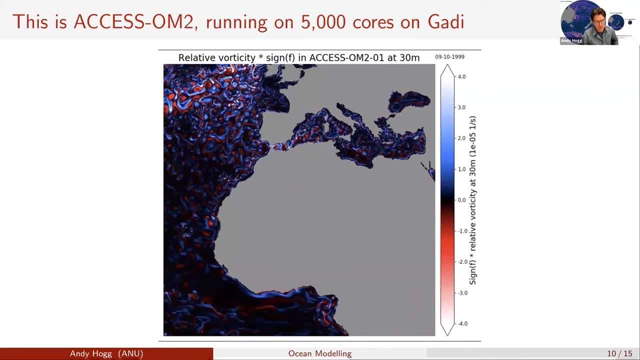 So the next question I'm going to look at is: what subgrid scale model do you use, if any? And the answer to that is yes, we use heaps of subgrid scale models, And for those of you who are doing engineering, 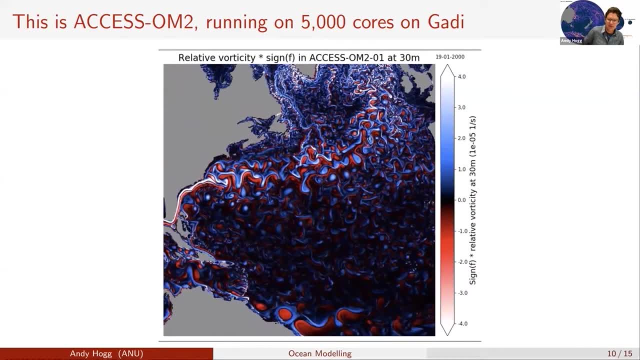 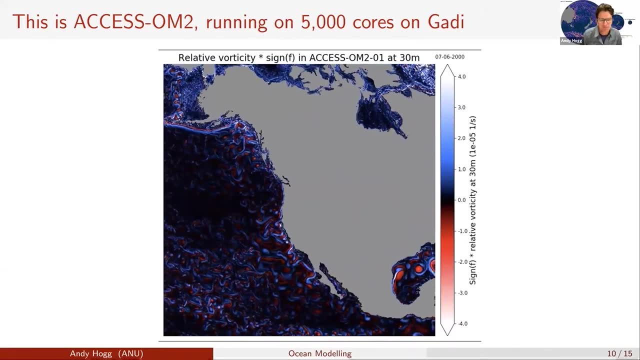 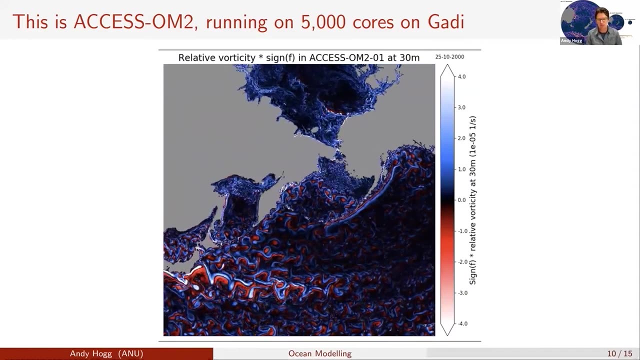 you're probably used to terms like direct numerical simulation and large eddy simulation or Reynolds average Navier-Stokes, And you know I would love to be able to use direct numerical simulation to simulate all these. Some of my one of my collaborators down at Uni of Melbourne. 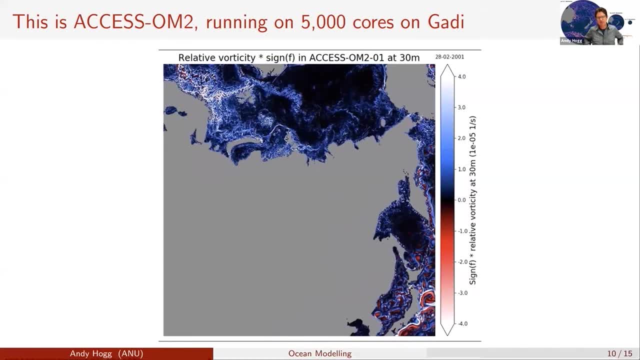 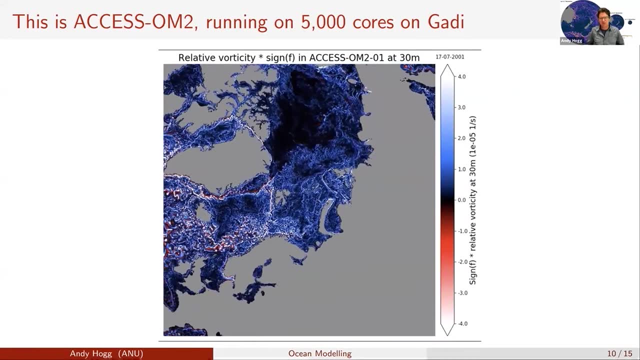 Bishat Gayan. he is an expert in this type of thing, And direct numerical simulation simulates all the scales that you can, but you can't possibly do that over the entire ocean, So you need all sorts of subgrid scale models. 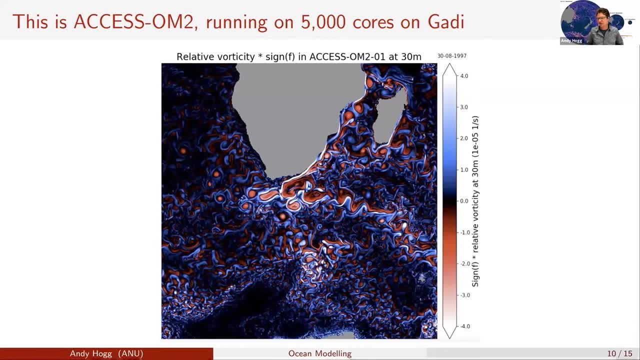 The types of ones we use include sub-MESA scale parametrizations. Sometimes we use a MESA scale eddy parametrization. We use we use different subgrid scale models for convection. These convective models are very poor, but they're things that we're trying to improve. 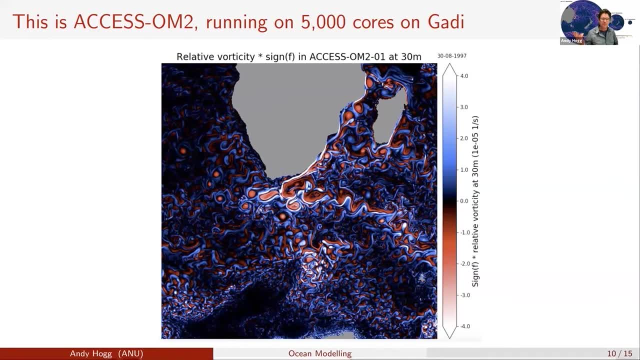 We use subgrid scale models to understand how energy and momentum comes from the atmosphere into the ocean, how gases are exchanged across the ocean atmosphere into interface, And so I'd say, in one of these ocean models you're normally implementing something like 10 subgrid scale models to deal with. 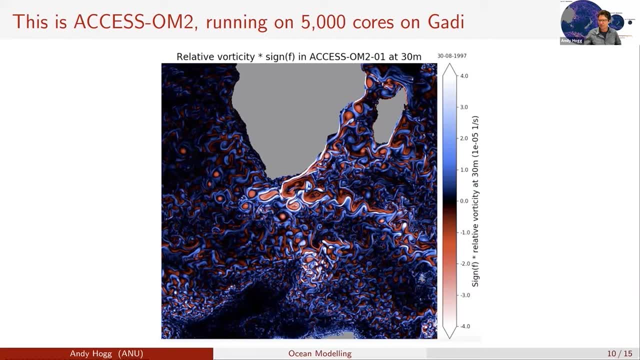 a whole lot of processes that you just can't resolve. What have I? what else have I got here? Let's answer this one: How do atmosphere and climate models compared to ocean models? That question was clarified, so I'll put both of them up. 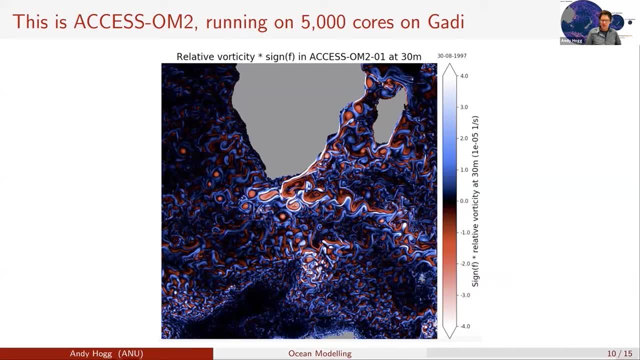 Please give an overview comment. So atmosphere models, you know, ocean models and ocean models really have the same fundamental underpinnings in that they really depend on fluid mechanics. The big differences are in the ocean. we have to track salinity and temperature. 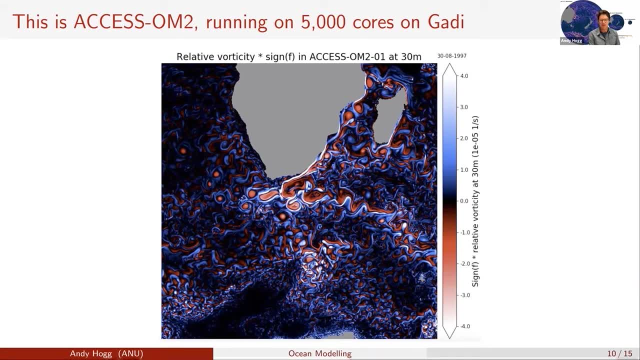 The flow of the ocean occurs on very small scales and takes a long time to adjust. The ocean is much the atmosphere, sorry- is much more compressible. Instead of salinity and temperature, we're interested in temperature and moisture. We really care about microscale physics in clouds, and we have atmospheric currents- a much larger scale. 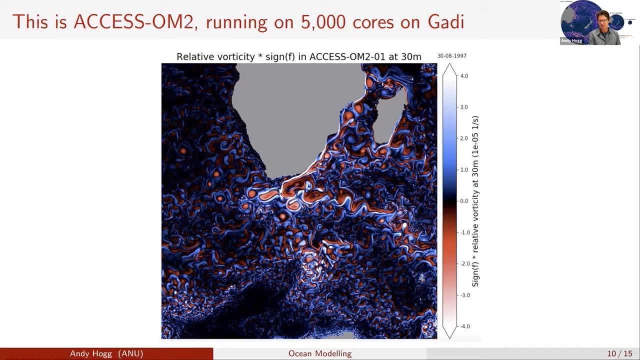 Wind is a much larger scale, but they establish themselves much more quickly. So you know it's. it's the same sort of principle. I can go to an atmospheric modeler and we can talk the same language. What I can't do is turn around and use my model for the ocean. 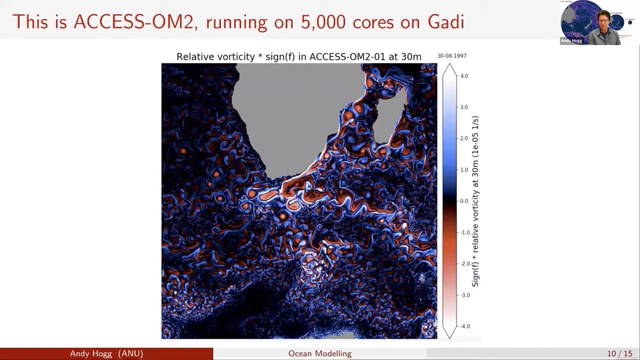 Exactly To model the atmosphere In a climate model. well, in a climate model, you actually need everything. You need the ocean, you need the atmosphere, you need the sea ice, you need the land surface scheme. So a climate model is much more complicated and a big part of a climate model is actually integrating all these different models together to produce a coherent simulation. 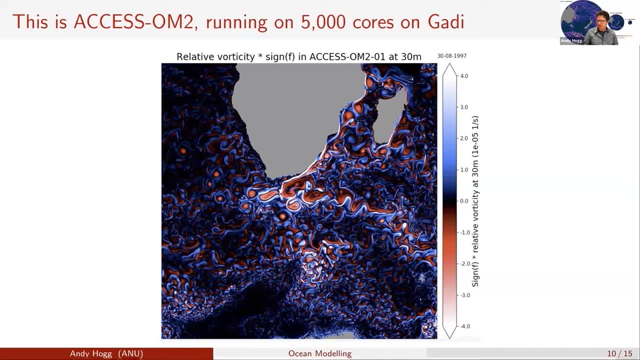 Okay, Let me answer this one, which is about whether an ocean model can be used to simulate real time events such as tropical cyclones, And the answer is yes And well, we can't simulate the atmospheric component of a tropical cyclone. 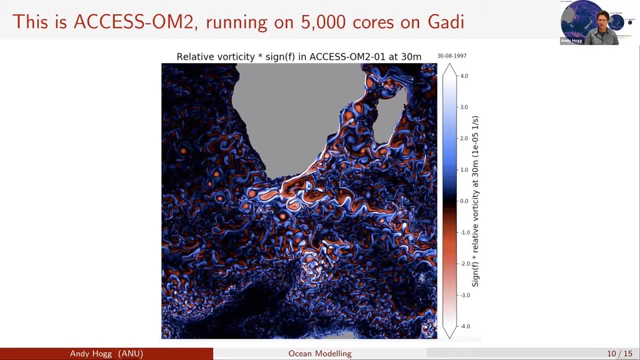 but we can simulate the ocean component, And so the way we would do that is is we would use a combination of a model like this, and we would use it in combination with a technique called data assimilation, And data assimilation is basically a fancy word for getting the initial condition of an ocean. 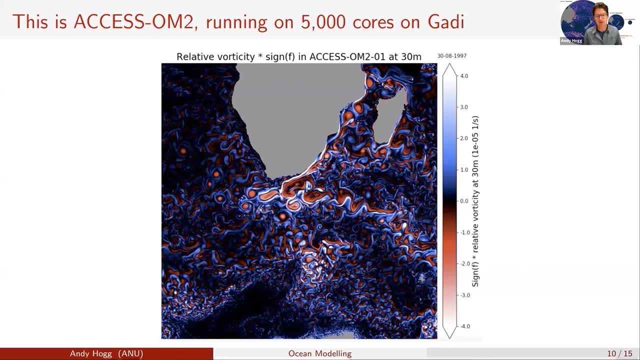 initial condition of the ocean, So an initial state, if you like, And that means that we can use all the satellites and observations that are available to initialize the model to a state which is very close to today, And then you can move forward and predict a near term event. 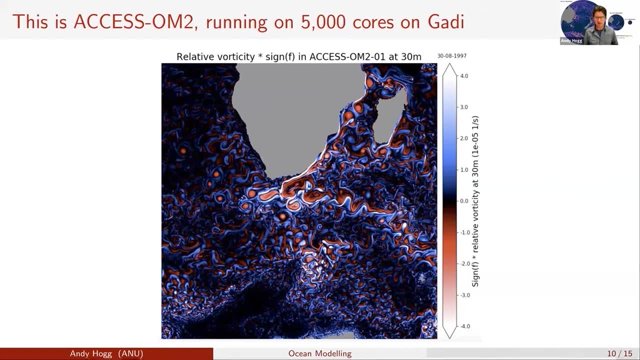 Okay, And that's what numerical weather prediction does, And that's what I would call ocean state forecasting, And ocean state forecasting in Australia is done by the Bureau of Meteorology. In your country, it's probably done by a bureau as well. 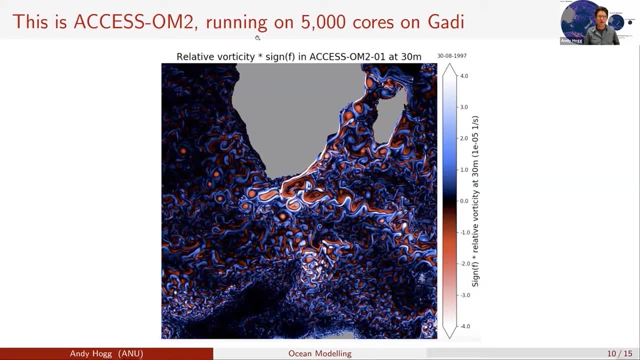 some sort of meteorological bureau, And the development of this ACCESS RM2 model is really to get the next generation ocean forecasting model. Ocean forecasting is an operational forecasting, Which means that when they run the model it has to work. When I run a model, I like to play games with it and find out interesting things. 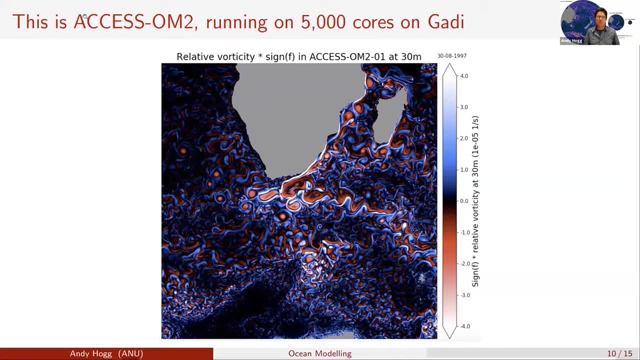 So The way we do this is- me and my group have been working on this model for the last few years and in the future. the operational agencies are picking up this model. In fact, they're already doing it, And maybe by next year they'll be using this model for the operational forecasts and 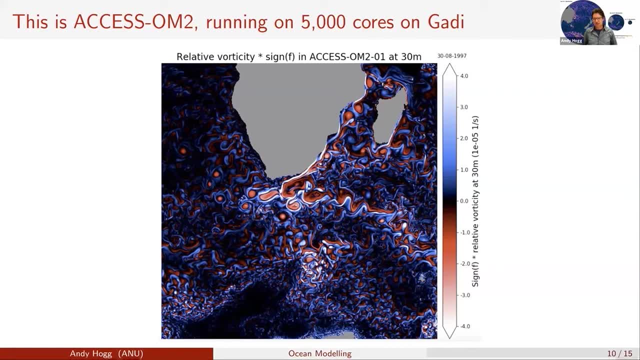 they'll use that another four or five years, by which stage the researchers will have moved on to another model. in fact, we're already moving on to another model um to use. so so thank you for that question, um. so let's answer another question. what do you think will be the global temperature means sea level. 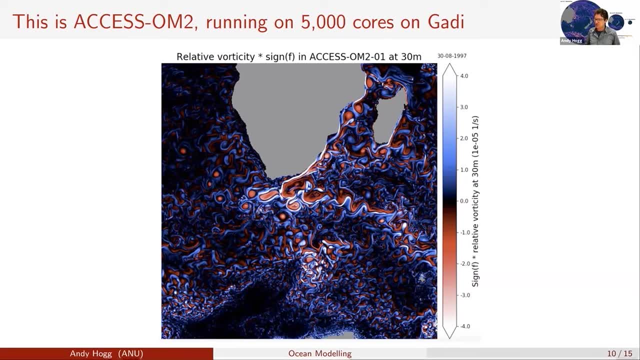 and speed of currents on average after, let's say, 15 to 20 years? very good question. um, global temperature will be a degree higher? uh, maybe only 0.6 of a degree, but i think it'll go up. sea level will go up, that's generally. sea level will go up everywhere. but 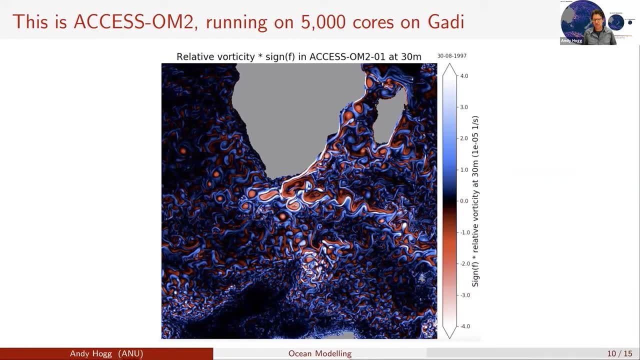 it'll go up faster in some places than others. um, i hate to say it, but the the western pacific region is probably going to cop a lot of the sea level rise and it's probably least equipped to deal with it. and so that's. you know, it's a big concern to many of us living in this region. 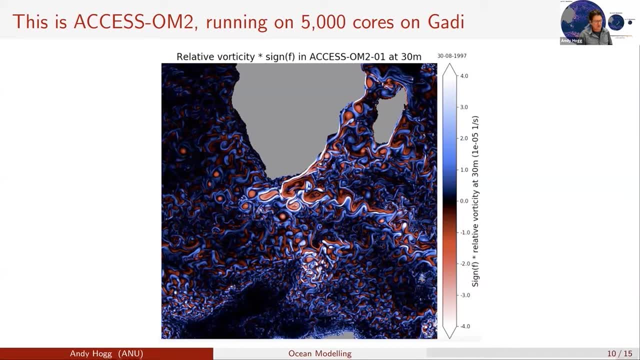 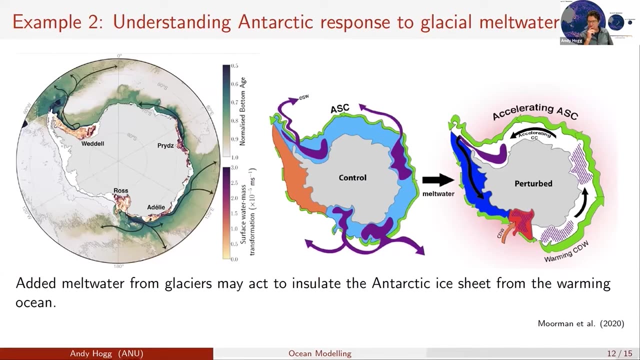 so there's a big uncertainty as to how big that sea level rise will be, and we're working to reduce that uncertainty by better understanding, um, things like, uh, what's going on around the fringes of antarctica and what the antarctic contribution will be to global sea level rise, uh, speed of. 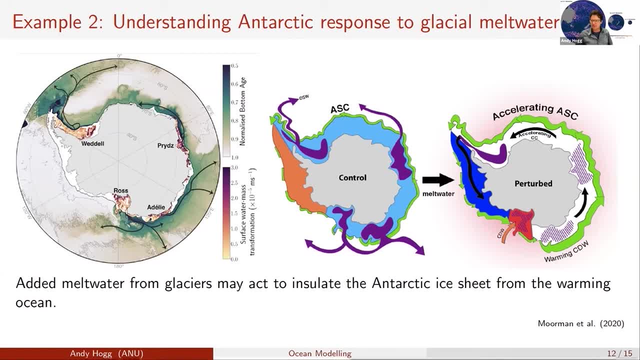 currents on average. they will change a little bit, but that's much more difficult to predict than than the actual global temperature. a very good question here: how do we validate this ocean model with empirical data from the actual, from the actual oceans and and that's a really good point. so one way we do that is actually: 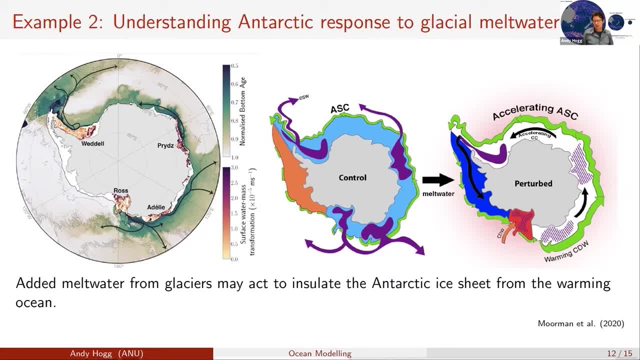 through this data assimilation process that i was talking about before, and we've recently been through this exercise with our model and the data assimilation people picked up that well, look you, you in our model we're developing some subsurface biases in the ocean, in the tropical pacific. 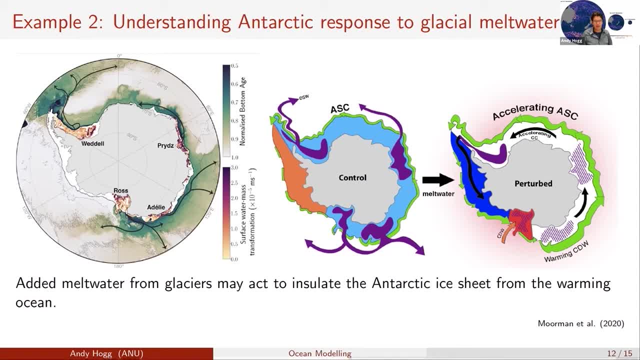 and these were biases that we hadn't expected to see, and they revealed a problem with our model that we can now go away and fix, and we've now identified the problem and we're in the process of improving that aspect of our simulation, and so that's, that's a key, key thing. uh, we do have some. 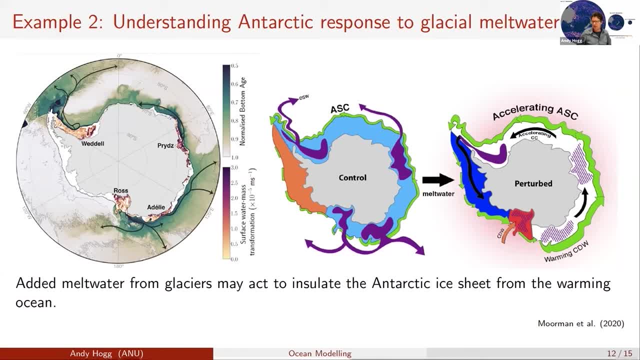 standard metrics that we use. um, uh, and i'll refer you to a paper on. you know, when we release the actually would, there's about 20 or 30 figures comparing the model output with uh with with the best that we can observe. so good question. um missed the part where you explained. 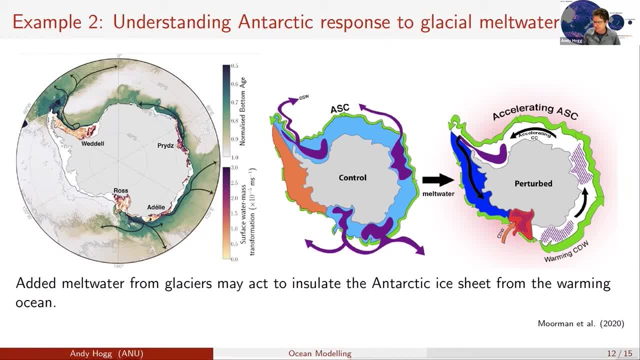 about vorticity. don't apologize for that. you did i, uh, sorry, i'll put this up. uh, you did miss the part where i explained about vorticity, because i didn't really explain it very well. so, truth be told, vorticity is the curl of the velocity and we care about that in the ocean because, if you 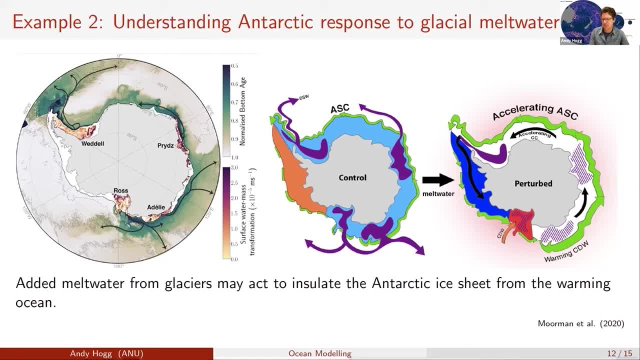 go through about 10 pages of maths, you can demonstrate that under some situations vorticity is a nicely conserved quantity, but it's a mathematically abstract um. so i decided that in a talk that was so short i probably couldn't- um, i couldn't do it justice. 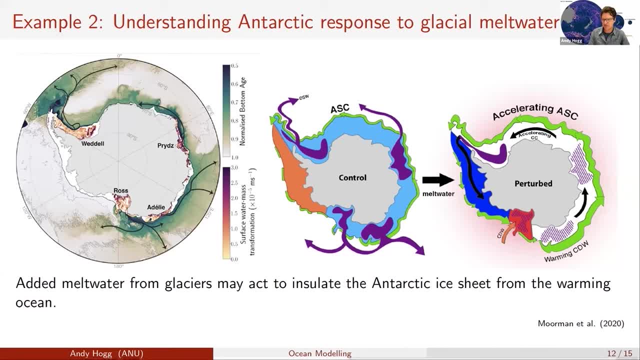 but if you, if you are more interested in this, you can look up something called urtel's potential vorticity and you'll find some, some really interesting mathematics behind how vorticity works. can we get live data to model real-time systems? um, that is a question which i 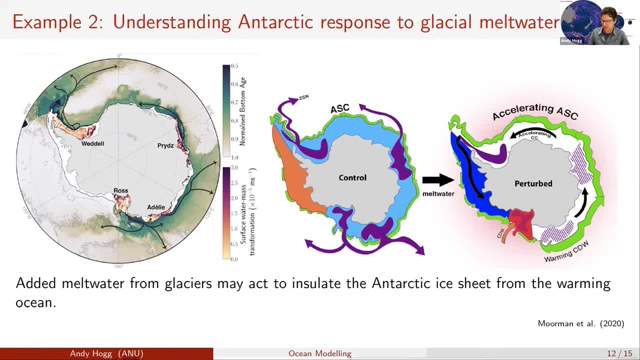 think i've already answered, thanks to data assimilation and ocean state forecasting. um, this is a question which, uh, is again about the validation against empirical data and um, uh, it's actually more specific from the last question. it wants to ask for specific parameters. we can measure, so we can. we can measure sea surface height really well. 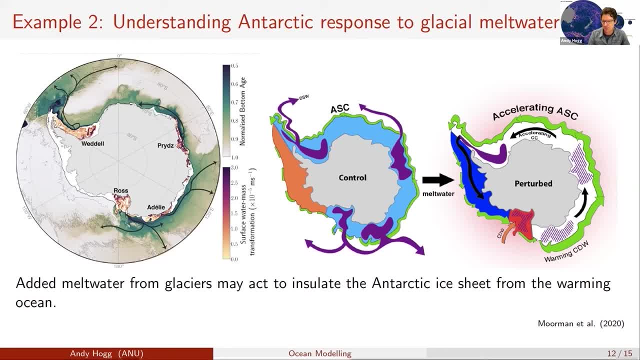 from satellite and um. therefore, we can measure the variability of sea surface height, and so that gives us an idea of how dynamic the ocean is, and that's what we're going to talk about in the next um part of the presentation. so if there's some issues with that, i'm going to go back to the 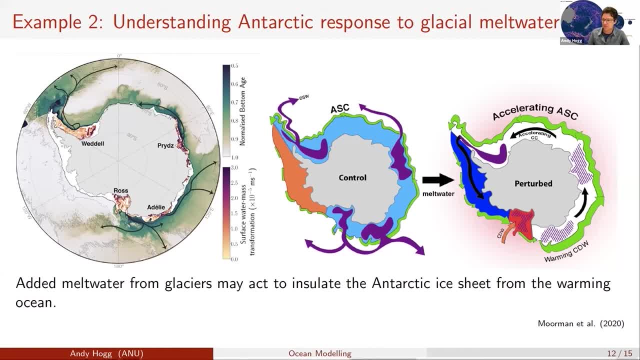 slide and i'll get it back to you, and if there's any more than that now there, you can have the presentation. i'm going to be a little bit longer and i'll show it on the other side so we can know. we've got a lot of data here as well, and that's one of the key things we validated. 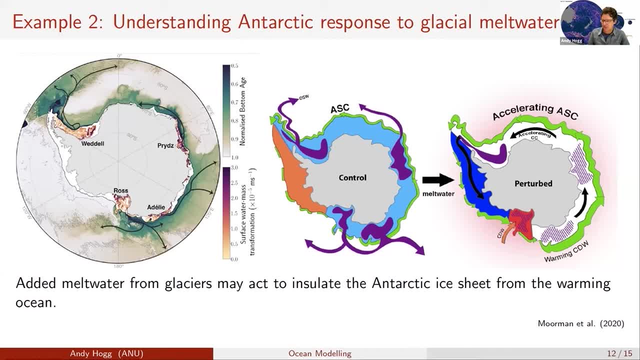 that's one of the key things. we validated this and found it comes comes up fairly well. um, we can model the mean flow in the current systems less well. we can model the sea surface temperature quite well. we can observe the sea surface temperature quite well, but only at the 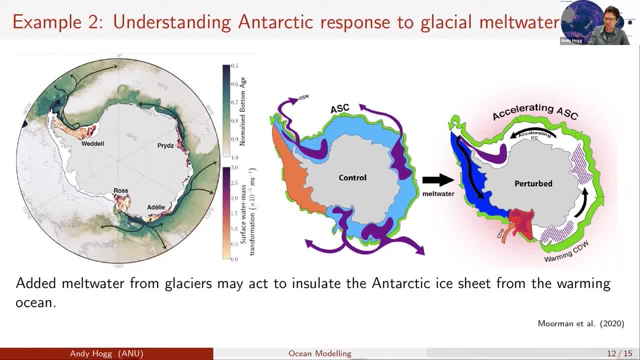 very, very, very surface, so that's very hard to validate against. and there's a lot of robots out in the ocean and and ship cruisers that are looking at salinity and temperature distribution within the ocean and those can be very, very easy to model. so they're different and we do have a lot. 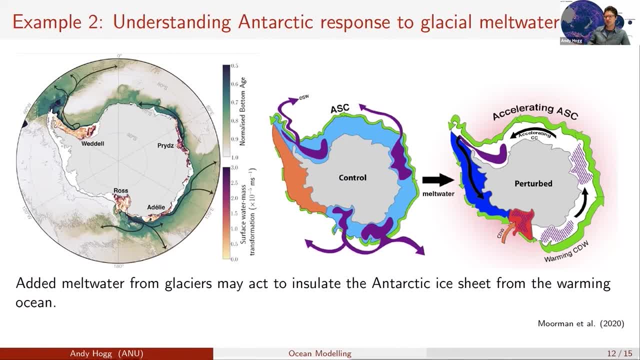 salinity. you know, salinity and temperature is moved around by these ocean currents, and so that's also something that we, that we look at a lot. okay, let me see. a couple of these are comments. here's one from left field: can we use the modeling to understand the Bermuda Triangle fluid mechanics and is 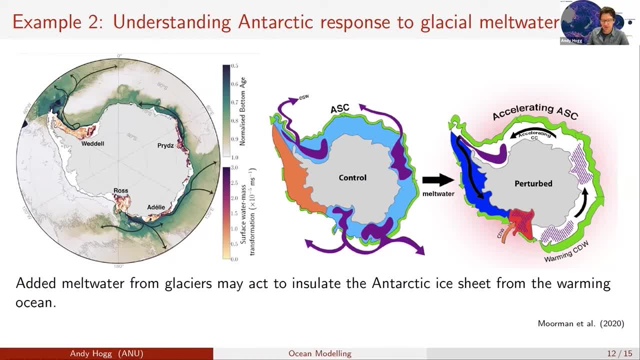 there scientific explanation, not that I'm aware of there's. there is nothing particular there that is going on in the ocean. you are welcome. all the data I use from our model is actually available publicly on the thread server at NCI here, and so you could actually download a ocean model of the Bermuda Triangle. 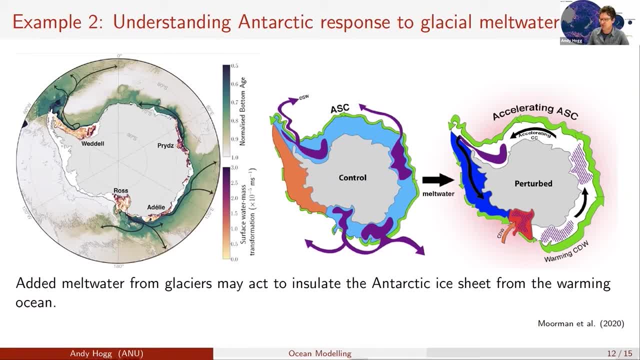 area and and have a look yourself. pretty sure there's nothing going on there. how am I going, Jay? why don't I take this one, which I haven't read yet, but I'll read it as we go. will global ocean level rise as a result of molten glaciers affect all these simulations? if yes, will? 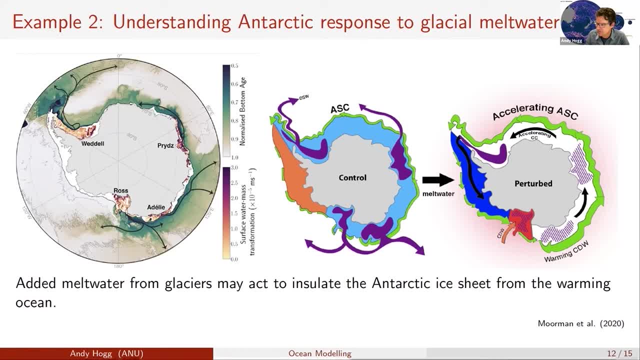 it be difficult task to include the melting glaciers as an additional factor. modeling these changes are different, and is this difficulty in modeling the reason why policymakers are procrastinating to take any concrete actions, given the adverse effects of global warming? personal view is that so, so let's deal. 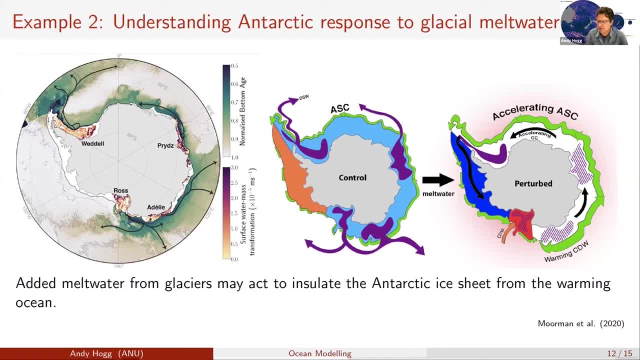 with this in order. global ocean level rise will will occur as a result of melting glaciers, and that's an important uncertainty that we really want to get to grips with. so we're going to be working on that a lot. global sea level rise also occurs just because the oceans warming projects here and there, else maybe go. we're really not going to split up quite that. why is that going to continue and go up to SCRAAF- a difference between global levels, but global centers will occur only- and this menstruatry during the day, and eventually the state of Korea, never a large nimbus. 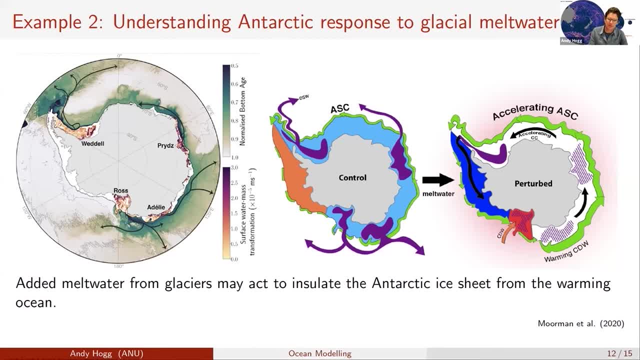 because warmer water takes slightly more volume, And so so far, most of the sea level rise that we've experienced has been more through warming than it has been through melting glaciers. So that's an important point. It's very easy to model the thermal expansion of seawater. 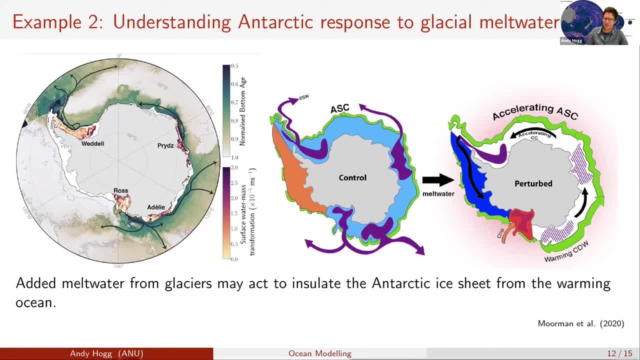 and it's very easy to understand how sea level will rise in response to global warming. This has been obvious for a long time and it is not the reason why the policymakers are procrastinating. The additional warming sea level rise from melting glaciers is more difficult to model, but again, 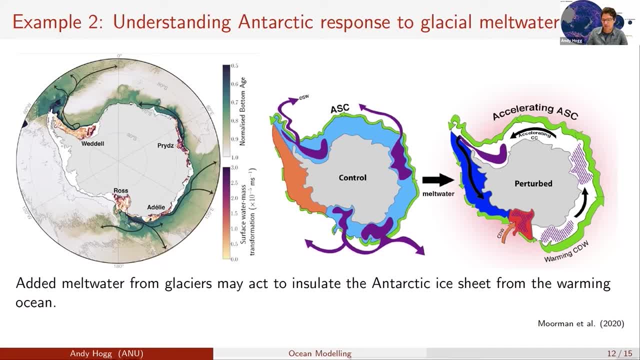 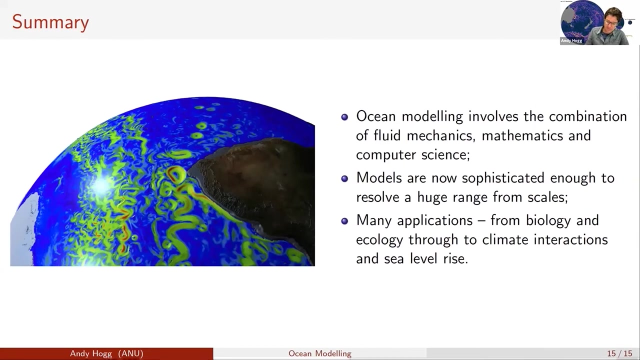 I don't think that's the excuse for procrastination. The excuse for procrastination is really just that it's difficult to get people to change the way they do things And I think you know there's a lot of vested interests in various systems. 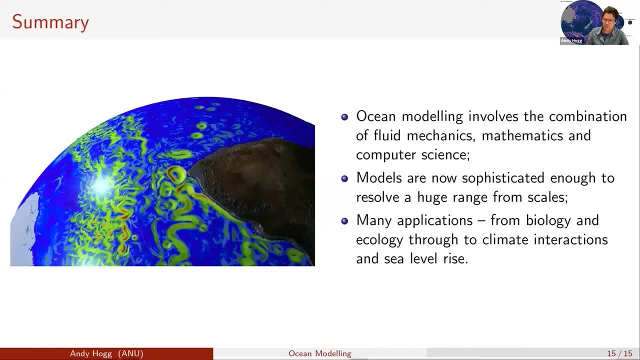 I think we're seeing change. We're seeing change in many countries at the moment. We're seeing the adoption of renewable energy in large scale, electric vehicles. we're seeing, and I think you'll find that once these energy systems change, they'll change really quickly. 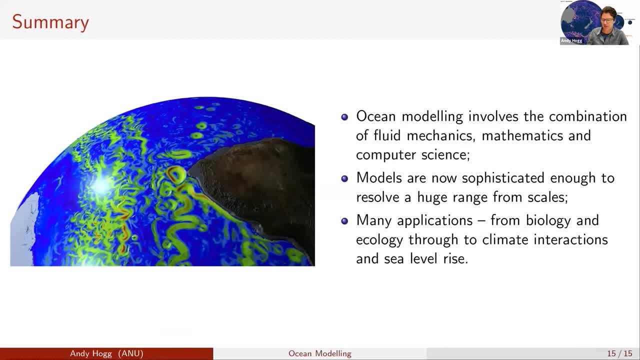 And I have actually have a lot of hope for, for how this sector is going to cope with this in the future. So one last question if I've got time, Jay, and that is: how much does the small scale dynamics affect the large scale circulation? 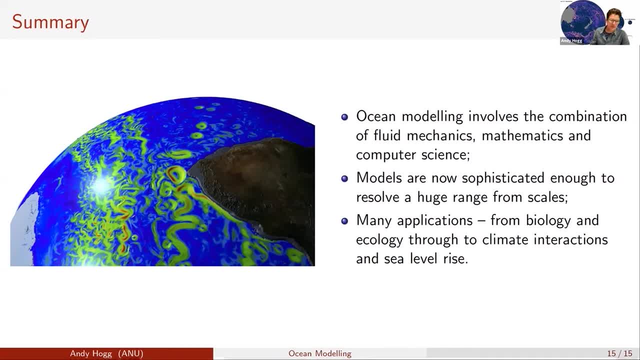 And the answer is that depends on which region you're in. In the Southern Ocean we've been making a case for some time that these small scale eddies you can see, you know they're not going to be able to move. 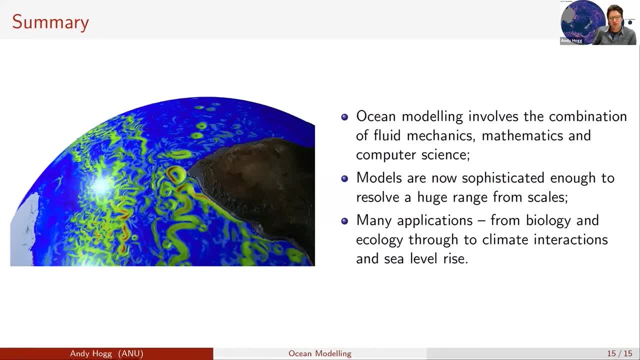 You can see here affect the large scale. We also know that small scale mixing and convection have a feedback onto the large scale ocean circulation. One of the problems we have is that the models that we use to represent these small scales are very expensive. 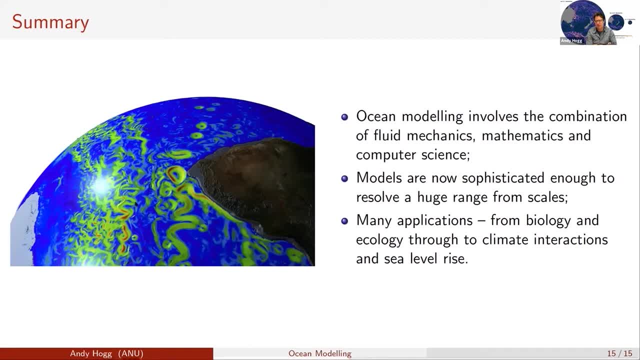 So it's very hard to answer that question in a way, in a way that you know, with with a modeling tool, because modeling both the slow large scale system at the same time as modeling the fast small scale things is very computationally expensive. 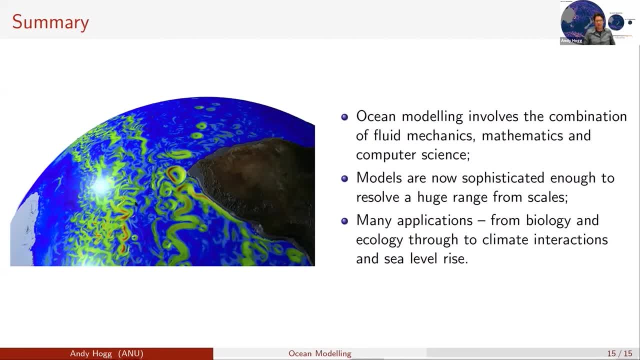 So it's very difficult to answer those questions with a single model simulation, But there are definitely many examples where the small scales are actually important to the large scales. How are we going, Jay? Are we just about done for the day? Yeah, I mean maybe five more minutes. 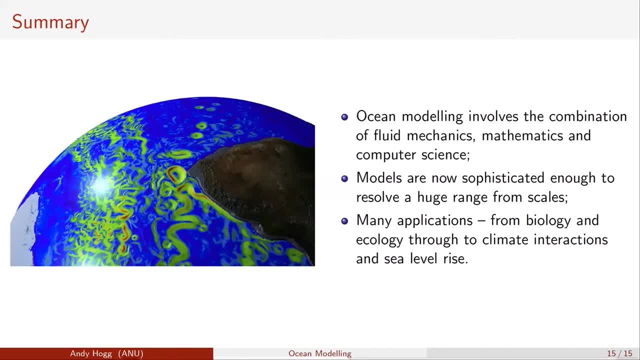 And yeah, I've got a question after you're done with this and the one that I'm happy for you to take, that And then, yeah, Okay, I'll, I'll answer this one then. Will warming oceans also contributed to more ocean calamities? 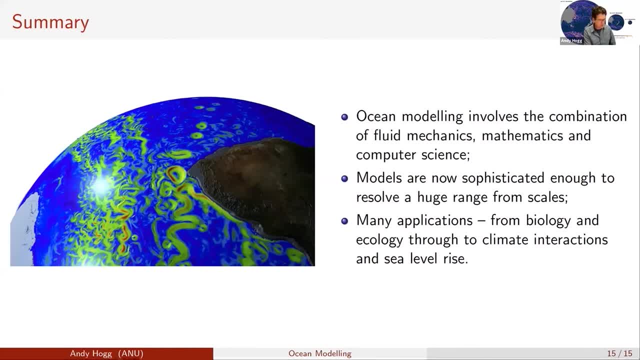 I'm not sure what sort of ocean calamities you're thinking about, but you know I mean sea level rise is is a calamity for some people. You know it will be economically expensive, but humanitarian, you know, societally in some point. 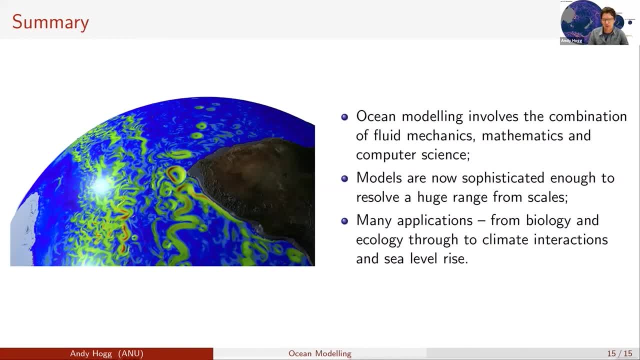 lying areas, it'll be catastrophic. The other catastrophic thing is a combination of ocean warming and acidification can really affect, for example, the formation of coral reefs. These coral reefs are critical for our biodiversity And I think it's you know almost certain that. 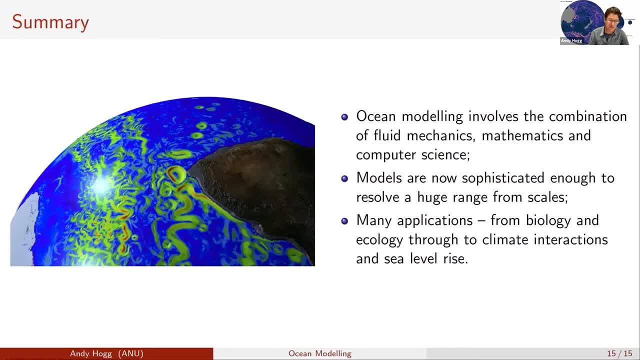 we will see more, for example, coral reef bleaching episodes, And I'm not a biologist but I you know I'm not that optimistic about the health of our reefs in the long term with the current ocean warming. Another calamity is sea ice in the Arctic region, which is very you know. 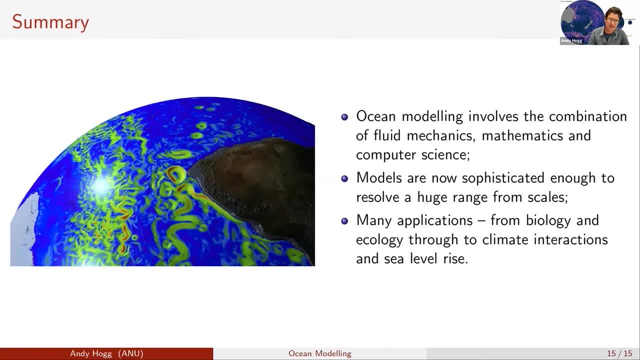 has taken a big hit And that as a consequence of disappearance of sea ice in the Arctic region, what we find is that the the the surface of the ocean is less white and more black. it absorbs more radiation and you get a positive feedback effect that the Arctic Ocean is warming faster than than you know. the Arctic is warming. 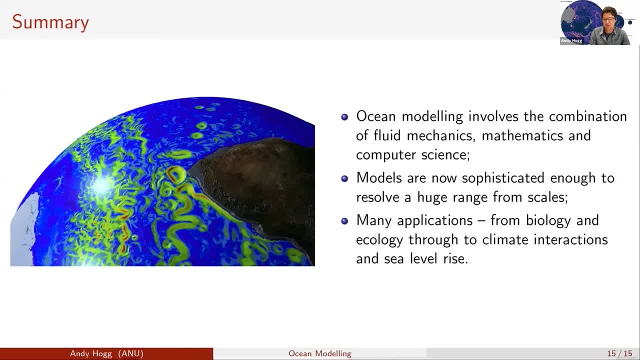 faster than any other part of the planet, And so that's, that's a big concern And it's you know, the ocean, sea ice system is key for that. So, short answer: yes, I've given you a few examples. 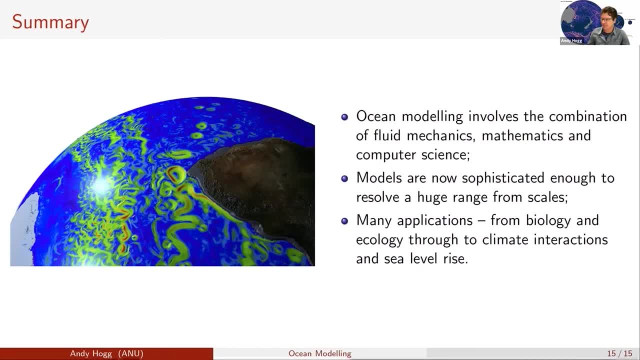 there are other examples around that that you can look up if you like, And then you're being streamed in a few lecture theaters around the world. So a question has come from one of those. hopefully you can answer it quickly. Is the ocean circulation slowing? If yes, why, And what could the impact be on climate change? 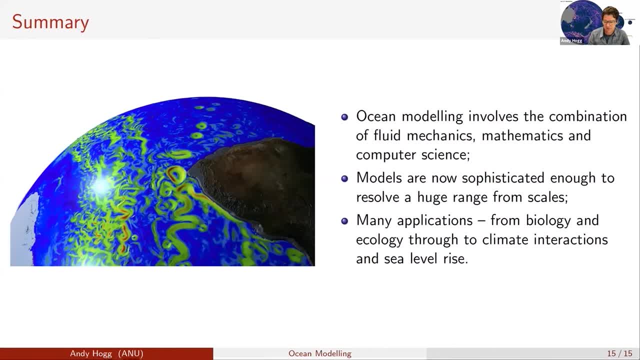 As a whole, I would say the ocean circulation is not slowing The. there are possible modes of ocean circulation, circulation which will slow down. So a lot of what I've shown you in plots like like this one on screen here what you're seeing is the signature of horizontal circulation and near surface currents. 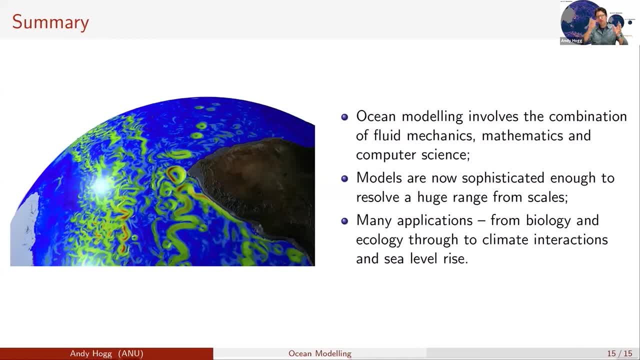 But one of the important currents is this overturning circulation, this deep circulation which takes dense water down to the bottom of the ocean, And there are theories that that deep limb of the overturning circulation could slow down, particularly in the North Atlantic region. 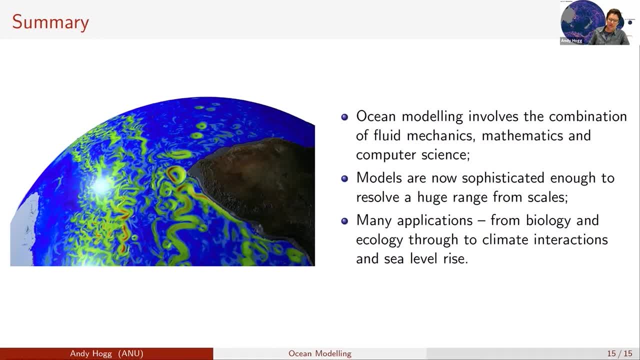 And the about 15 years ago, oceanographers set out to study that overturning circulation more carefully, And what they discovered is it's much more variable than they thought, but that variability does seem to have a slowing effect, And so that is one mode of circulation.